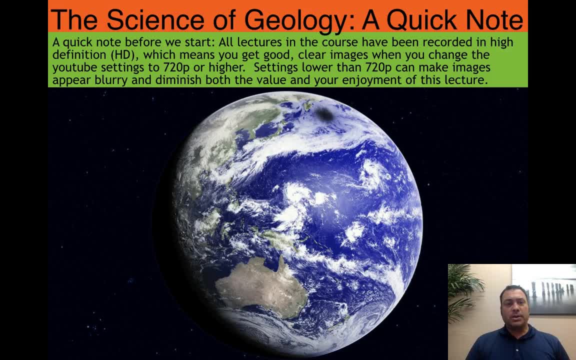 You might not even see them. So, anyways, at this point I just want you to go ahead and learn how to toggle between high definition and low definition on your YouTube channel. 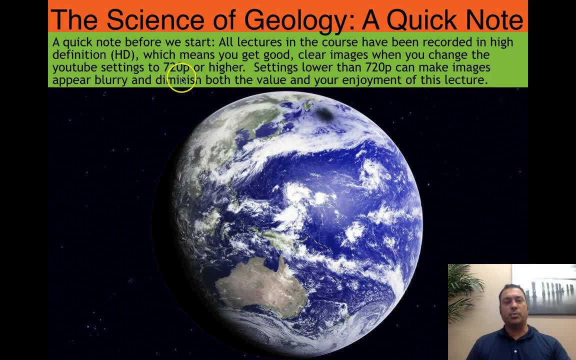 High definition means 720 points or higher. Lower than 720 is no longer considered high definition. Sometimes it's default set at about 360. So that's only about half the definition you can get. You want to get as much definition as possible. Now, if it slows down your computer so much that it doesn't load up 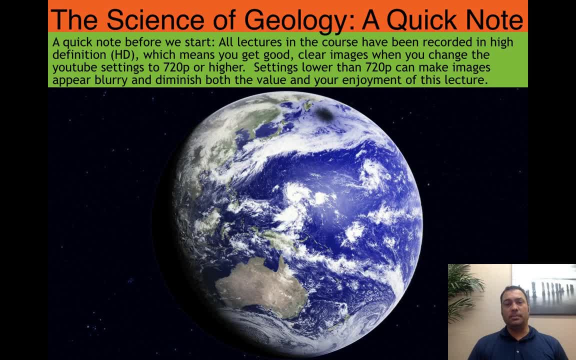 very rapidly, obviously you can reduce the resolution. But, anyways, I just wanted you to 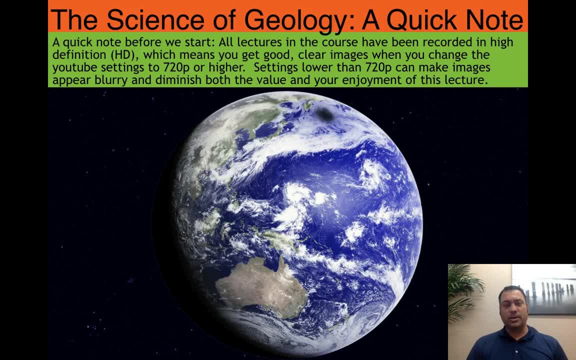 kind of know that that would be the best way to go. So, anyways, learn to toggle it. 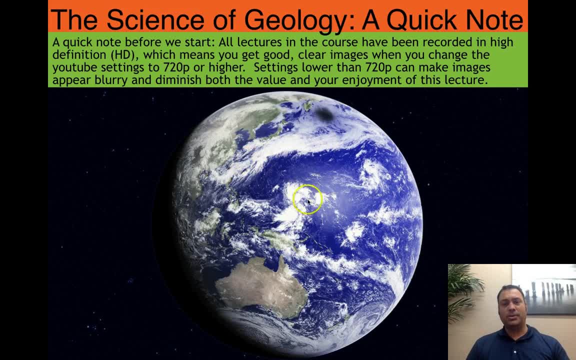 You can actually pause the video and watch maybe how the definition changes on this planet. But, anyways, pause the video and quickly toggle over to high definition. If necessary. 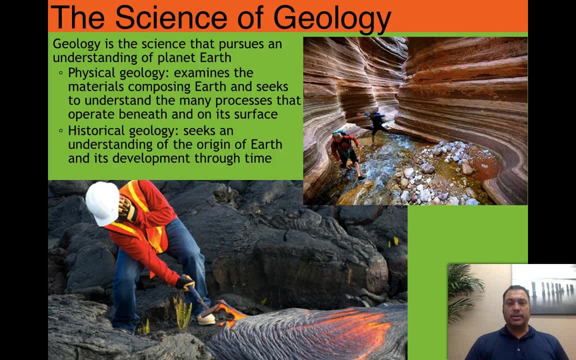 So, in our very first lecture, we're going to be introducing the science of geology. Geology is the science that pursues an understanding of planet Earth. We all have an intimate understanding of what the Earth is. The Earth is what we live in. Some people refer to it as Mother Earth. 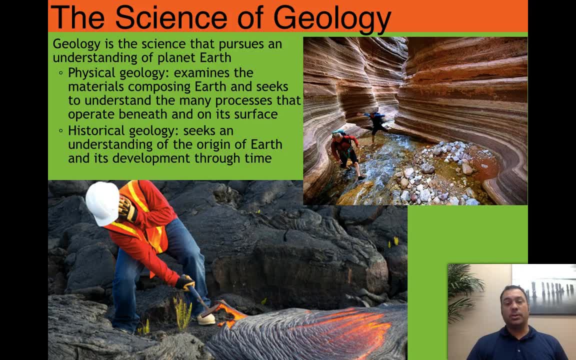 There are numerous religious deities. There are numerous approaches culturally to the Earth's history. So it's really close and important to us. 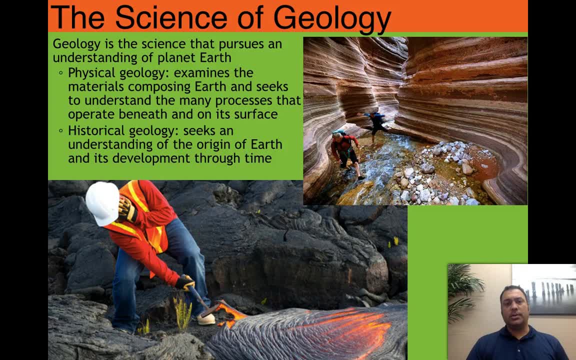 Now, the way that scientists look at the Earth is a little different, so we're going to introduce the science of geology, what we're actually doing. We're going to be taking ourselves away from the metaphysical approach of looking at our environments and actually start looking at it from a scientific viewpoint. And the way that we do this is usually by splitting geology into two sub-disciplines. There's 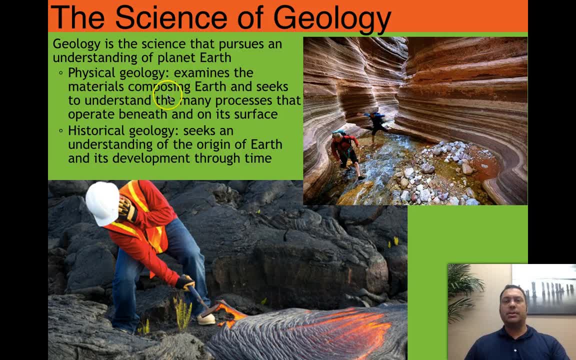 something called physical geology, and that examines the materials composing Earth and seeks to understand the many processes that operate beneath and on its surface. 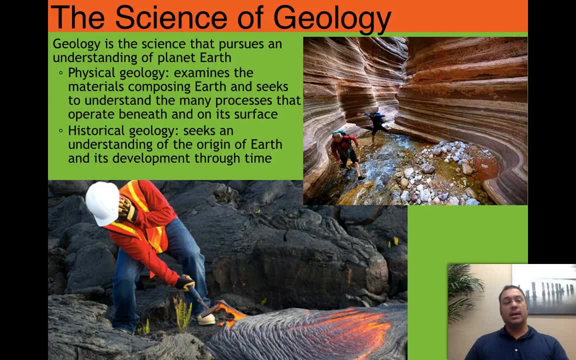 This is the main thing we'll be discussing in this class. 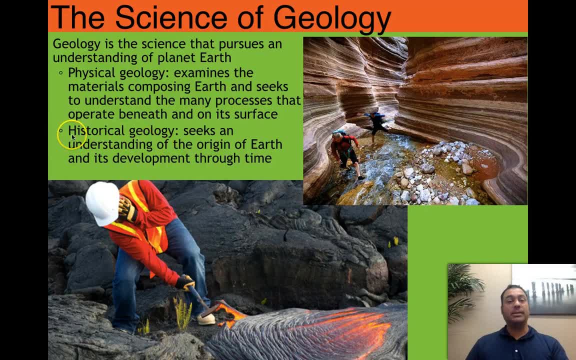 The second group is historical geology, or the second discipline is historical geology, and it seeks an understanding of the origin of Earth and its development through time. So, in other words, we would tell the story of Earth. That's usually taught as a different class than the one that we're teaching here. This will be predominantly physical geology. We will do some historical evidence. 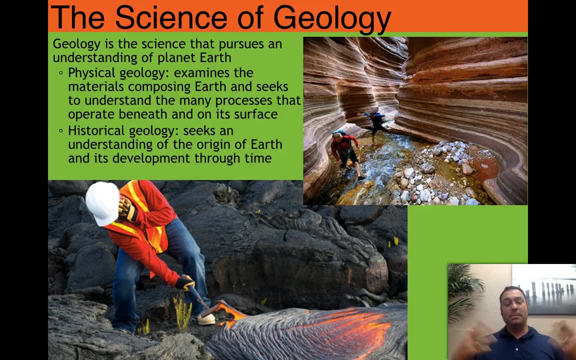 At the end, however, for those of you that are interested in that big picture question. 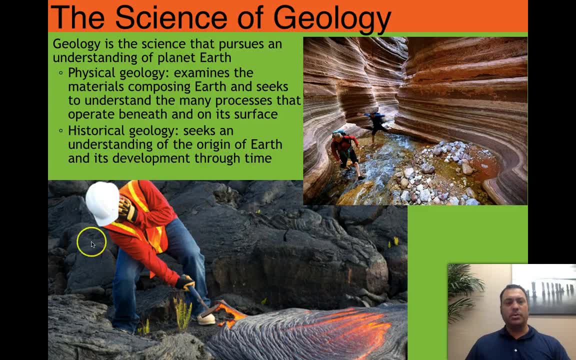 So what do we see here? Well, here we see, this is actually from the University of Hawaii website. This is one of their young, budding geology students that's taking a class in igneous rocks. And you can see that the student is coming down and having the experience of putting the rock hammer in the lava and covering their face because the heat is extremely hot. About three times hotter than your hottest oven setting 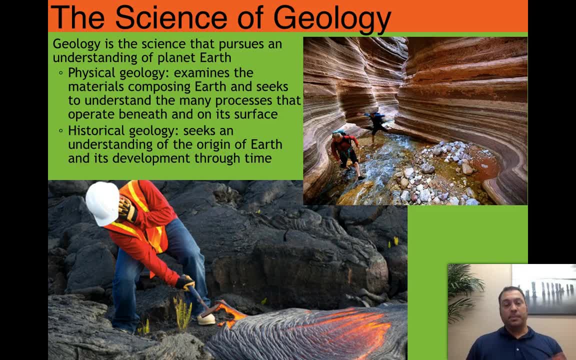 ever could be. And you can see how close the student is. 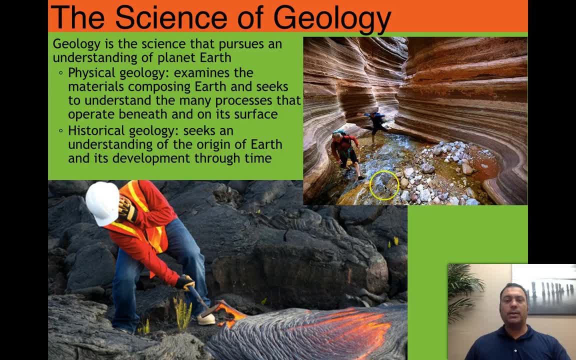 Up here, this is two hikers in the Grand Canyon. What I really like about these hikers coming through the Grand Canyon, this is a place called Hidden Canyon in the bottom of the Grand Canyon, is these sandstone layers right here. 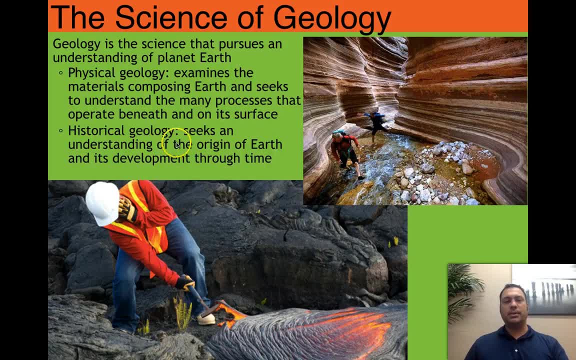 Each one of these layers is almost like a layer of history. This really fits into historical geology. But we'll be talking about where these layers come from right here. 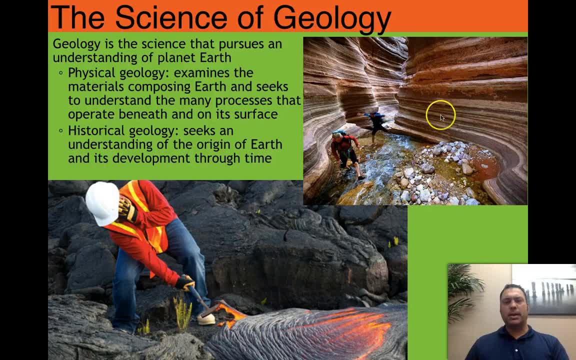 But not just that. What about these boulders down here? These boulders aren't made out of the same stuff as the walls. The boulders came from somewhere very distant. 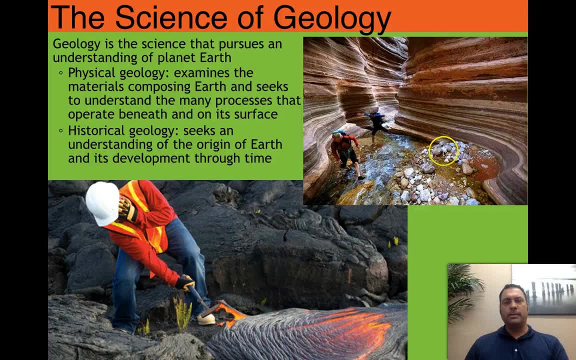 And it's a very different story for this than it is for these walls. In fact, 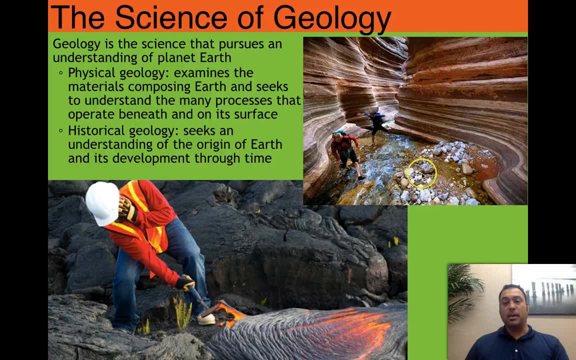 the rocks down here, even though the rocks themselves might be a billion years old and maybe the wall rocks are two hundred million years old, this deposit is being deposited today, but this one is quite ancient. So there's a lot of history going on, all just in a couple of picture slides right here. And these hikers are just kind of coming up right away. 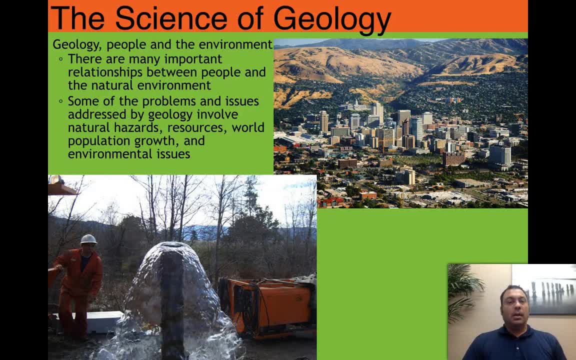 This is a little bit of a long sight. We also need to be aware that geology is really the science of people and the environment. So it's kind of the original environmental science. There are many important relationships between people and the natural environment. For example, here we see Salt Lake City, Utah. Salt Lake City, here's a matter of fact, the Capitol Building of Salt Lake City, right here. We might marvel at 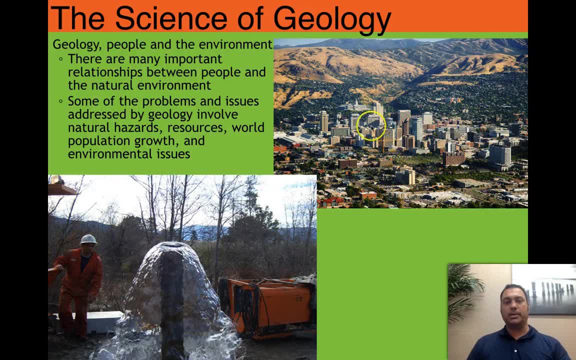 man's wonderful architecture. Here we see these tall buildings in downtown Salt Lake City. Some of them housing business enterprises that do billions of dollars worth of work every single year. But what do we see behind it? As tall and beautiful as these things are, we have these hills in the background and we have a canyon that comes right down here and we even see a little dam that's covering this section if you have sharp eyesight and you have it on high definition on your video. You can see these things. 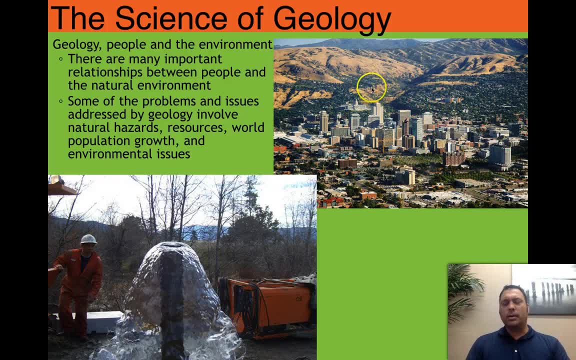 The question is what's more important or what's a more powerful force here? Well in the short term 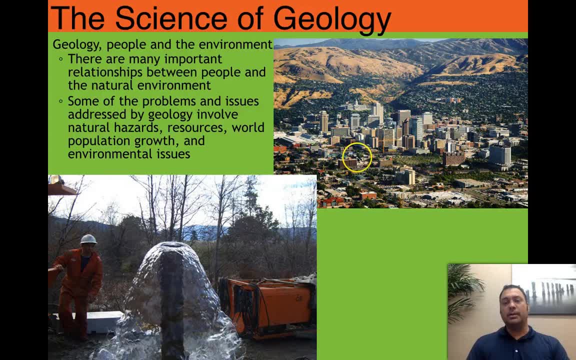 man has been able to convert all of the surface area into a city. But over the long term eventually what is causing these hills behind Salt Lake City to rise 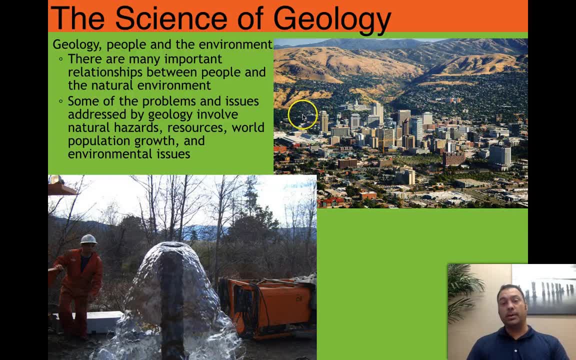 will continue to do so and usually that is accompanied by an earthquake. So it turns out that in Utah there are lots of earthquakes, there's something called an earthquake fault and those of you that might 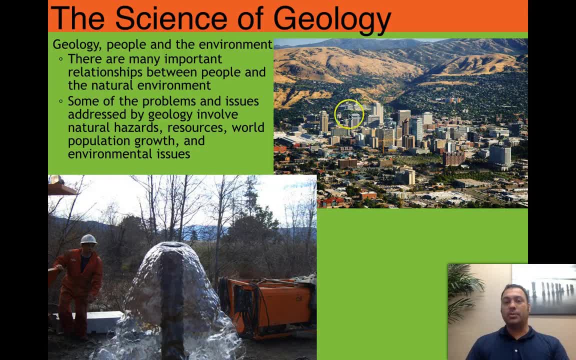 eventually develop a trained eye for these things turns out the fault is actually running right here behind these buildings and it's right in front of the 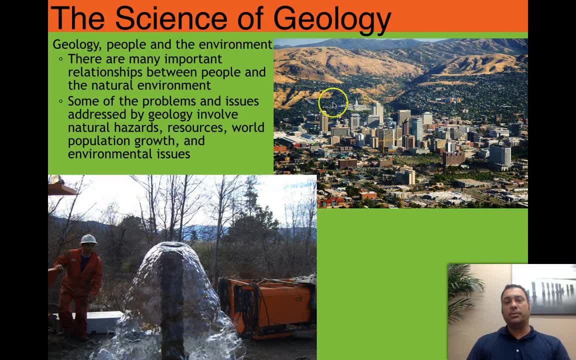 legislative offices located right here. In the event of a major flood we'd see a debris flow that would come right down and distribute all over inside the city which is why the built this dam here. 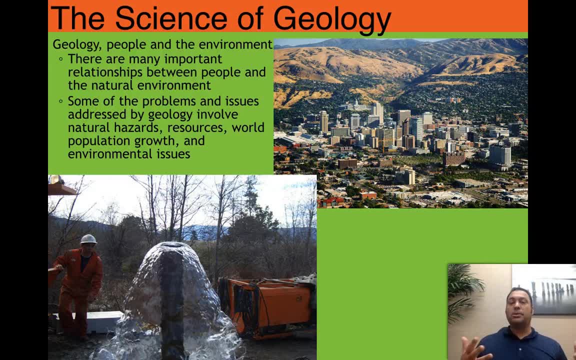 So eventually in the short term humans can actually do tremendous progress but in the end nature wins. It always will. 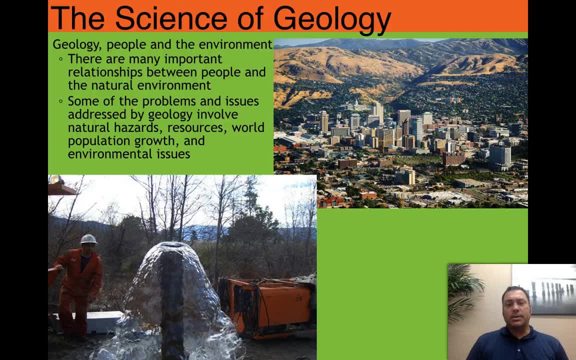 What causes earthquakes? What causes these mountains to rise in the first place? That is, of course, the subject of this class. 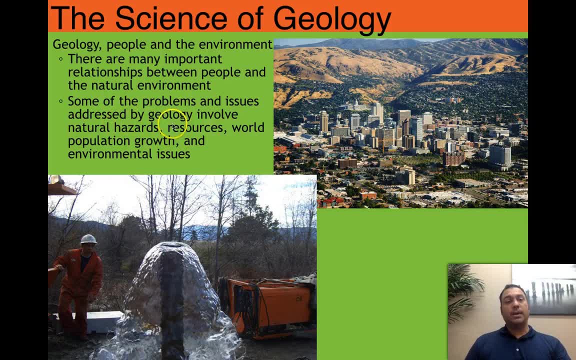 Some of the problems and issues addressed by geology involve natural hazards, resources, world population growth and environmental issues. Probably the most important thing that people argue over worldwide isn't necessarily land or clean air or access to food. 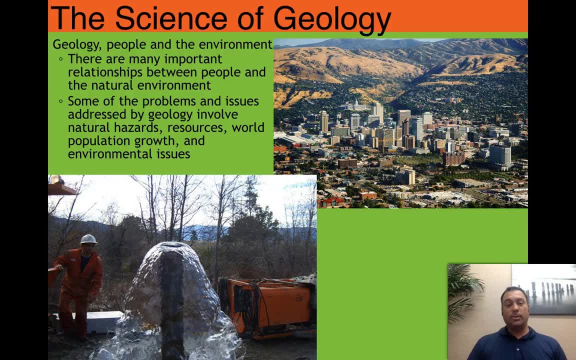 The number one point of conflict isn't even religion, even though religion is usually brought in as a justification for the conflict. The main thing that people fight over worldwide is water. 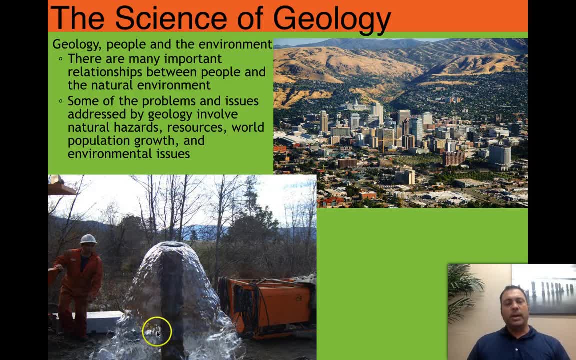 And here we can see this gentleman is looking at a water well that's been drilled. And the water is actually under natural pressure, so it's actually coming right out of the ground, out of this pipe. This is called an artesian well. And when you have artesian conditions, you wind up having water that comes right out, almost like oil. Out of the ground, if you can imagine an old oil well, spraying oil up into the air in the 1920s and 30s. This is what we see here as well. 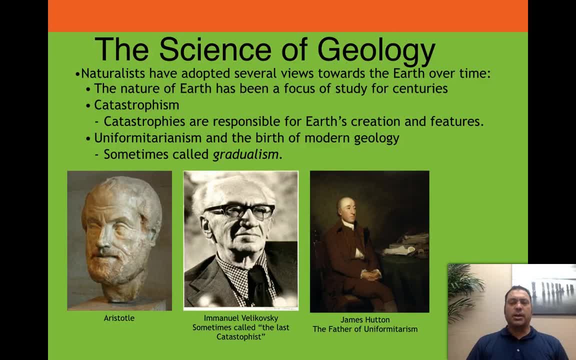 So the science of geology has come a long way. There was a lot of different ways that we looked at the world. 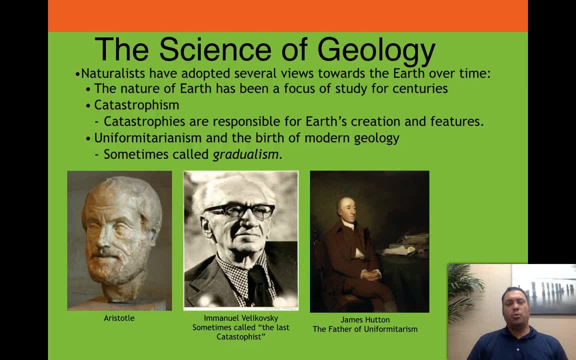 And basically, the first people to look at it were called naturalists. There were no real scientists. There was nobody to teach science in the traditional way that we do it now. Back in the days of ancient Greece, there was a series of famous writers, the most famous of which is a gentleman by the name of Aristotle. He was a philosopher, a naturalist. He spent a lot of time talking about origins of mountains and where fossils came from, in addition to the fact that he worked out formal logic. I mean, he actually looked at human thinking and worked out how logical systems operate. 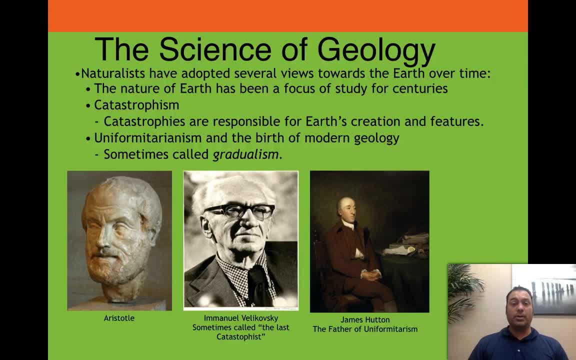 He was an absolutely brilliant person. He made a lot of critical mistakes, but at least he took a swing at some of these questions. And he approached them from a non-religious viewpoint, even though he himself had made some religious statements. And a lot of people generally believe that he was a believer in the Greek pantheon of gods and goddesses. 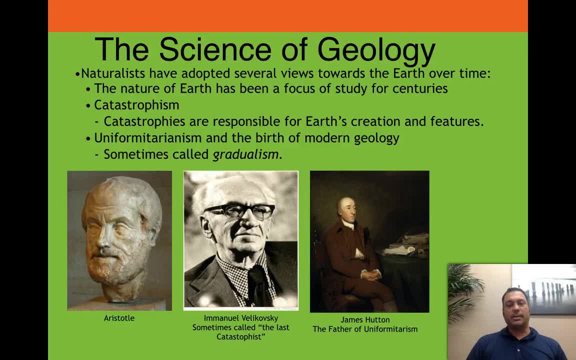 Ultimately, he was kind of the father of science, as we know it. And he spent a lot of time looking at earth science. The first way that people looked at things was through something called catastrophism. Catastrophism is basically where catastrophes are responsible for earth's creation and features. 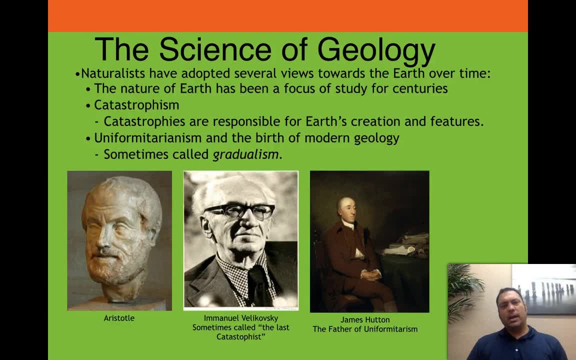 This is a way of thinking that dominated science and dominated our approach to almost all earth sciences until about 1900 or so. By about that time, we began to give up on that idea, because some other new philosophies had come online. Regarding science. And some discoveries had been made that actually demonstrated that it's probably not the best way to approach the problem. So catastrophism is the idea that, you know, major events such as a major flood created the Grand Canyon and also created all the river valleys all at the same time. Or major ice sheets came in and did it all kind of almost in a miraculous sense. And of course it was used, catastrophism was used by a lot of religious institutions as justification for a lot of their things. Theological beliefs. 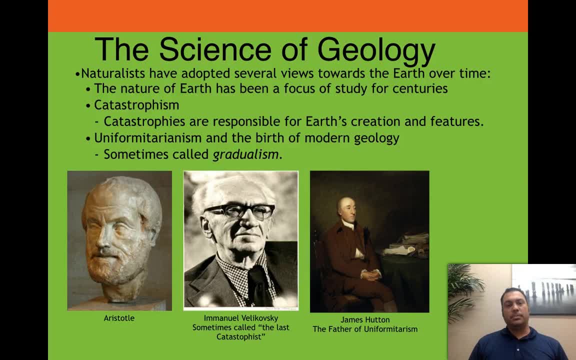 Uniformitarianism is a little bit different. Uniformitarianism is basically the philosophy that things are changing gradually over time. And it's sometimes referred to as gradualism. Uniformitarianism basically gave rise to the modern geological sciences as we know it. Right? So instead of looking necessarily at what a rock is, sometimes we spend more time looking at the processes that create the rock in the first place. The gradual evolution of systems. Okay? 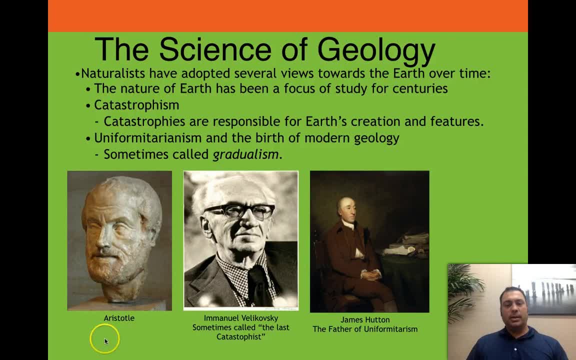 So here we see kind of the main players in this. Here we see Aristotle. Here's, I can't even say his last name. I think it's Velikovsky. But he was the last catastrophist. There are none of these left. I think he passed away in the 1950s or 60s, right around in there. He was the last one. Still a very good scientist. I'm not saying that he wasn't. 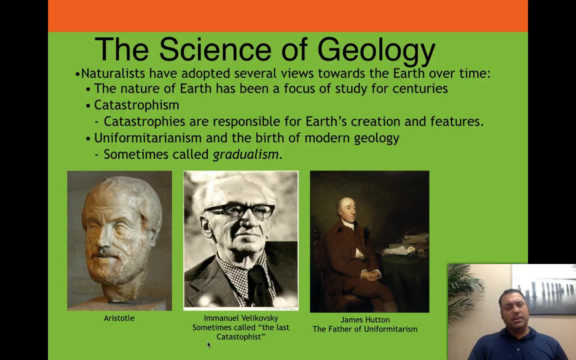 Had some really good observations. But his interpretations were largely incorrect. And of course we now know, in the light of things called plate tectonics, that his ideas certainly don't hold up. 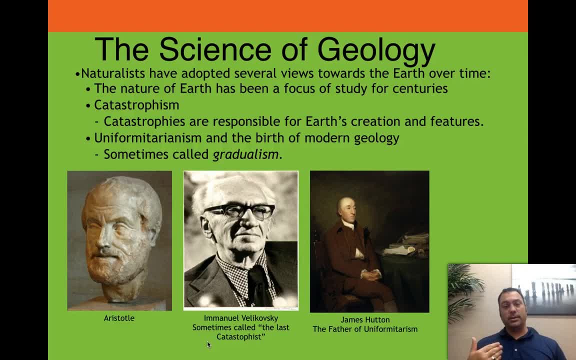 But his observations are still useful to us in some respects. Of course the guy that got it all started was a gentleman by the name of James Hutton. And he is an English scientist. 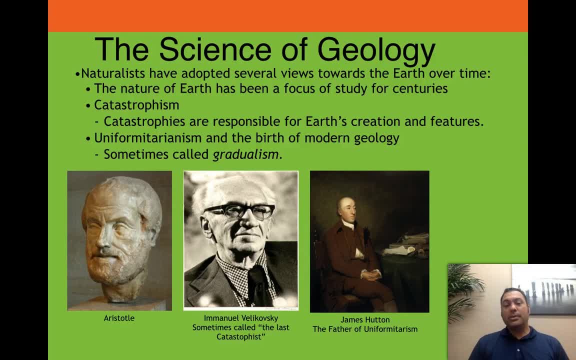 He was not the most popular person amongst his peers. He was considered a very abrasive and difficult person to get along with. And as a consequence, even though he had the idea and actually wrote a lot of the stuff down about uniformitarianism, people didn't want to deal with him. 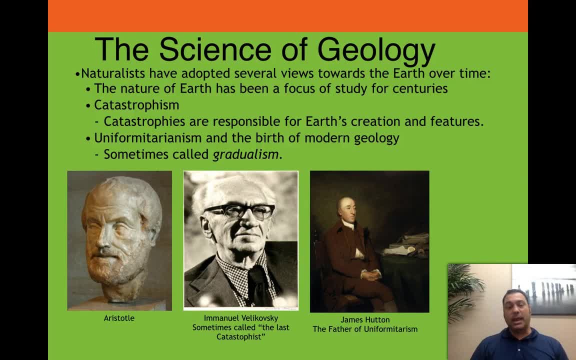 And so his ideas were slow to take hold. It wasn't really until a guy by the name of Charles Lyell, who was a good friend of Charles Darwin, actually, before the field of geology really got its first textbook 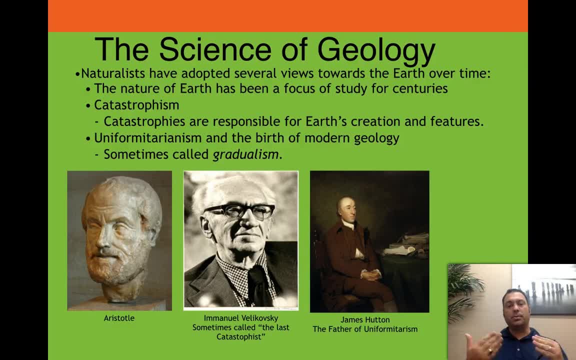 and we started actually seeing cohorts of students that were studying it in a formal way. Okay. 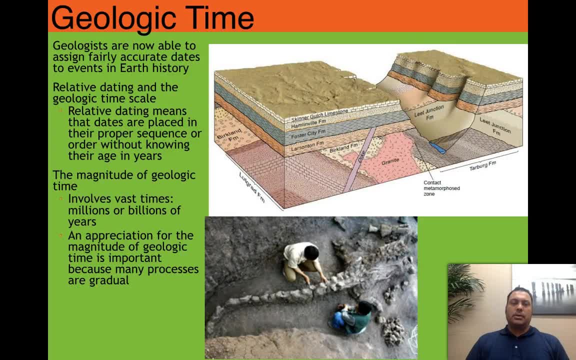 Another idea that we need to kind of introduce early, because it's one of those things that we're not accustomed to as human beings, thinking about, which is geologic time. You know, when we go from place to place, we're used to thinking in terms of minutes. If we're thinking about human lifespans, we're thinking in terms of decades maybe. And in some tragic cases, only years. But we're not certainly, and even in historical terms, we're thinking about, we might think about millennia. 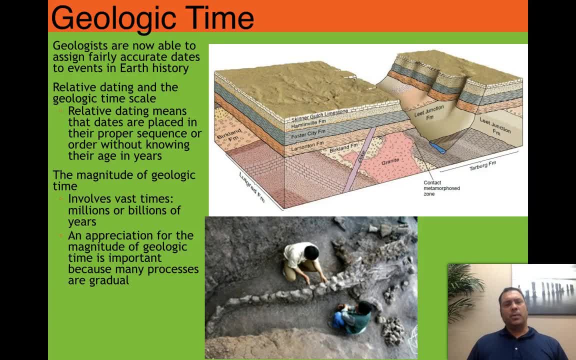 But we don't necessarily think in geologic time scales, right? We don't think about what a million years means or what a billion years means. A billion years is so much time, you can't fathom it. It's something you can't even imagine. A thousand years ago, human beings were populating medieval Europe. They were getting ready to build ships that would go across the Atlantic Ocean. Polynesians had settled all over the South Pacific and had conquered even as far as Madagascar. Genghis Khan's armies were almost about to go and basically unify all of Asia. That was a thousand years ago. That seems like ancient history to us. 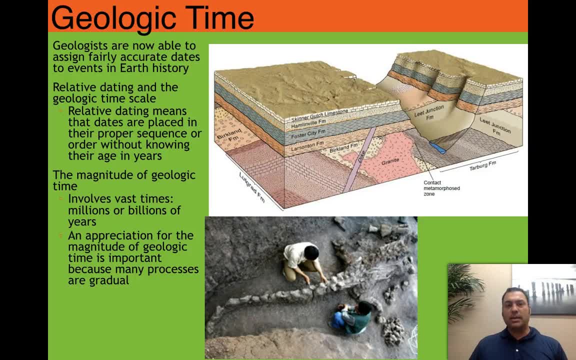 But a thousand years ago, what did the landscape look like? Exactly the same as it does now, almost exactly. But what about a million years ago? 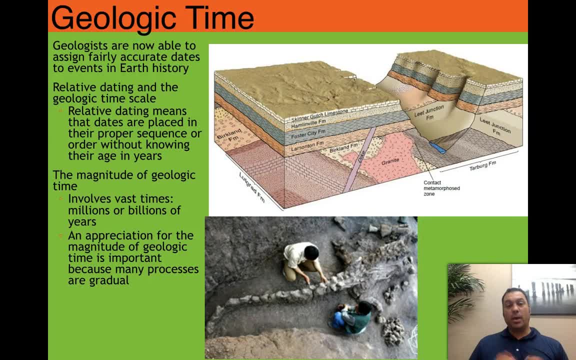 If we think about it, a million years ago, the island of Hawaii, the big island of Hawaii, didn't exist. 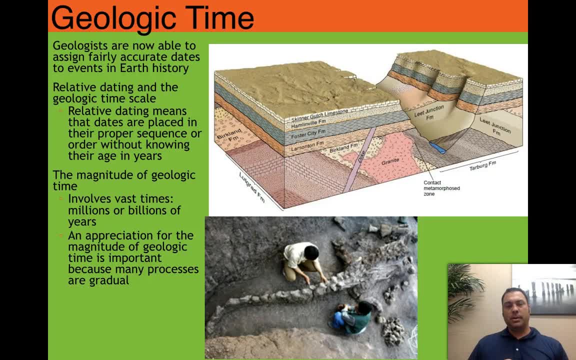 If we think about what happened a million years ago, the city where we now know as Los Angeles was a shallow inland bay. 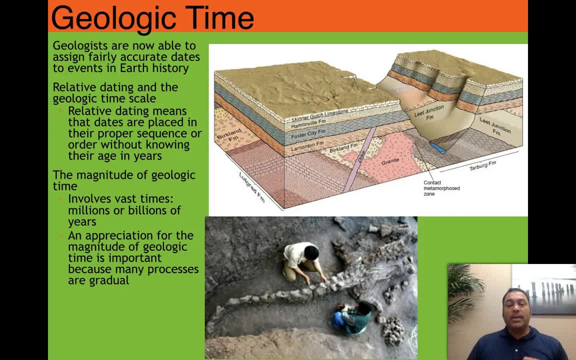 If we think about things a million years ago, we find that a lot of things have changed. 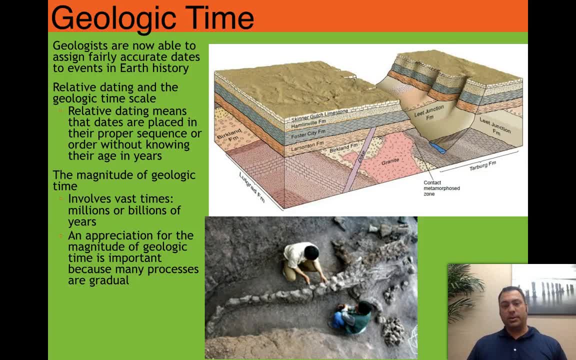 And if we go even further, 50 million years ago or 100 million years ago, a lot changes. When we look at rocks, we know that they're 100 million years old. 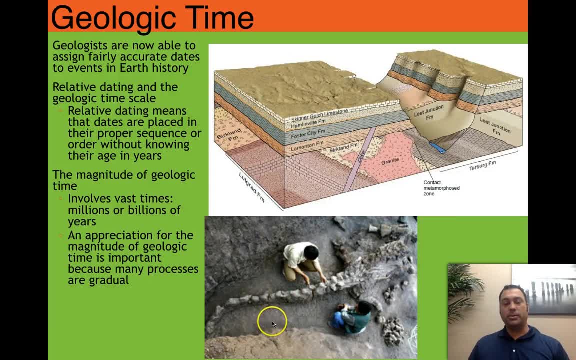 And we'll discover why during the class, why we know that they're 100 million years old. 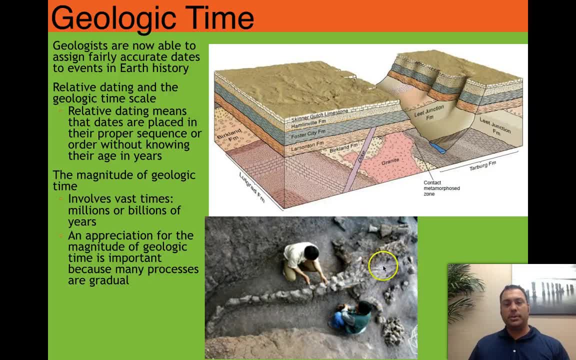 We find that the animals themselves, this is a fossil, this is a dinosaur in here, have changed considerably. 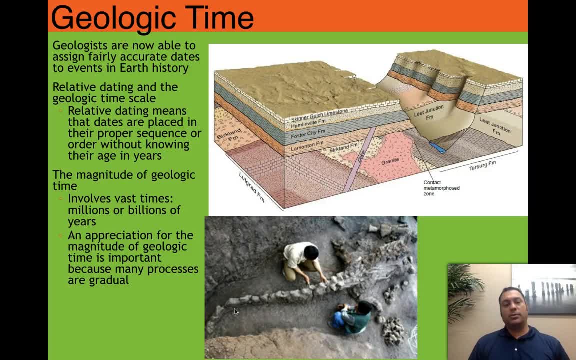 So we need to develop what we call an appreciation for the magnitude of geologic times. 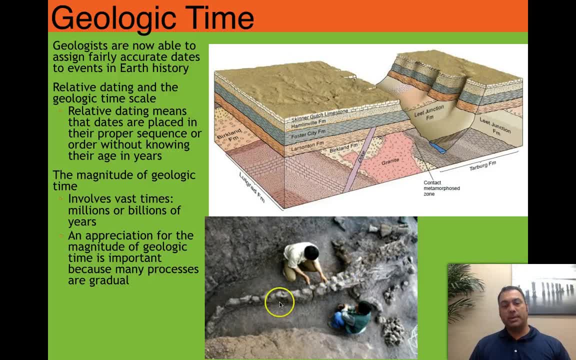 This process of this animal, it might have gone extinct. As a matter of fact, its species all went extinct very quickly, 25 million years ago. 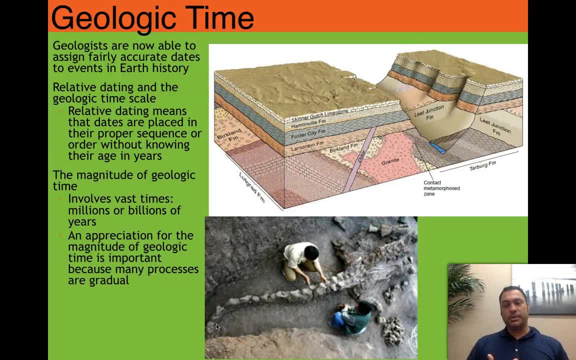 But its evolution occurred over several hundred million years. And we are now discovering through DNA analysis that we are very closely related to a lot of what we even see in the dinosaurs. So it means that there's some common ancestry amongst us. 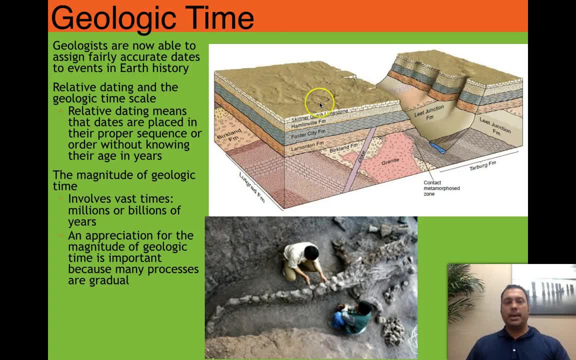 Other things that we would see is we could look at maybe a landscape now, and we can make some assessments about how old things are. 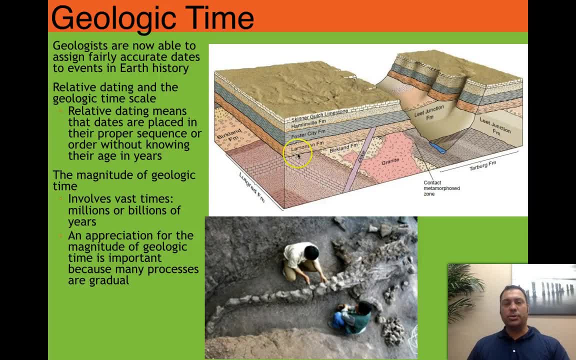 Well, obviously, the things at the bottom, for example, this orange layer is going to be much, much older than this upper layer, this limestone, the Skinner Gulch is what it says here. 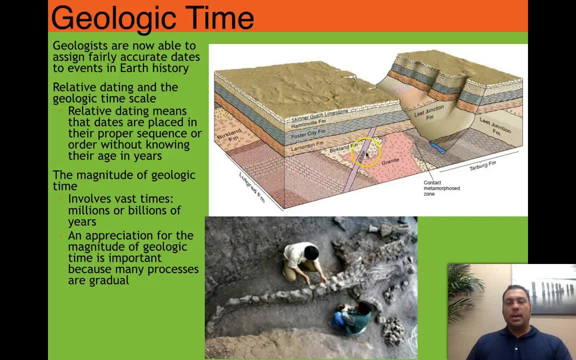 So what's at the bottom is going to be older than what's on top. And there's another rule, right? 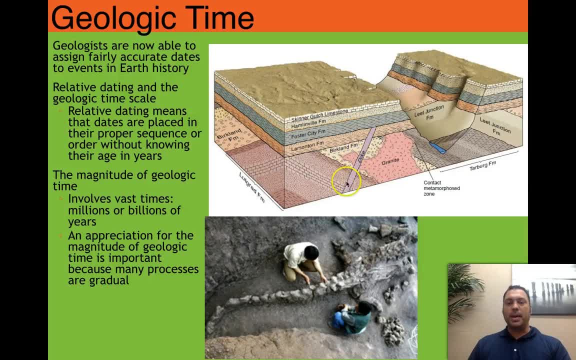 Here we see a dike. A dike is a body of magma that was injected into the rock through tectonic processes or volcanic processes. 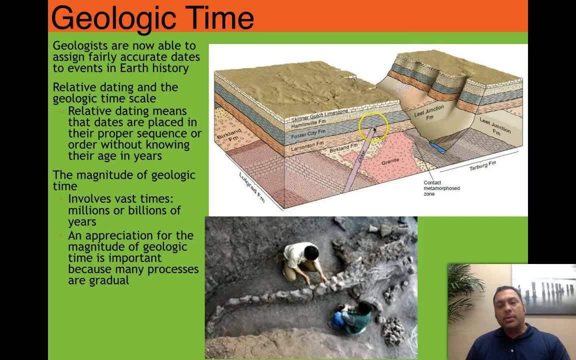 And when we look at a dike, we notice the dike only comes up to the blue one that's cut off. 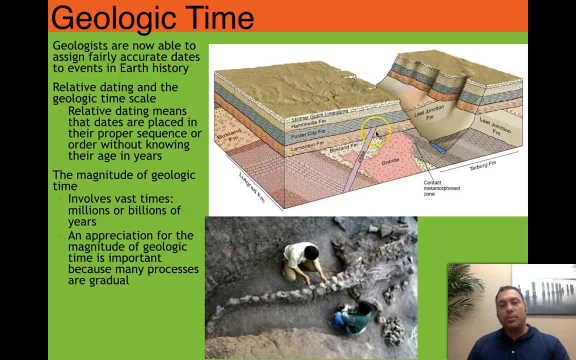 So when we look at a rock, we know that this orange had to be here, or the dike wouldn't be able to go in it, right? 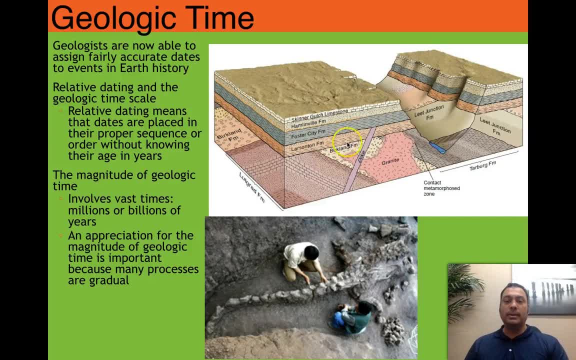 There's an old axiom that we need to keep in mind. You got to make it before you break it. 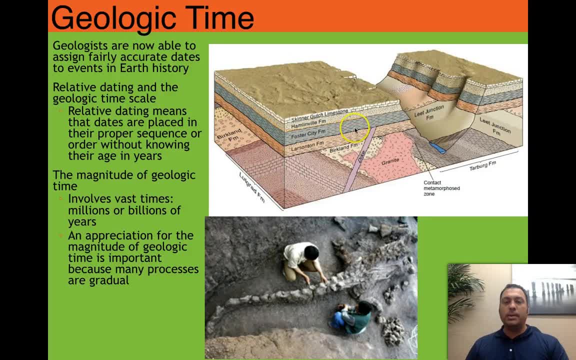 So the dike is older than the orange, but younger than this gray or this blue, depending on whether you're colorblind or not. It could be gray to you. 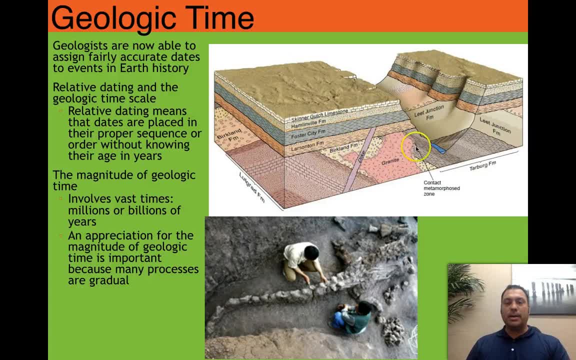 All right? And then, of course, beneath all of that, we see these rock layers, and they're all tilted. 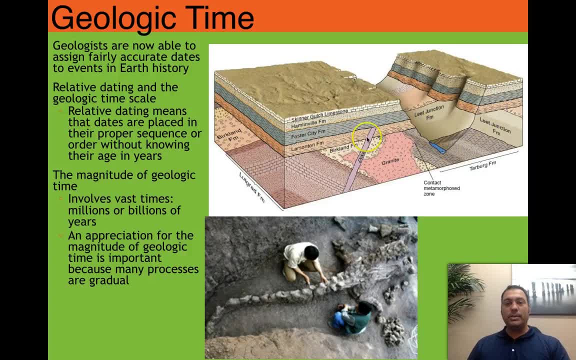 So the rock layers had to be made again and then tilted before these other layers could come on. 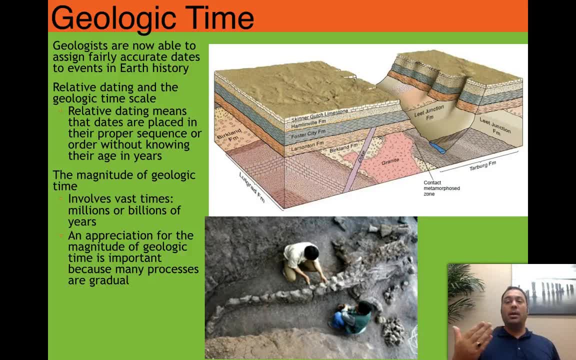 And so you can see that we aren't able to put together a story. What's the most recent part of that story? 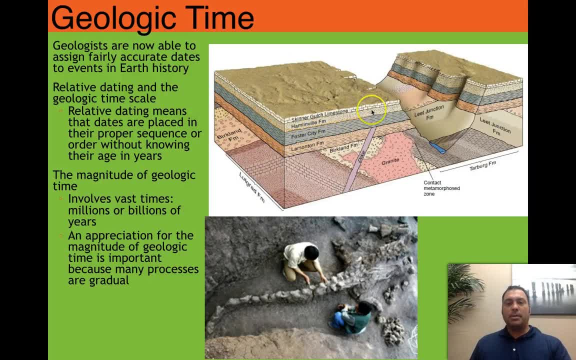 Well, the limestone is obviously not the top part because it comes up here and it ends, and then it's found back over here again. 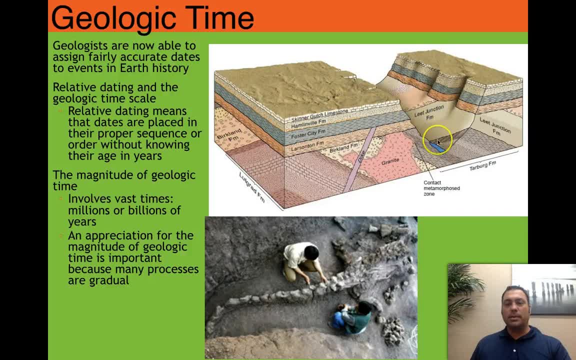 So we have a gully that's actually formed in the meantime, and now there's a river. 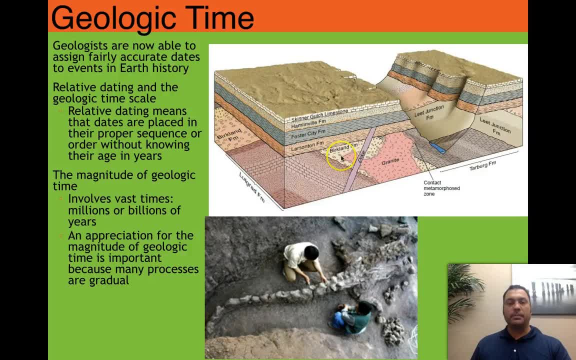 So the most recent story is this river cutting through here. And so the way that kind of the whole purpose of this little slide is by looking at this, we're able to figure out relative dating. In other words, how things happened in sequence. It's almost, you don't actually get a number, but you might actually get a, this had to happen before this, before this had to happen before this, and so on. 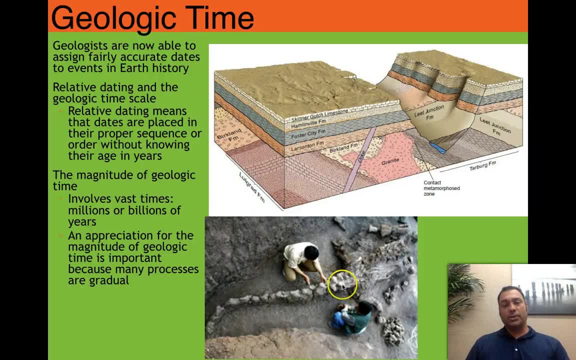 But we can sometimes put numbers to it. We actually know about how old a lot of the dinosaurs are. And if we find the fossils in the rocks, we know about how old they are. And so we can put a number to it. You get the idea. 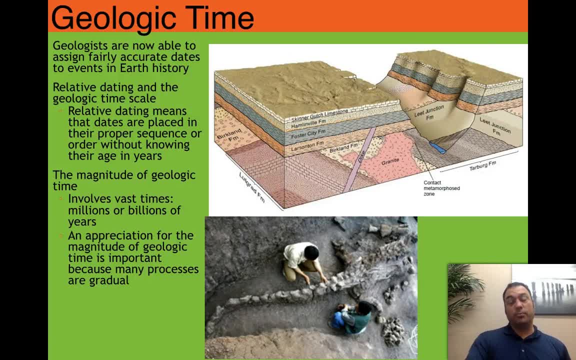 And so these are concepts we'll be bringing up throughout the rest of the semester. 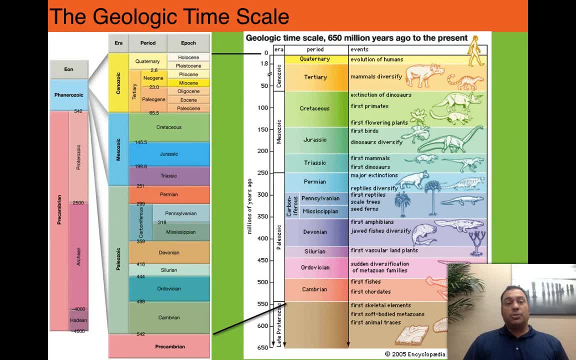 The geologic time scale, of course, has shown us that there's tremendous diversity of Earth history, what's gone on. 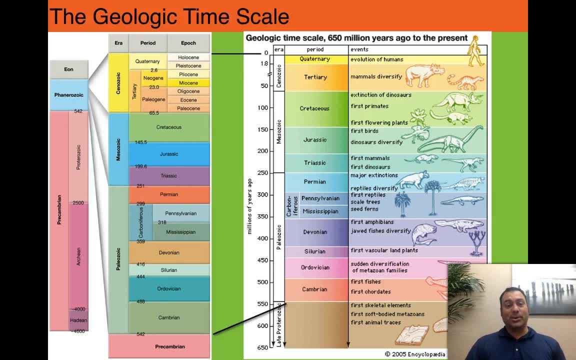 Now, when I say tremendous, most of that tremendous diversity has occurred, especially in the life sciences, really only in the last half billion years, about 550 million years ago. Prior to that, there was really a lot of boring stuff going on. The largest part of Earth history is something called the Precambrian, which is, if we look at this here, so if this is a bar and this is all of Earth history, this is from the origins of the Earth, which we will discover to be 4.5, or actually in here, 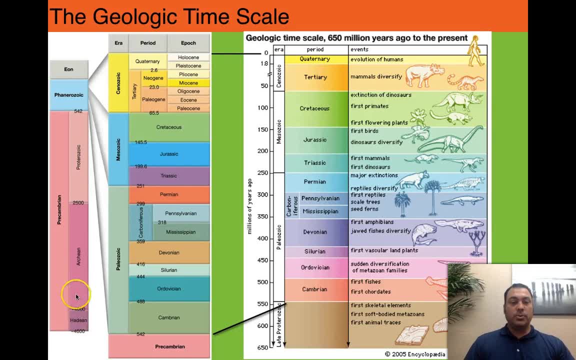 it's going to be 4.6 billion years old, to 542 million years ago. That's 90% of Earth history. 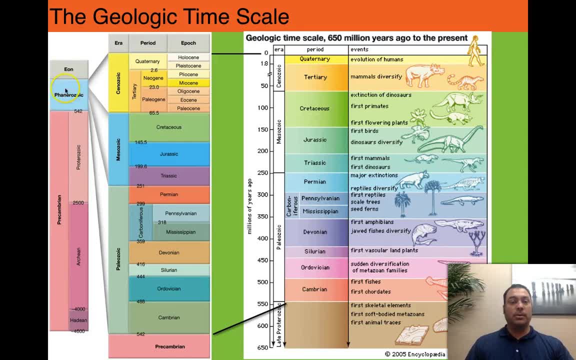 There's something called the Precambrian. This blue part over here is the part that we live in, something called the Phanerozoic. 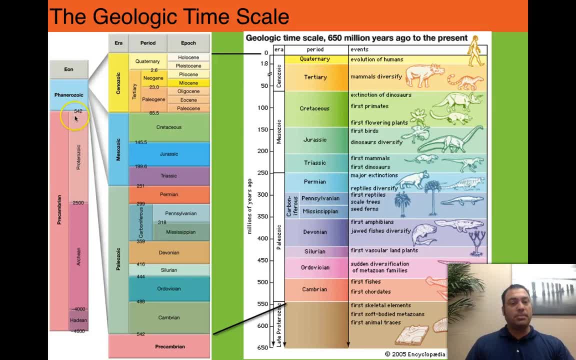 So what do these things mean here? Well, the Precambrian means just before the Cambrian. Well, why would they call it that? 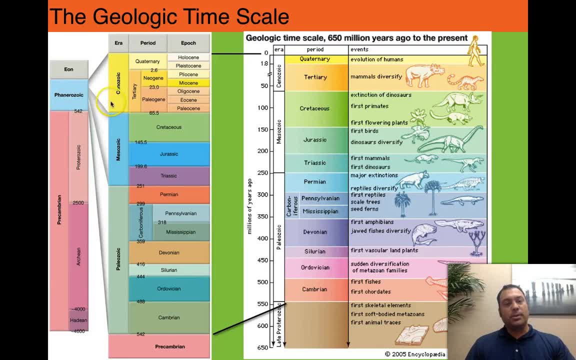 Well, if we look at the Phanerozoic, the Phanerozoic is broken up into three groups, the Cenozoic, the Mesozoic, and the Phanerozoic. 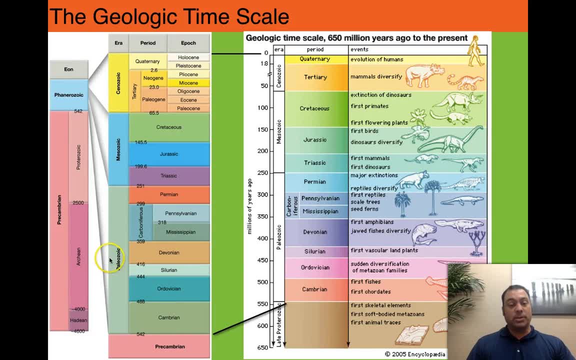 And the earliest part of the Phanerozoic, which is, say, the most ancient part, is the Cambrian. 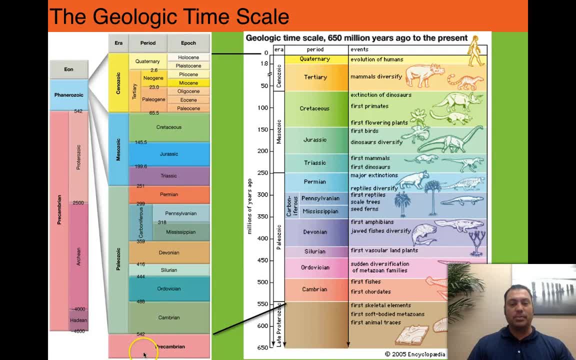 So the Precambrian is just everything before the Cambrian, which is why you see Cambrian and then Precambrian here. Okay. 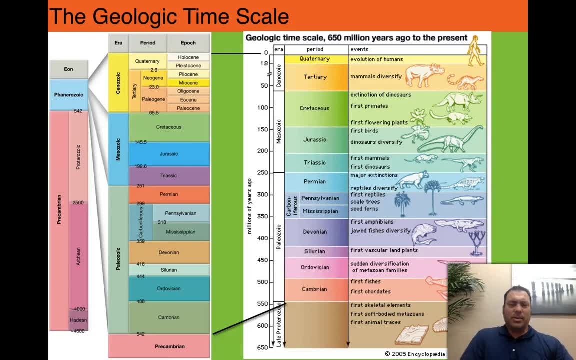 So you might be saying, well, what does that mean? Well, 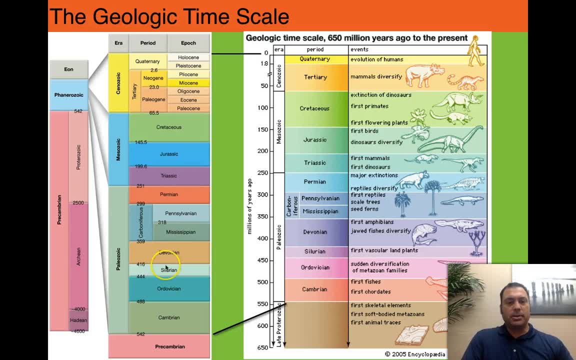 and by the way, these are a lot of fancy sounding words, right? Well, the Paleozoic means ancient life. 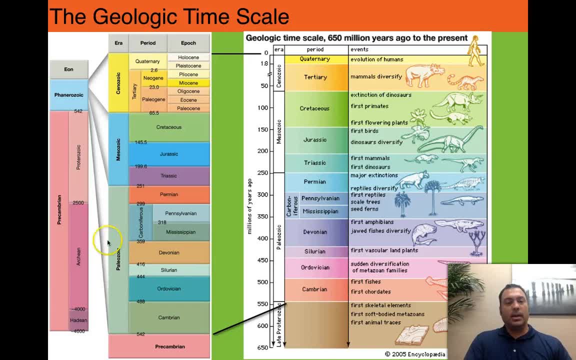 Paleozoic. Zoa meaning life. 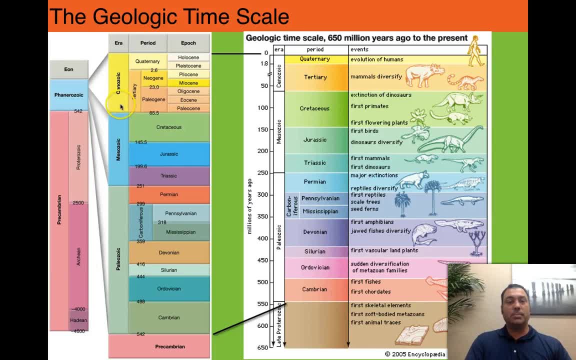 Mesozoic meaning middle life. And Cenozoic meaning recent life. 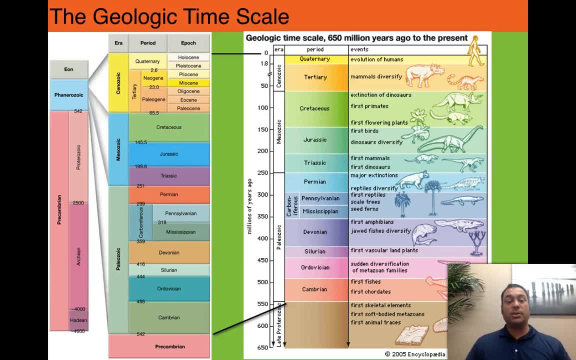 So the Paleozoic, the time of ancient life, is when we actually start seeing fossils in the rocks with hard shells and teeth and vertebrae and fish. 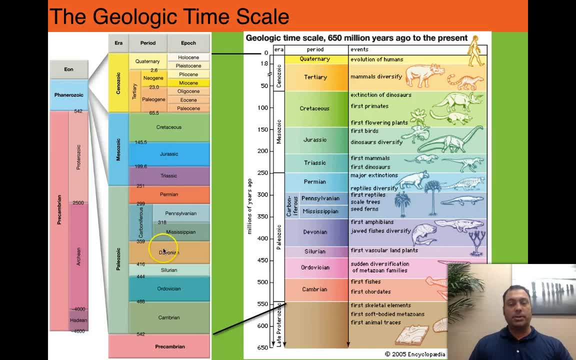 And by the time we get to the Devonian, we're actually seeing large sharks. 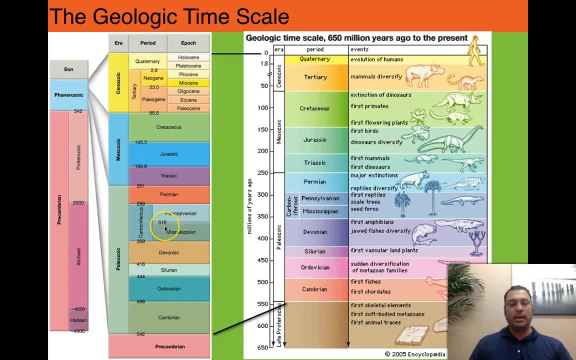 And the Mississippian, huge fern forests living up on the land. 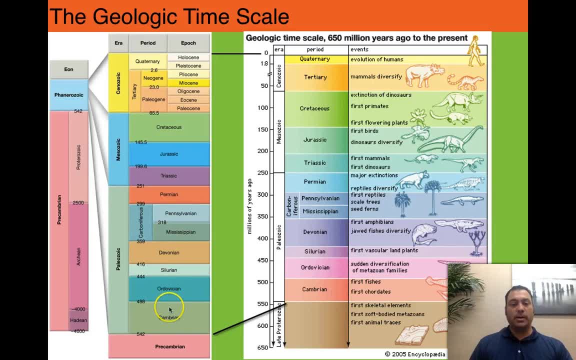 But during the Cambrian, everything was just in the ocean, right? 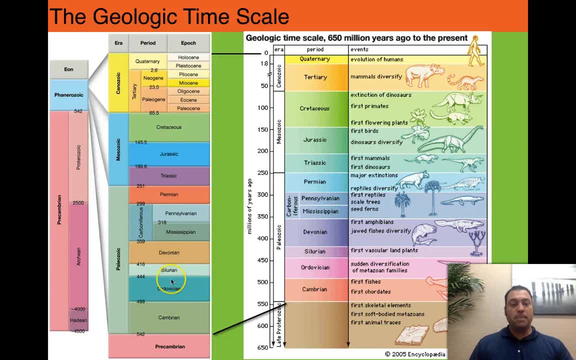 So between the Cambrian and the Devonian, there's tremendous changes in life that's happening here over this hundred million year period. 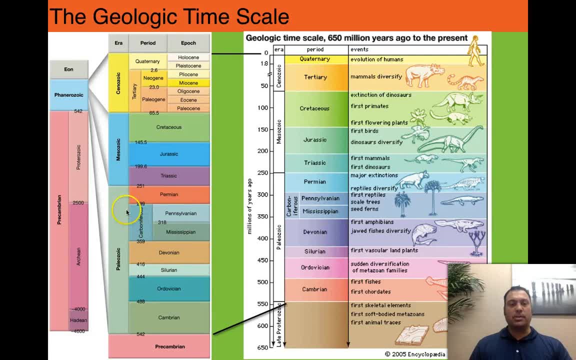 When we get into the Mississippian and the Pennsylvanian, which the Europeans call the Carboniferous, don't worry about it. And you won't have to memorize the timescale. Don't worry about it. I'm just guiding you through it. 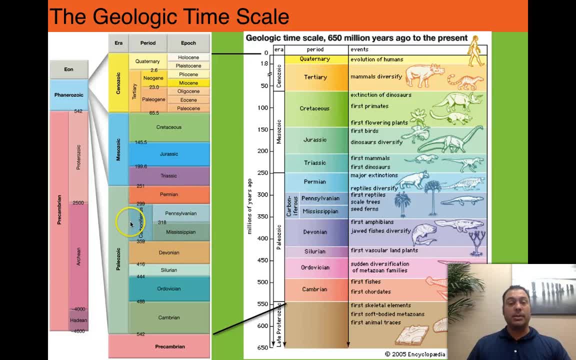 We start seeing an explosion in the size of land animals, as well as insects. During the Carboniferous, we find, not mosquitoes, dragonflies with wings that are several feet across in the fossil record. 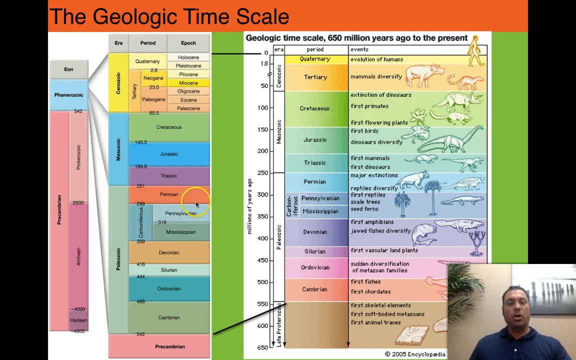 And by the time we get to the Permian, we actually see animals that look almost dinosaur-like. They're very large. They have very sharp teeth. 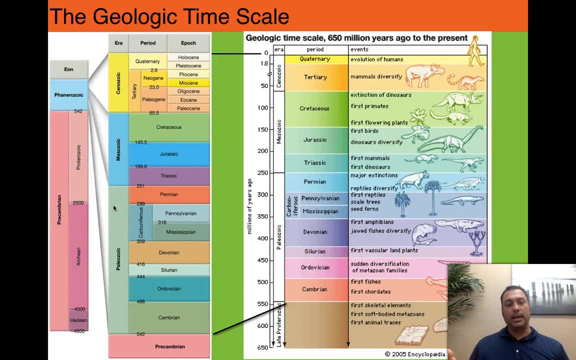 There's carnivores living both in the oceans and up on the land. But between the Permian and the Triassic, 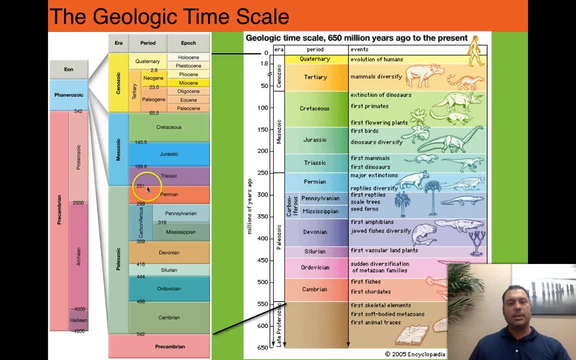 at 251 million years ago, there was a massive extinction. And almost all of the things that lived during this period of time went extinct. 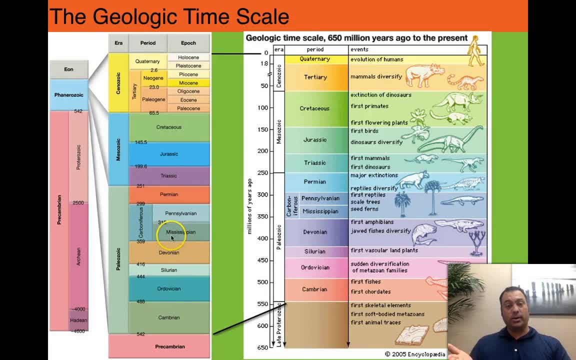 Now, a few things did survive, of course, because we, you know, were here. But our ancestors were hit at one point very strongly by an extinction. And we find that fish survived, and sharks survived, ferns, things like this that we see today. But a lot of the other species died off. 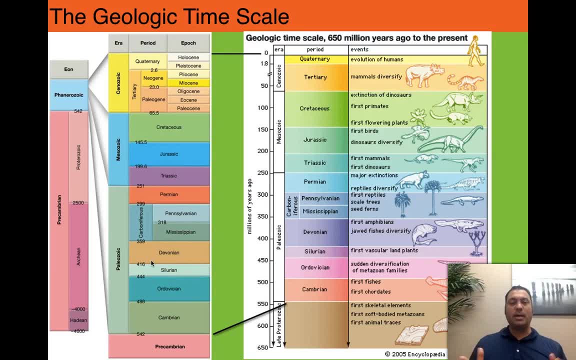 Things like trilobites, which are an early type of lobster creature that looks like a giant pill bug that dominated the oceans. 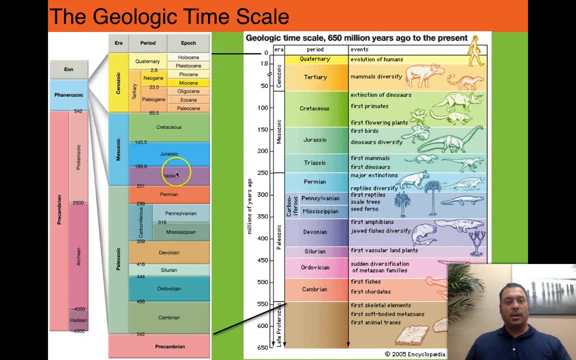 We're extinct by the Permian. And then we go into the Triassic, the Jurassic, and the Cretaceous. 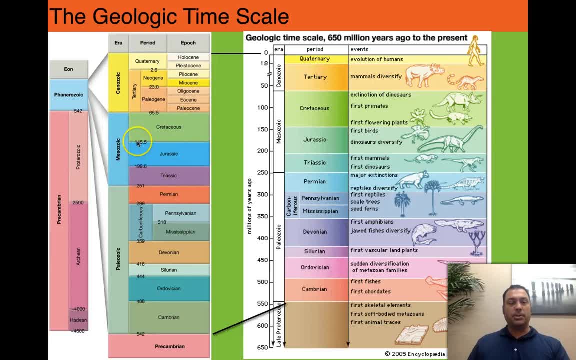 This is the three subgroups of a group called the Mesozoic, or middle, the middle life. 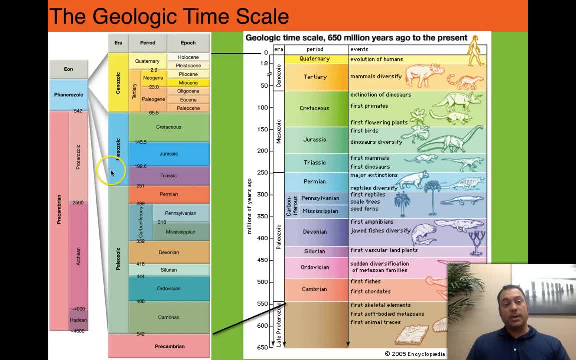 It's also commonly referred to as the age of the dinosaurs. So from the Permian into the Mesozoic is the time of the dinosaurs. 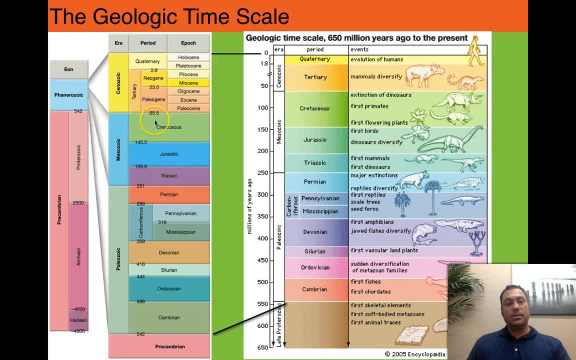 And they went extinct at 65 and a half million years ago. 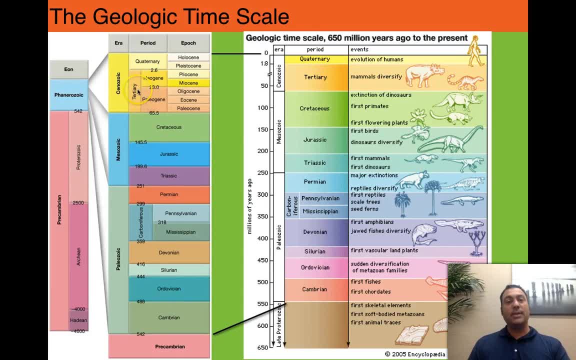 And that dumps us into the Cenozoic, which is the age of, of mammals. 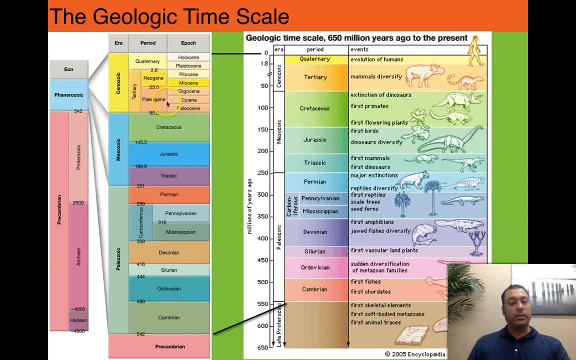 And so the early mammals grew very, very large. 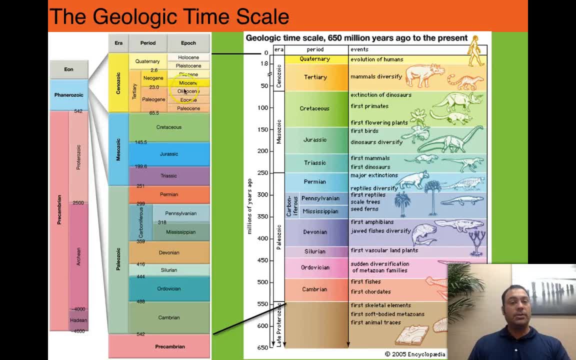 We evolved whales and elephants. But all of that evolved just right here. Right? And they're still evolving today. 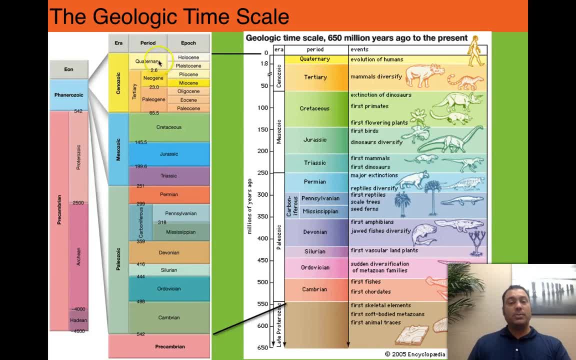 The most recent period of time is the Quaternary and the Holocene. And that's where human beings live. The Pleistocene is when you think of cavemen, right? Neanderthals and things like this. This is all in the Quaternary. Okay? 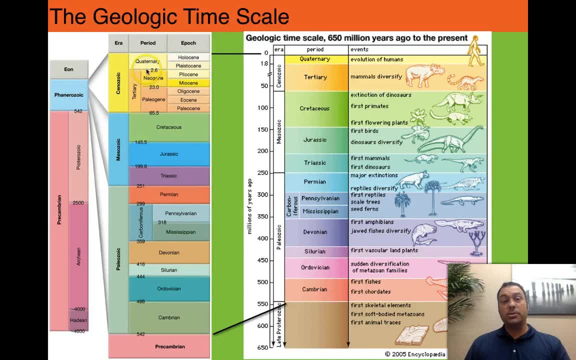 But if we look at the time period, that's only the last two million years or so. The Earth is 4.6 billion years old. 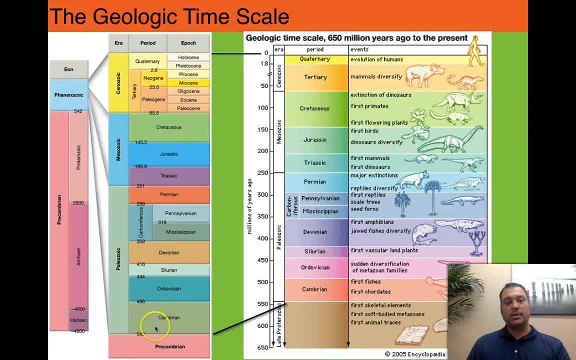 So we got a telescope into this, to this, and then this, to this, telescopes into, again, this time scale. But this tells us the different life forms that we would expect. 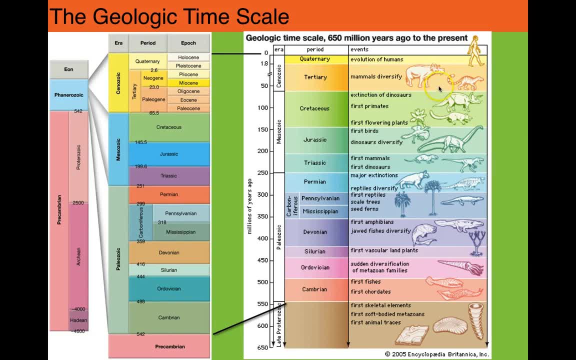 And here you can see the changes in body forms that we see in our rock record. All the way up to human beings way up here. 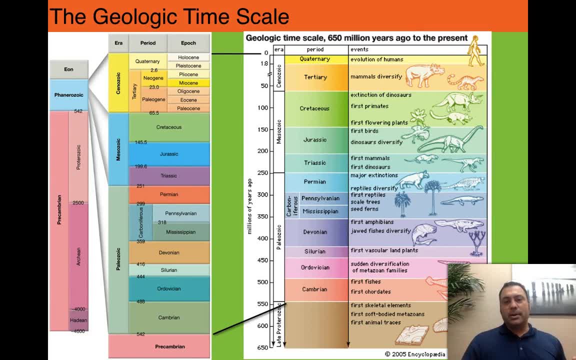 Hopefully you didn't get buried in the time scale, but it's interesting stuff. 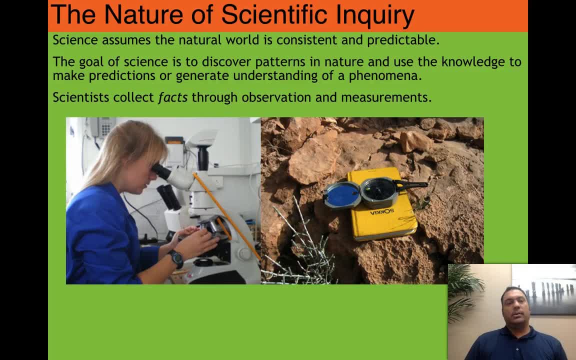 So the nature of scientific inquiry is, it's one of those things that kind of cuts across all boundaries. 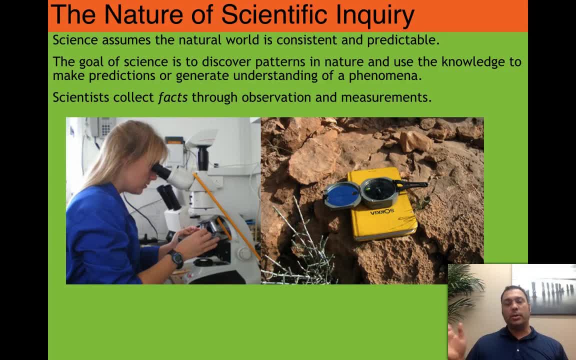 It's science that's not just done in the United States or in Europe, or even by the Chinese. It's done by Mongolians. 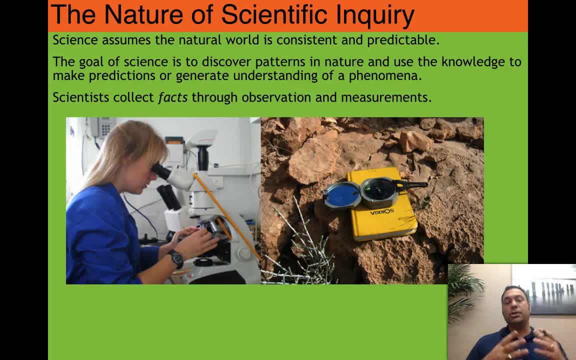 It's done by Africans. It's done by South Americans. There's geological institutes worldwide. 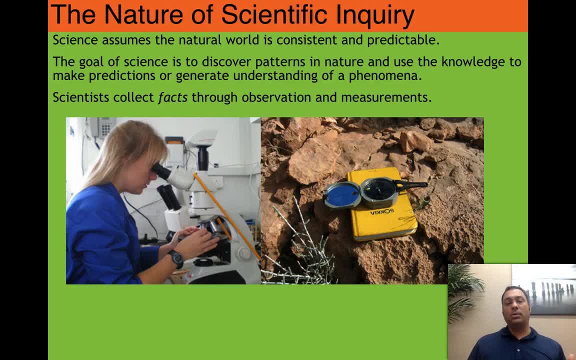 The Earth, like I said, is something that almost all people consider that they have in common, unless, of course, they're floating around on a raft. 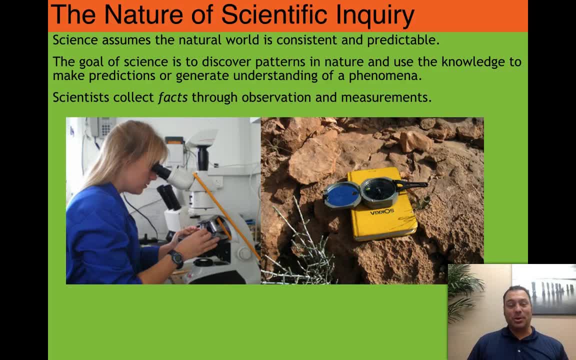 You know, then in which case they would be more interested in what the ocean is doing. 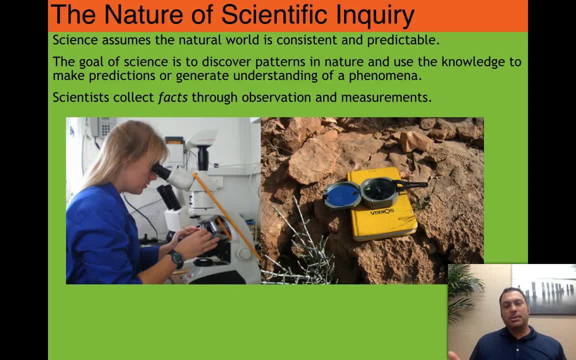 But almost everybody recognizes the supremacy of importance of the Earth. Okay? 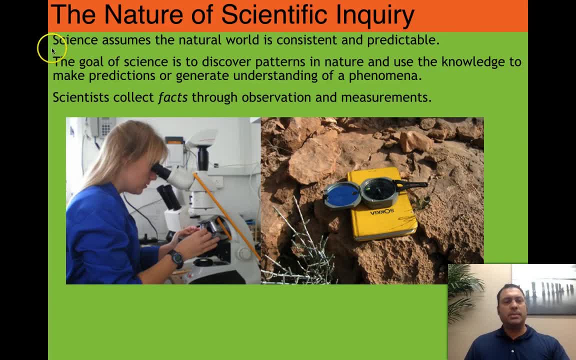 So when we apply science, remember the assumptions are that science assumes the natural world is consistent and predictable. 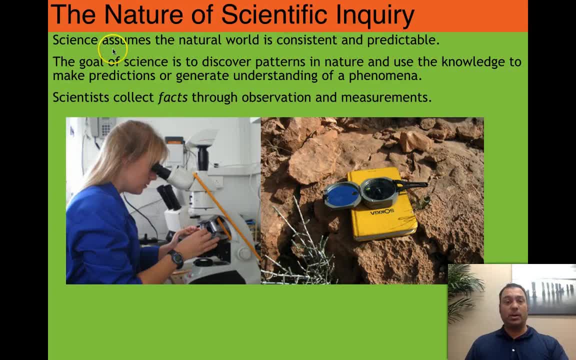 That's an assumption. It could be a fallacy. It could be wrong. But so far we have seen no reason to believe that that isn't so. 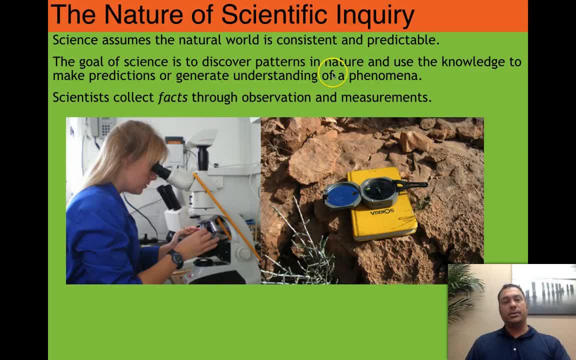 And the goal of science is to discover patterns in nature. It's not actually to get answers. Sometimes we don't get the answers. 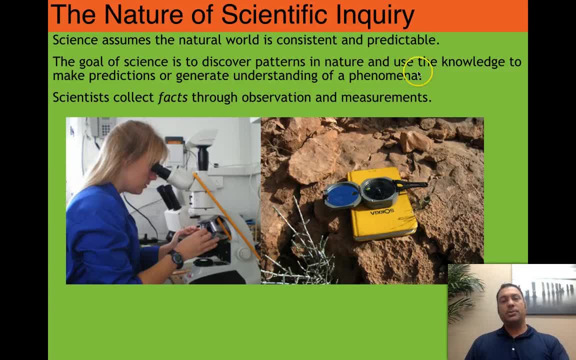 We just see the pattern. Patterns in nature and use the knowledge to make predictions or generate understanding of a phenomenon. All right? You might say, well, big deal. Well, it's important. 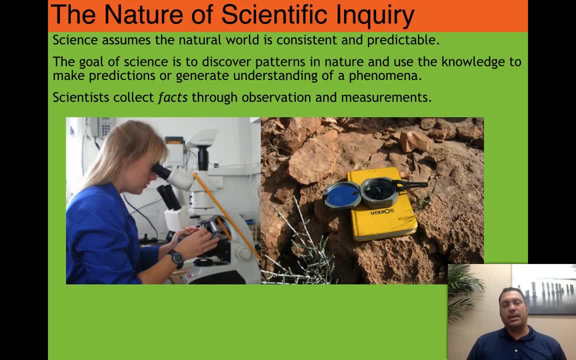 The reason why it's important is that if you build a building, for example, say a 10-story skyscraper, you're hoping that the engineer that built the building or designed the building 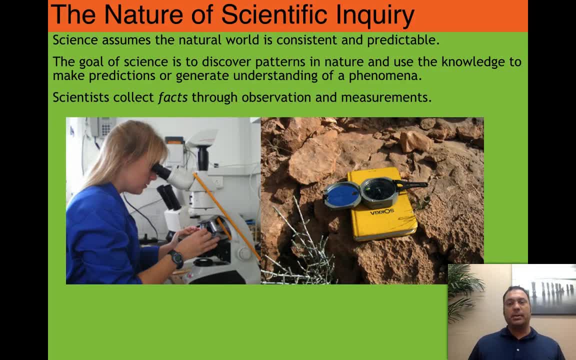 compacted the soil properly and built it on proper substrate so that the building doesn't fall over. 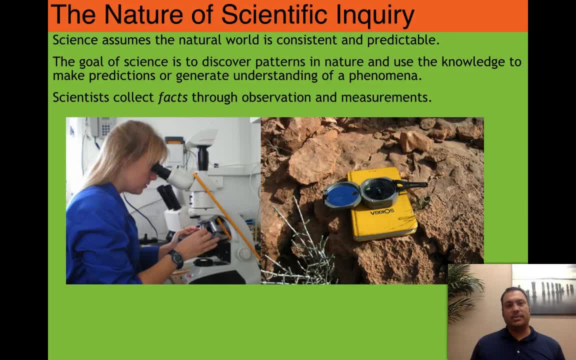 But how does he know that in advance? He has to have the science. Right? The science is going to tell him 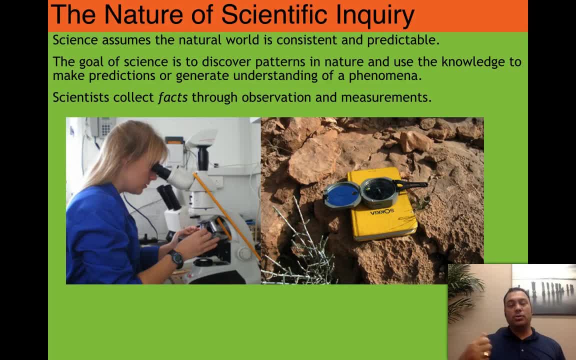 what the pattern is in nature and how to apply that understanding to a problem. Scientists collect facts through observation and measurements. 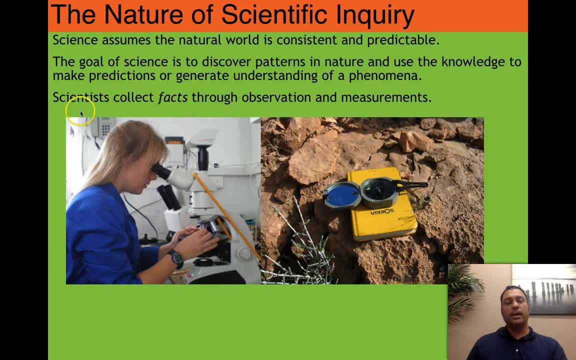 Another way of saying facts in Latin is data. Right? So scientists collect data. You could think of it this way. And so here we see a woman geologist 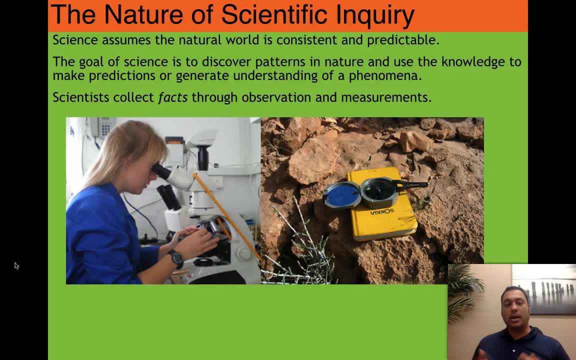 working on a microscope. Now, we're talking about that geology is not always conducted exclusively outdoors. 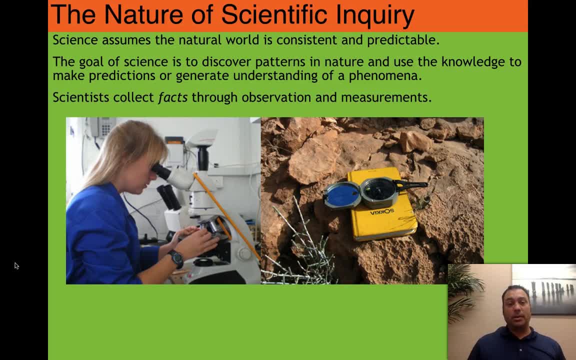 It's actually done frequently inside of a lab, looking through microscopes, being able to figure out what the minerals are telling us. 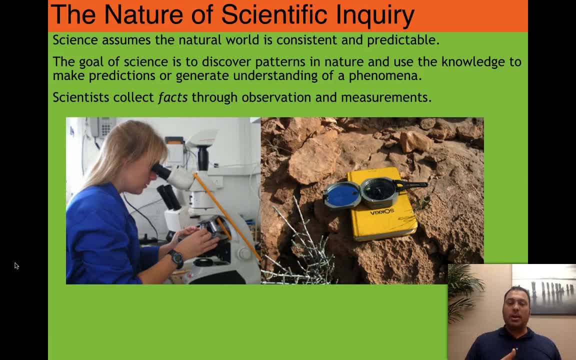 One of the growing fields right now where we're looking at minerals 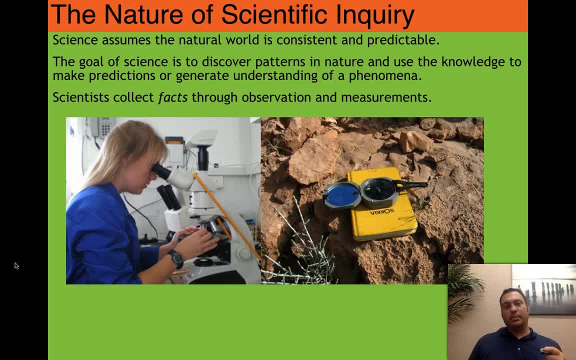 is forensic geology. People that commit a crime, maybe an atrocious crime, and then they hide, say, the weapon of the crime or they hide a body or something like that, and then they get mud on their shoes. 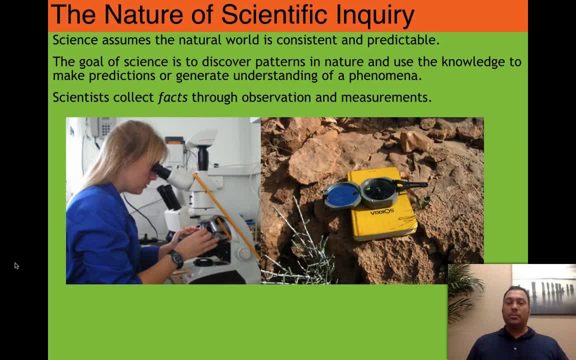 We are now able to track dust and dirt from crime scenes back to individuals if we have proper training on how to do that. 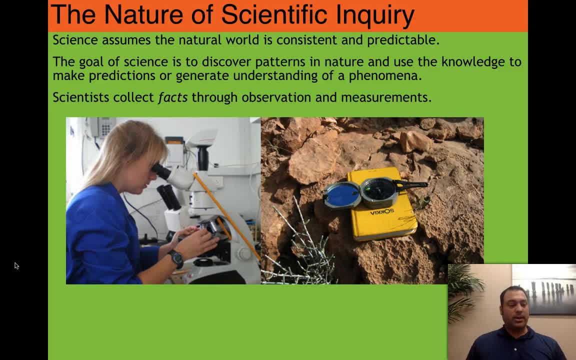 Of course, that doesn't mean that we don't do old-fashioned field geology. These are two common things, 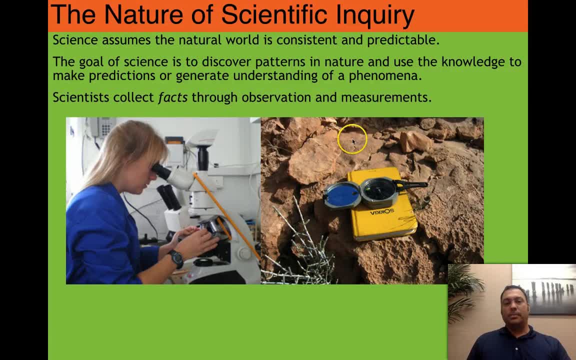 a Brunton compass and a yellow field notebook. These are carried almost by all geologists in the field, even when they are on vacation, quite frankly. 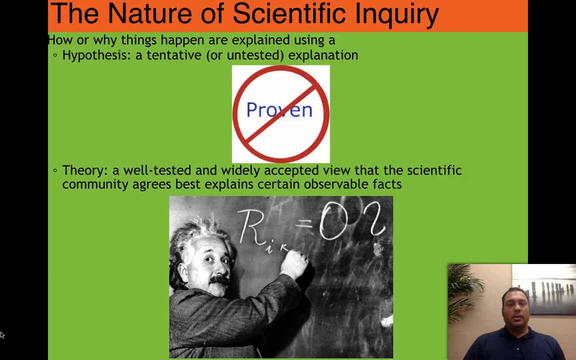 I take mine with me almost everywhere I go. How or why things happen 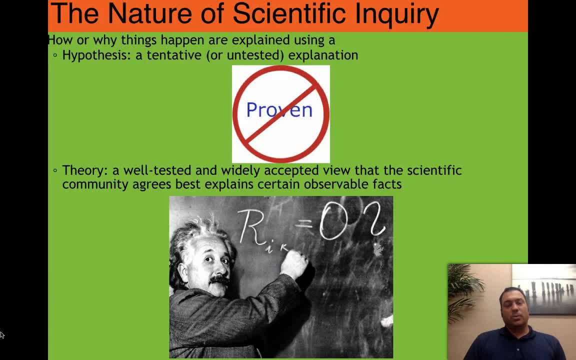 are explained using a hypothesis. The way that we go about the scientific inquiry is to put together a hypothesis, which is a tentative or untested explanation. 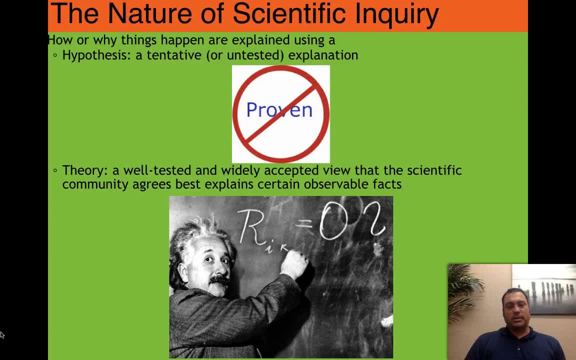 You can have almost an unlimited number of hypotheses. Charles Darwin, when he came up with his idea that we now call evolution, he never came out and said, I think things are moving, or life is evolving. 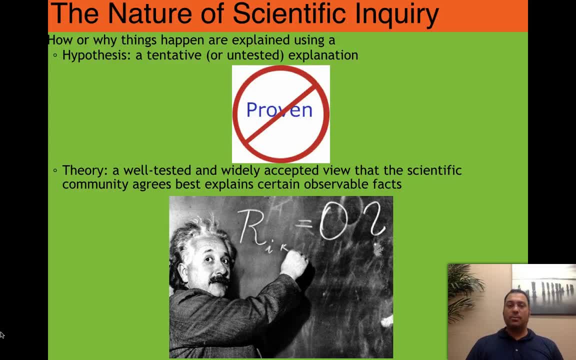 What he did was he had a whole bunch of hypotheses about what he thought was going on, and he started eliminating them until he found one that he could no longer eliminate. It was the one that we now look at as one of the principal axioms in biology, which is evolution. 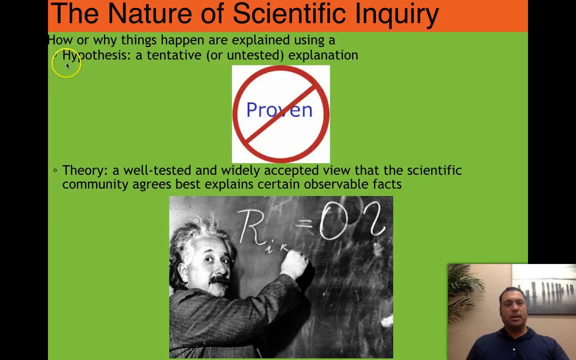 A theory is different from a hypothesis. A hypo means a pre-thesis 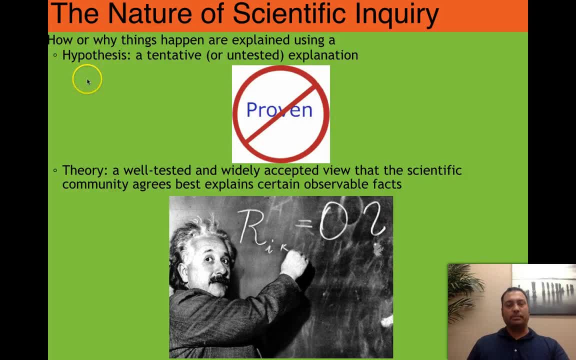 or before you actually have a full understanding. 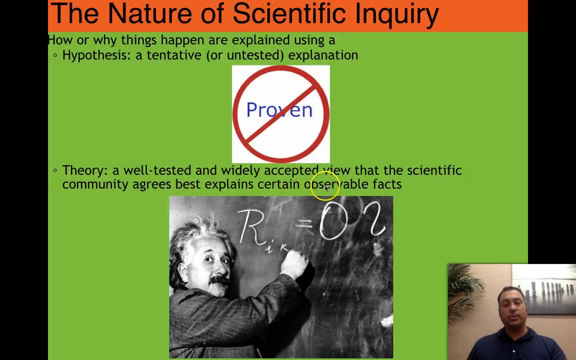 A theory is a well-tested and widely accepted view that the scientific community agrees best explains certain observable facts. 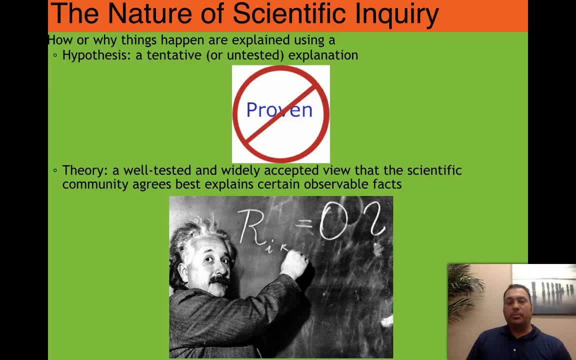 One of the most obvious people we think about when we do theories is Albert Einstein and his theory of relativity. 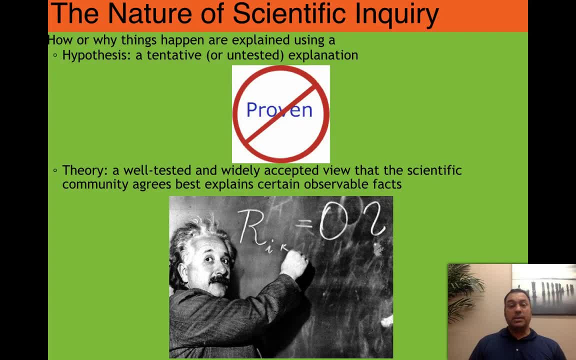 It turns out that Einstein's theory of relativity basically piggybacks on some problems that Sir Isaac Newton's equations couldn't explain. 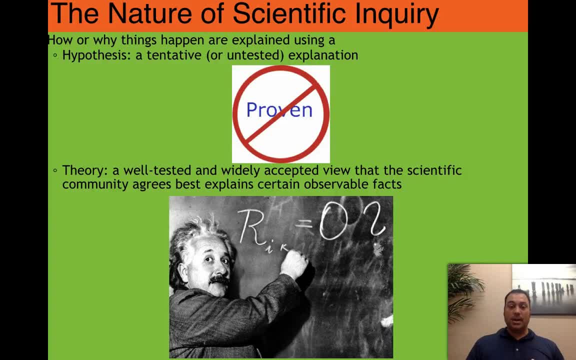 Einstein's ideas did come and actually explain some of the inconsistencies and kind of in some ways replaced Newton. 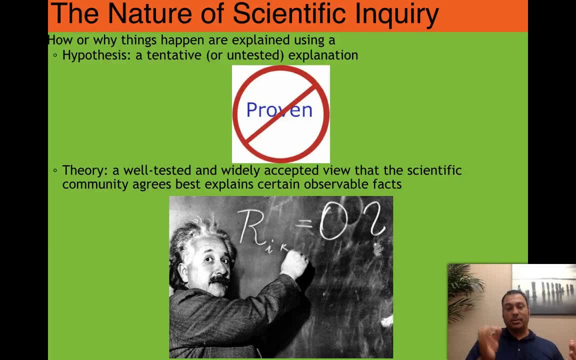 It doesn't mean Newton isn't valuable to us, but Einsteins are basically really good 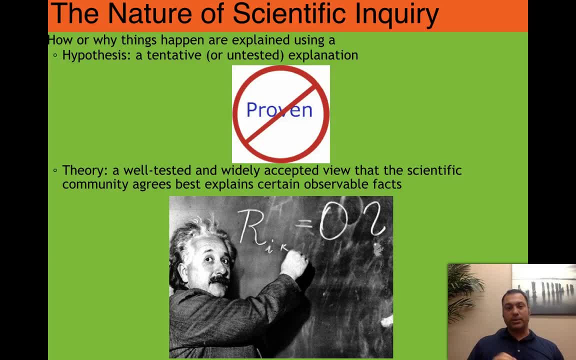 if you're into rocket science or studying particle physics. 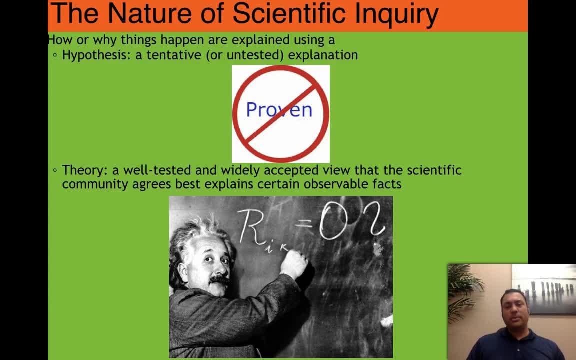 But it turns out that it is incompatible with other theories, and so we still have a long ways to go on these things. 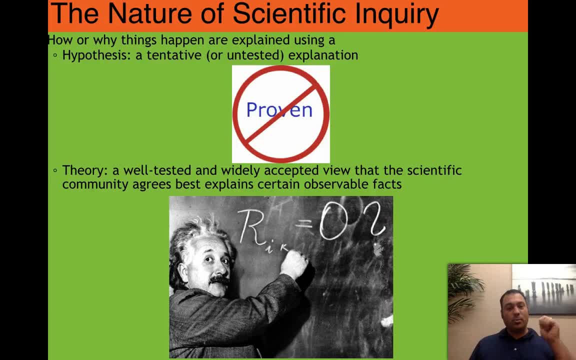 So certain theories, sometimes it's like a tool in a toolbox. We know that it works for this, but it won't work for that. Geology is the same way. 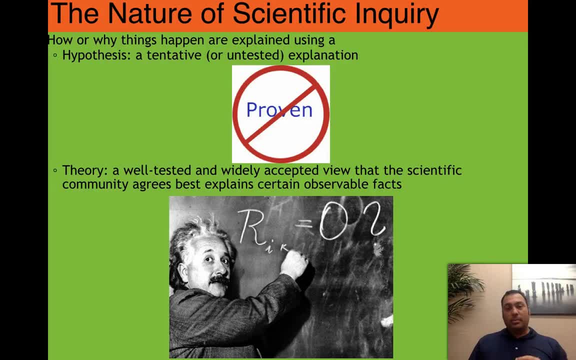 Einstein's theory of relativity is the same way. Evolution is the same way. 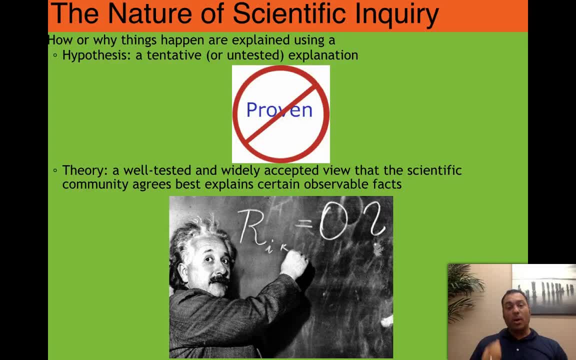 Sometimes it's really easy to get the what, but the how or the why can sometimes be painfully inescapable or ungraspable. 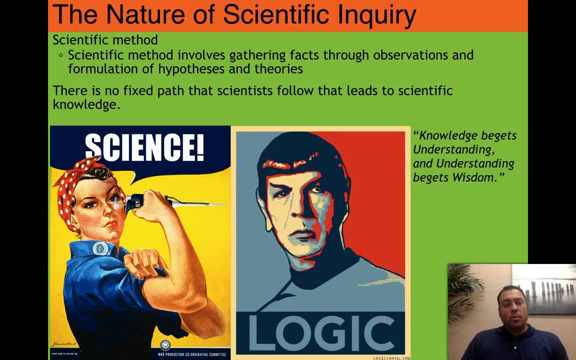 So what is the nature of this inquiry? Well, the scientific method is what we utilize to kind of do this process, right? You can't just have a hypothesis and go right to a theory, okay? 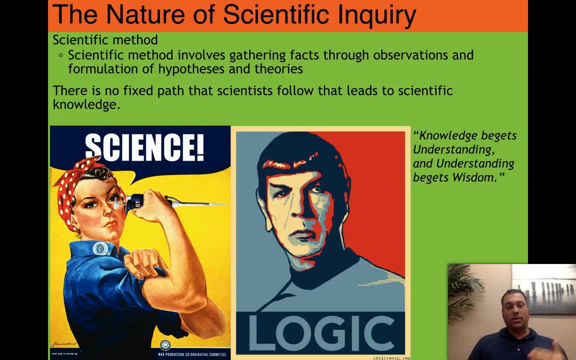 There's a process that falls out as we go through. 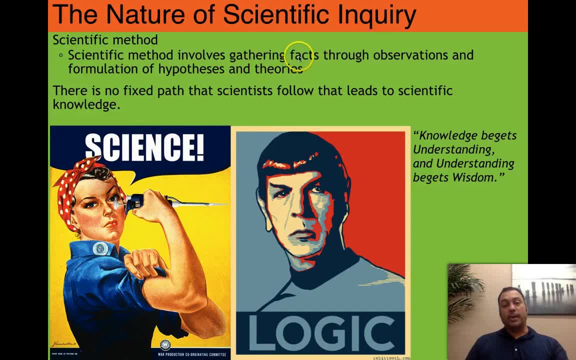 So the scientific method involves gathering facts, or data, through observations, right? 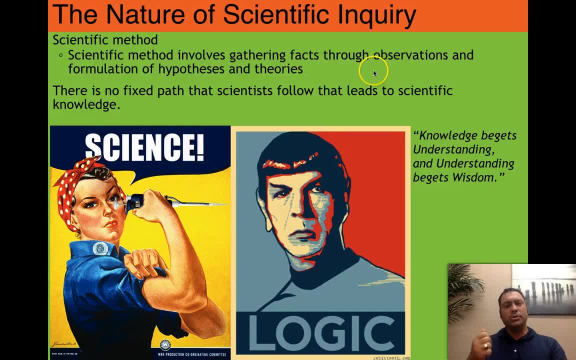 And when we say, how do we do that? We've got to take measurements, right? It usually means you're taking a ruler or something that you can write down in your notebook. 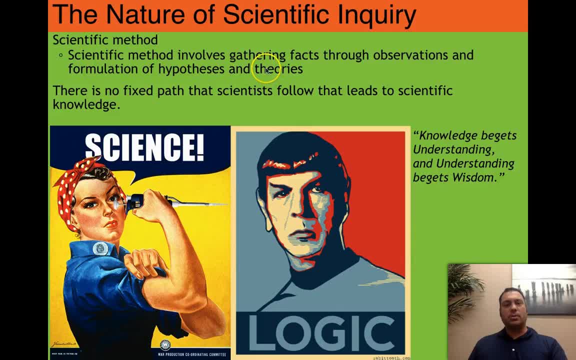 And formulation of hypotheses and theories, right? So not only do we have, you know, we have to have reasonable formulation of hypotheses and theories. 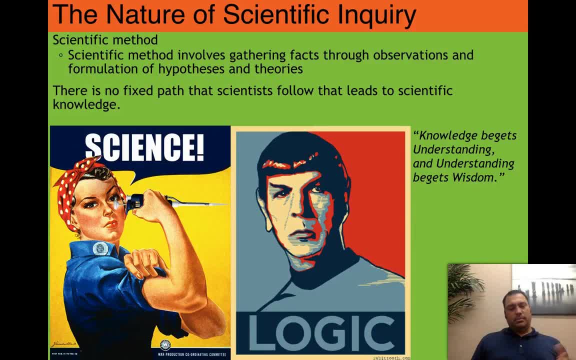 It's not something we can just say, well, most people won't say, well, you know, there's a river here because God made it. 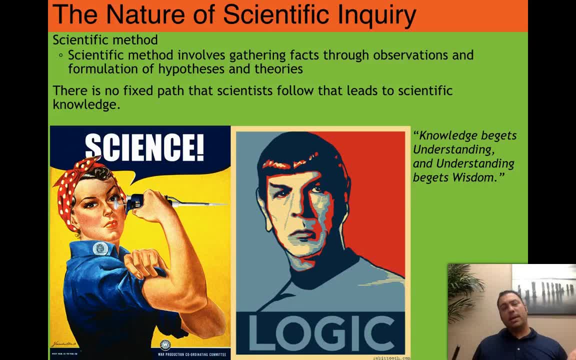 Now, people have in the past had that hypothesis, but the scientific method says, let's not approach it that way, okay? 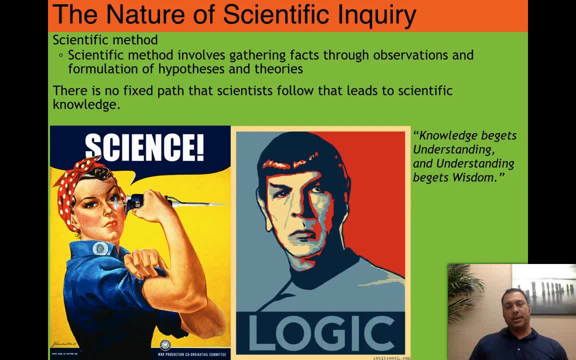 There might be a more pragmatic or practical understanding of why that river exists where it does, all right? 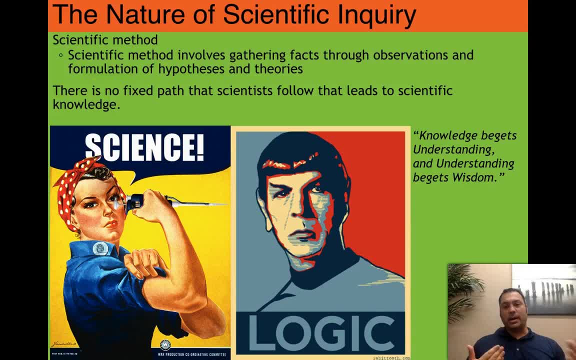 You'll find that as I go through the class, I'm most certainly not anti-religion, but a lot of phenomenon that are usually immediately chalked up 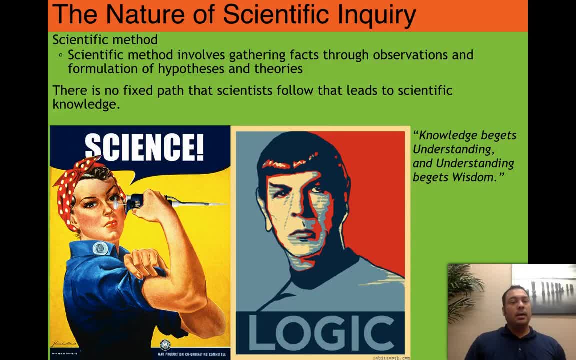 as religion can be explained in a scientific way. 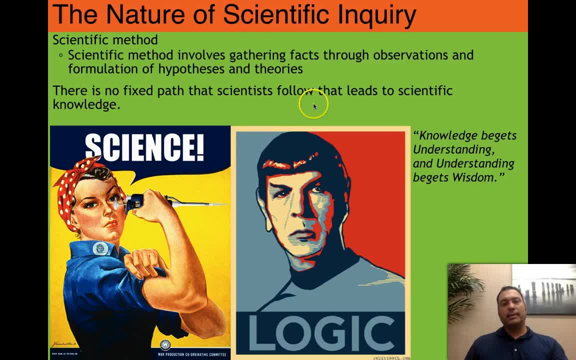 With that said, there's no fixed path that scientists follow that leads to scientific knowledge. Right? 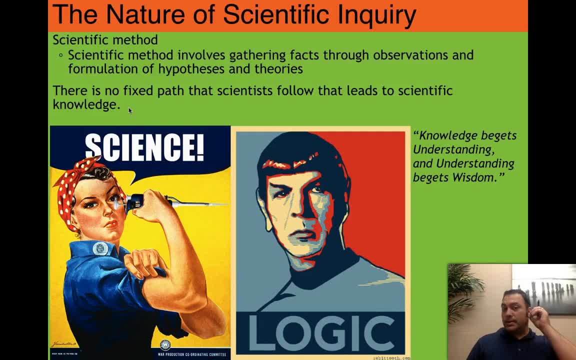 There's many different paths. You'll actually see scientists, those of you that wind up graduating with a degree in science, 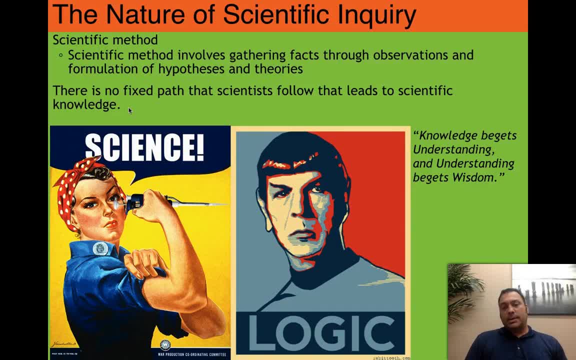 will observe yourselves, that scientists will sometimes look at the same problem 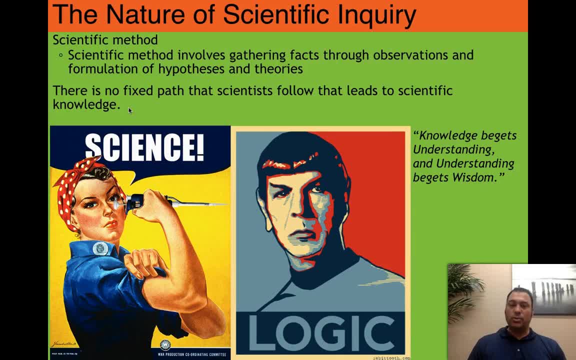 and get completely different answers because they have different tool sets that they bring to bear. 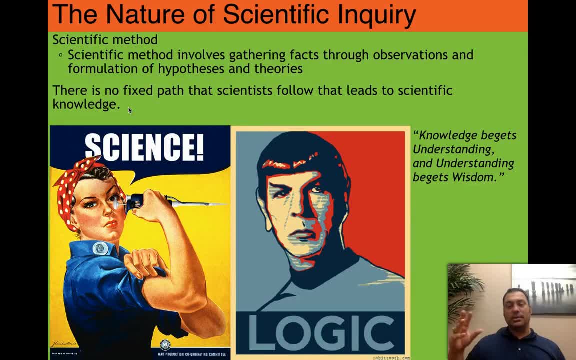 You know, maybe one is a chemist and another one is a physicist, and so they apply their own tools and they come up with different answers. 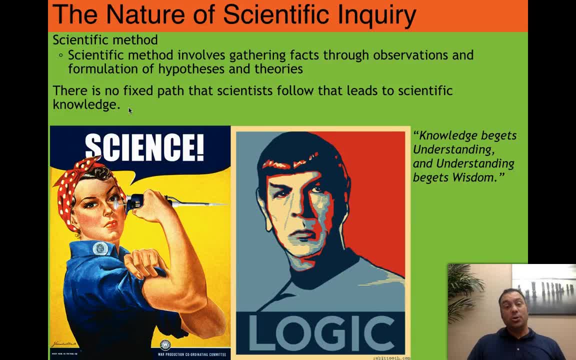 But when they both get the same answer, that's usually pretty enlightening stuff. 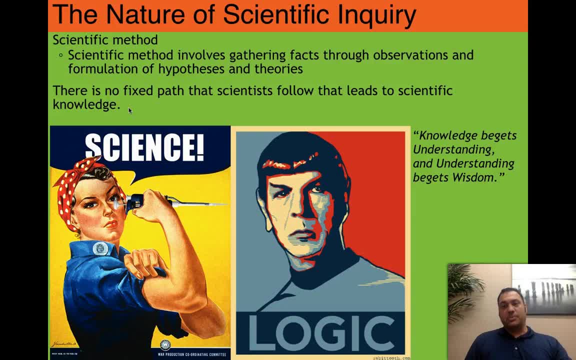 One of my things that I'm kind of famous for saying is that knowledge, all right, knowledge begets understanding, and understanding begets wisdom. Right? So, yeah, this goes for everybody. 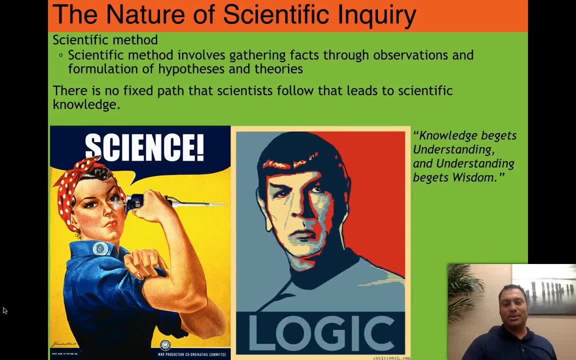 You know, this is one of my science fiction heroes, Captain Spock. He's all into logic. And basically logic is what leads you down this path from knowledge to wisdom. All right. 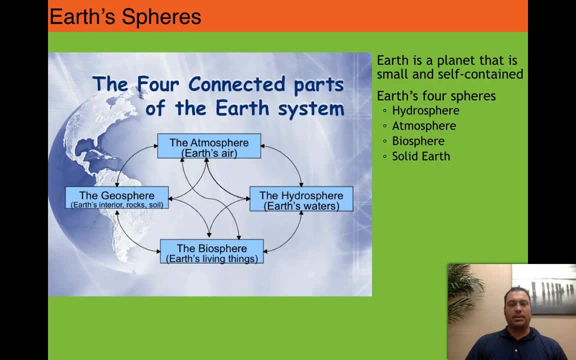 So we've kind of talked about what the science is, and I'm going to jump off that at this point. 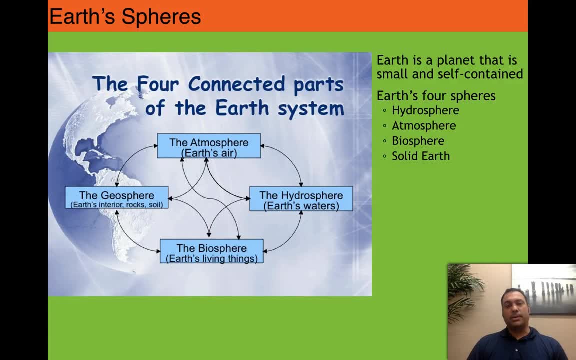 If you're interested in the scientific method, it's probably better to take a philosophy class that explains this in more detail, or you can just send me an email and I'll, of course, discuss it with you. 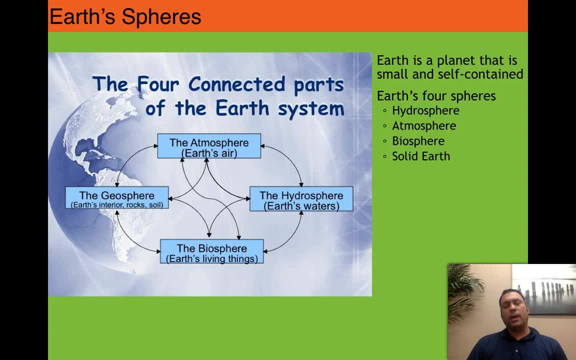 But the four connected parts of the Earth, well, I should say, the Earth is connected in four separate parts. The main part is going to be the geosphere. That's what we're concentrating on. The four connected parts. The geosphere is here. This is the Earth's interior. It's rocks. It's soil. 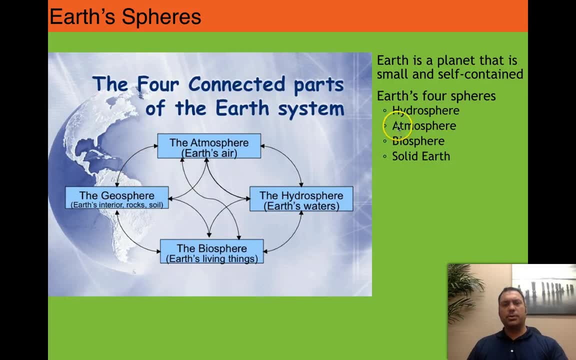 But there's other spheres here, too. There's the hydrosphere, which are Earth's waters, right? Here's the hydrosphere. The biosphere, Earth's living things. 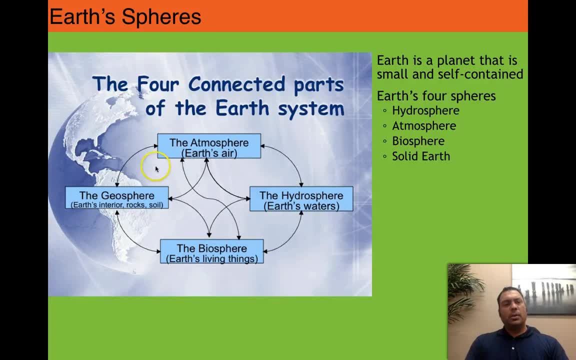 And the atmosphere, Earth's air. And they're all interacting one with another. 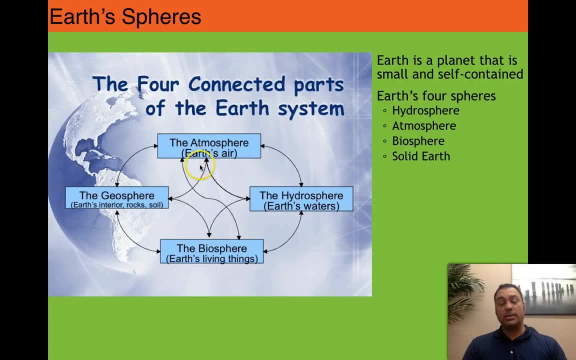 The geosphere is interacting with the atmosphere all the time to create things like soil. The atmosphere is interacting with the hydrosphere, which creates clouds and distributes water and is actually the source of rivers. 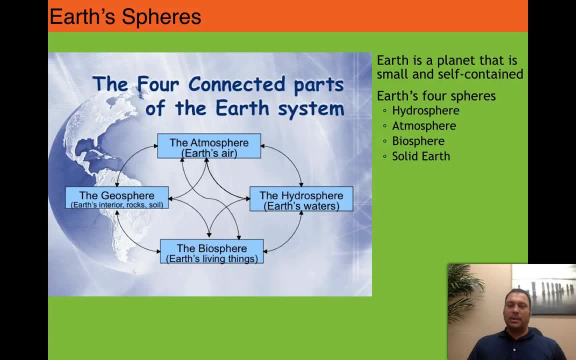 The biosphere, of course, we've done drilling in some of the most remote places on the planet to very deep depths. And even in those rocks, when we've done analysis to try to find truly dead rocks where nothing has ever been, we still find, even there, viruses and microbacteria. So the biosphere is everywhere. 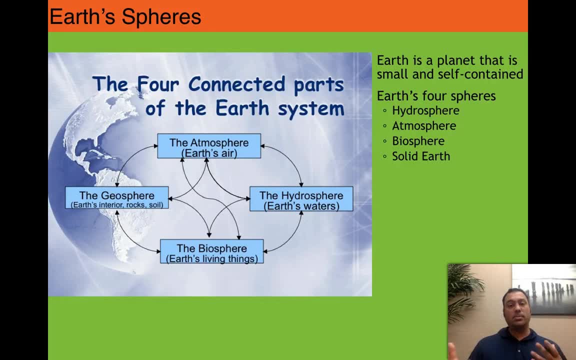 The atmosphere is everywhere. And the hydrosphere and the geosphere. And they're all going to be interacting. We're going to be talking about those interactions throughout the class. 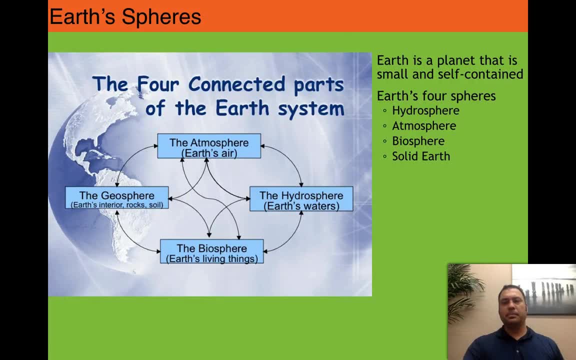 But for the most part, we're going to be emphasizing here. 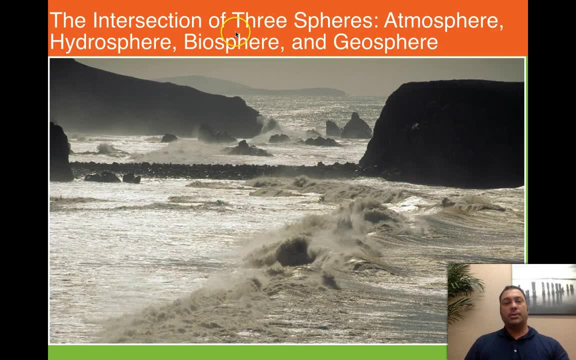 So here we see the interaction of three spheres. I actually altered this slide right before I put it up. I should say actually the four slides. 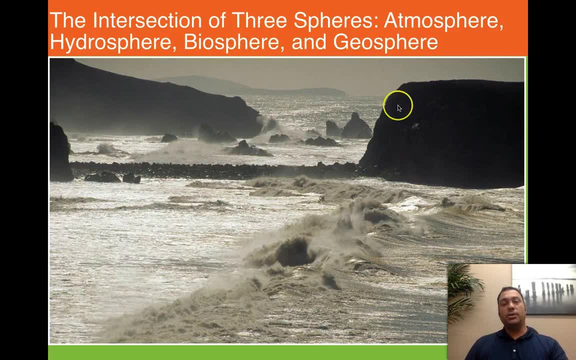 This would be the atmosphere, the hydrosphere, and the geosphere. 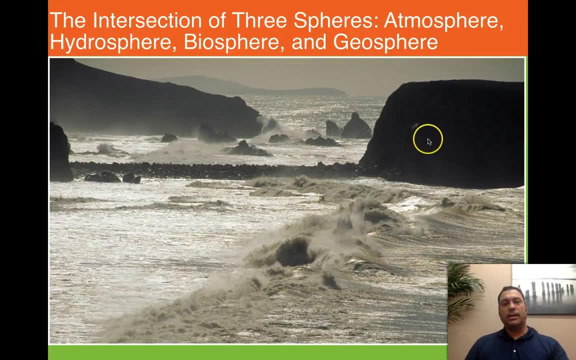 Here we can see the hydrosphere, the geosphere being these rocks, and, of course, the atmosphere being the air, the mist in the air. 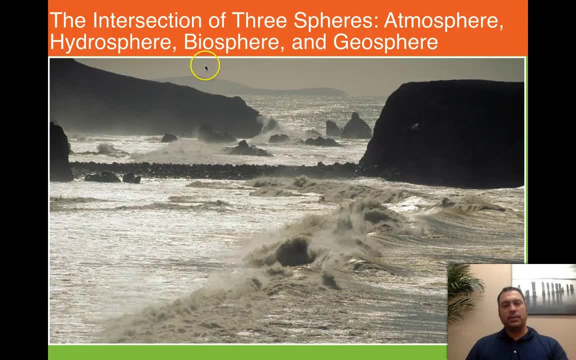 But I added biosphere right at the last minute because the biosphere is actually residing in the rocks and in the water. 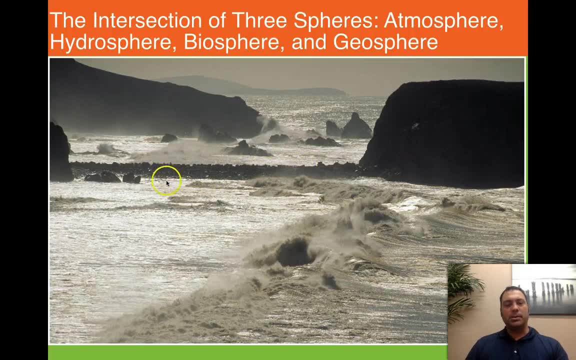 And if we were to look over here, you'd actually see birds and crab and things like that. They're all here. All four of them. 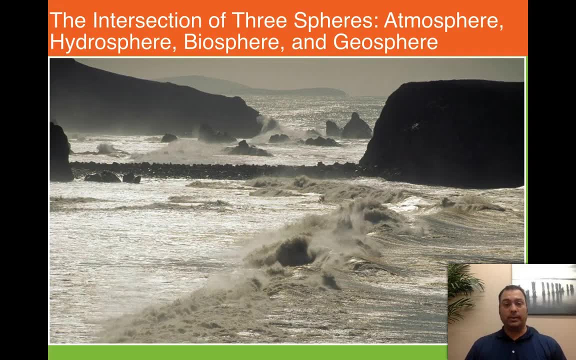 And the best place to look at this intersection, of course, is the coastline. 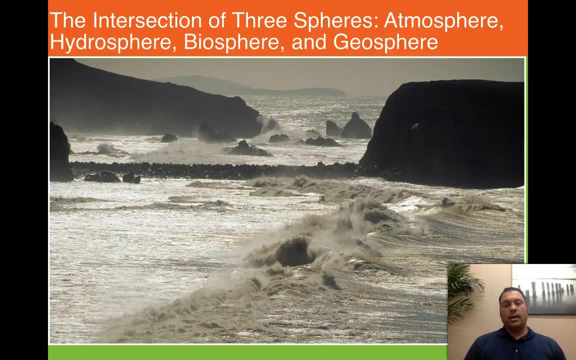 If people wanted to have a really good understanding of how healthy the Earth is and where kind of the environmental front line is, 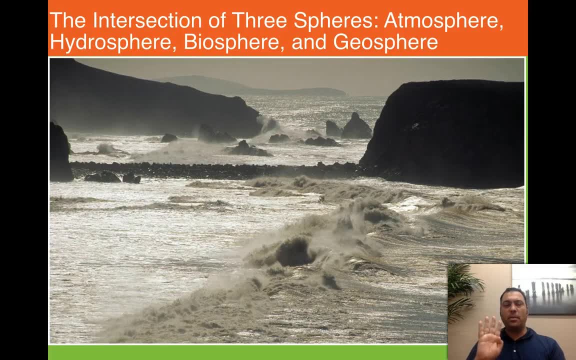 it's to go down to the coasts because that's where you see the four major spheres all interacting. 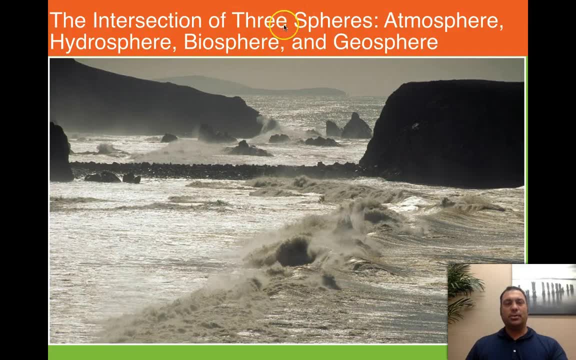 So forgive me, future lectures I'll change the three to a four, but all four spheres are being represented here. Okay? 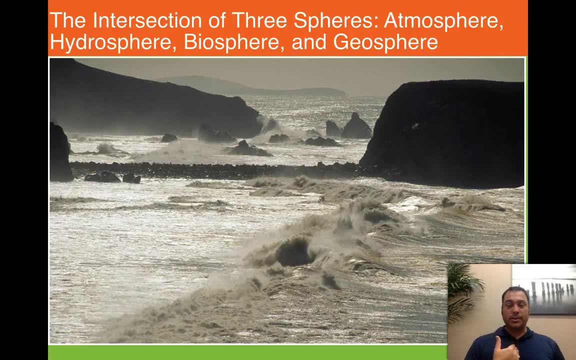 And so as my own training, I'm a coastal geologist by training. When I look at these things, I immediately see all kinds of different things that need to be investigated to find out how healthy this coastline is, how healthy this ecosystem is, and how sustainable the system is for future generations. 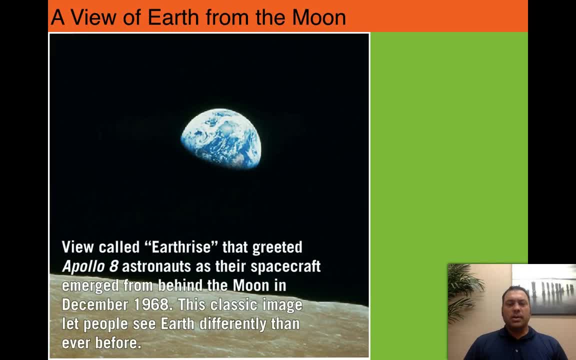 So to understand the Earth, we need to understand what it is. The Earth is a planet. 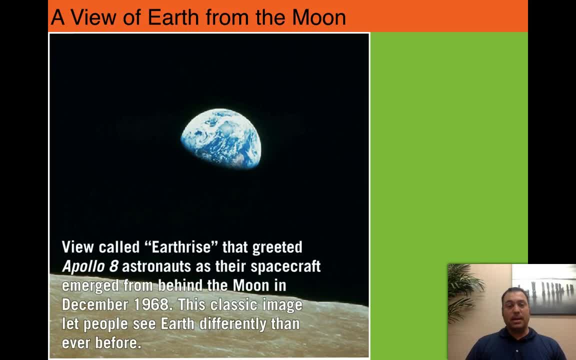 This is a picture of the Earth taken by Apollo 8 astronauts. 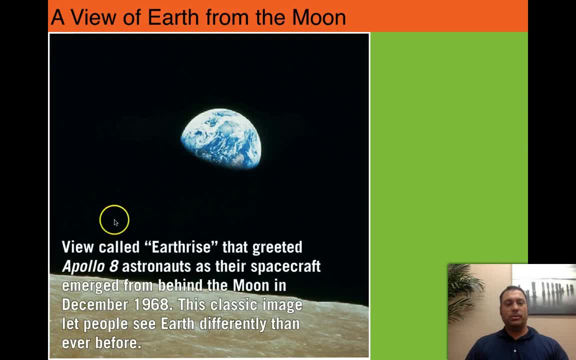 Apollo 8 did not land on the Moon. This is the Moon down here. But what they did was they did leave the Earth. They left Earth gravity. 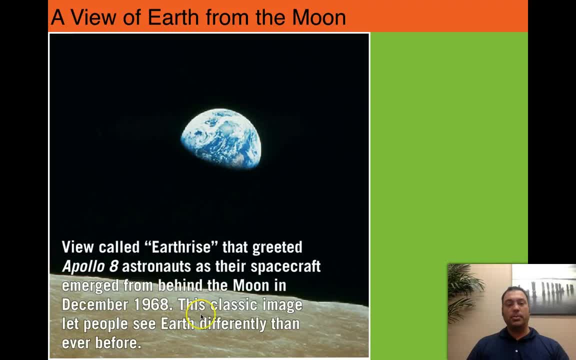 They actually were captured by lunar gravity. They orbited the Moon and then returned back to the Earth, almost like a figure eight. But as they came back around the Earth, they're the first persons, these astronauts, to ever see the Earth rise above the Moon. Okay? And quite frankly, nobody's seen it since the 70s. 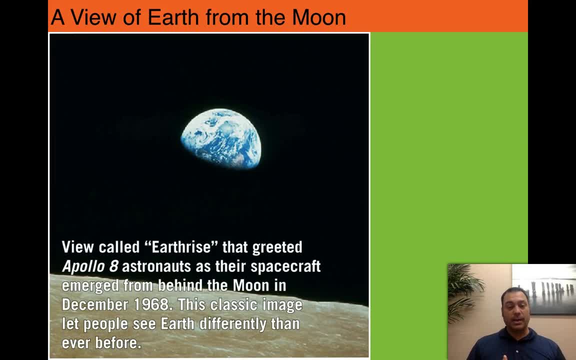 Humanity has not returned to the Moon except through satellites since. 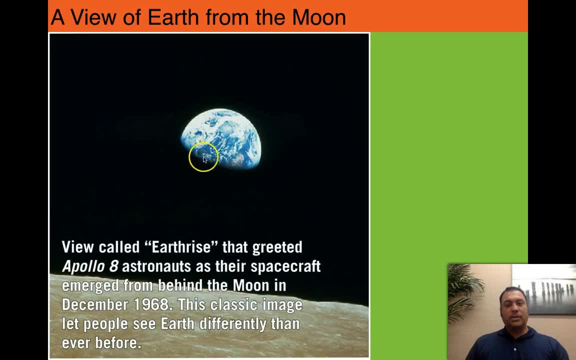 And this picture was taken of the Earth from the Moon. It's one of the most fascinating pictures if you think about it. 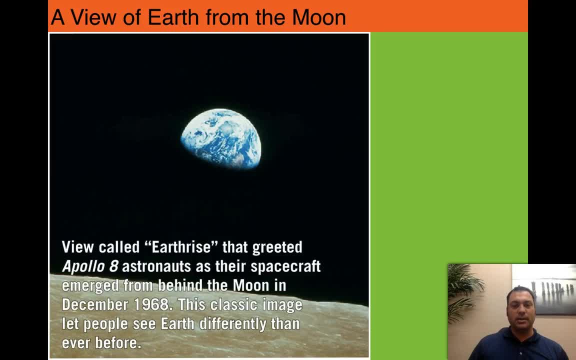 There's a lot of really interesting things kind of said in here. First off, we can see weather patterns. 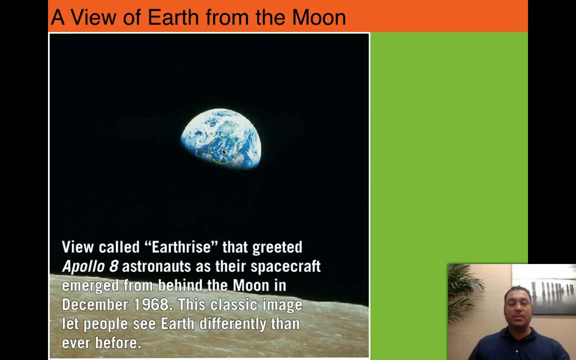 We can see the land. We can see the oceans. Even from a distance, we can see those spheres interacting from a very far distance. 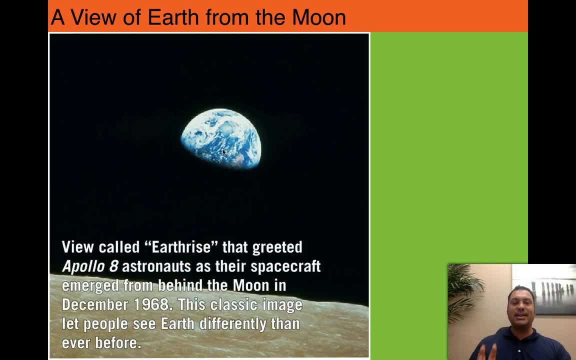 So the Earth is a dynamic place even from an objective viewpoint, even from the Moon. By comparison, the Moon is dead. 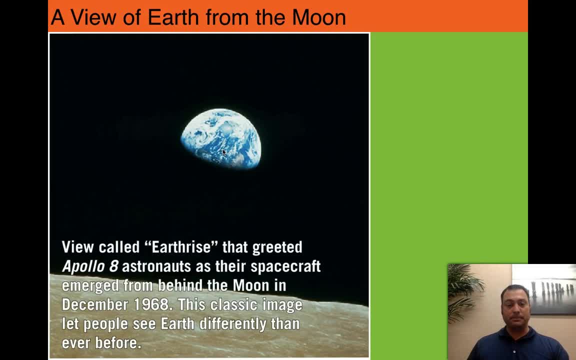 The Moon is boring and dead by comparison. Okay? 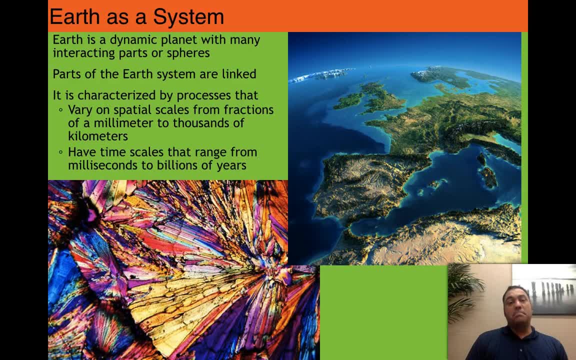 So the Earth is a dynamic planet with many interacting parts or spheres. Right? You know, I like to, I don't really like to say spheres so much, but that's in the literature and in the jargon, so I'll use it for a little bit. 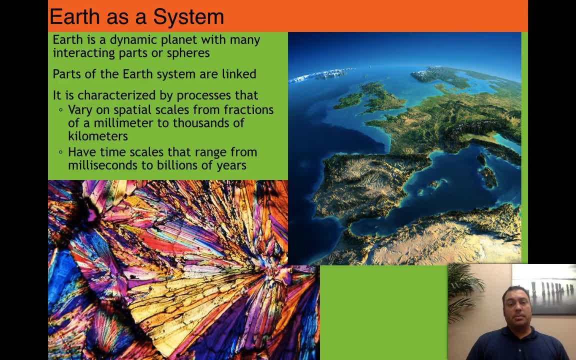 But it's interacting parts. And the parts of the Earth system are completely linked. 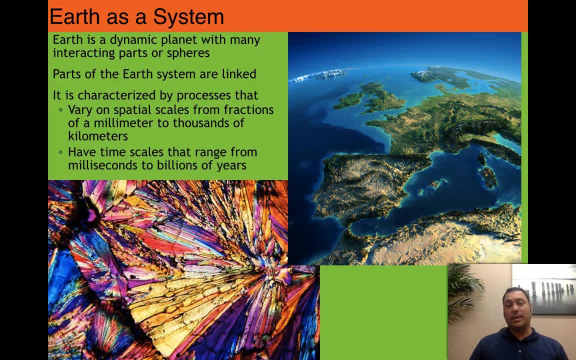 And it's characterized by different processes. So we got to think about scales. Right? 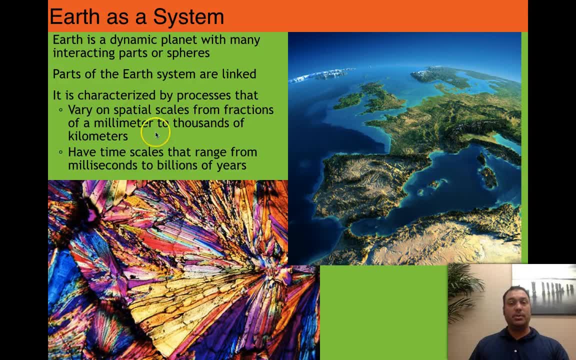 So they vary on spatial scales from fractions of a millimeter to thousands of kilometers. 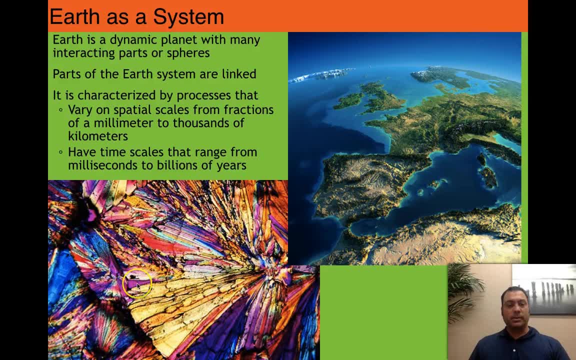 So these are tiny crystals that are forming inside of a rock. 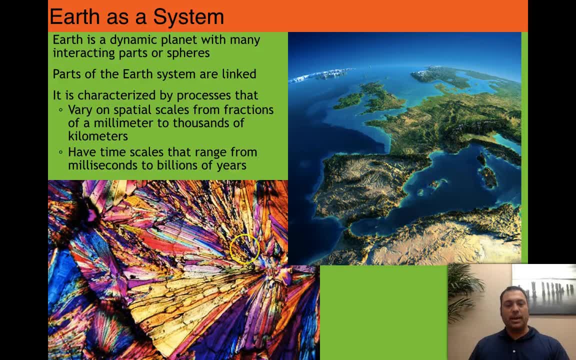 And here we can see the crystals originate here. They blade out in every direction. 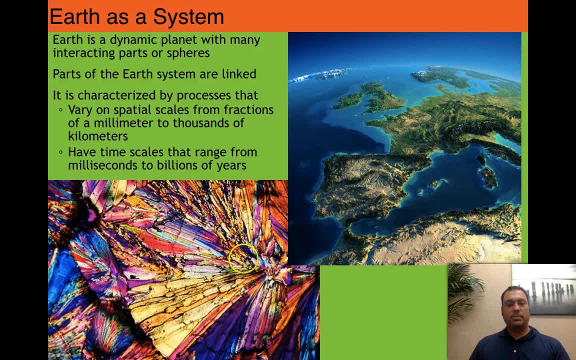 But these are visible only under a microscope. And here we actually see another one blading out like so. 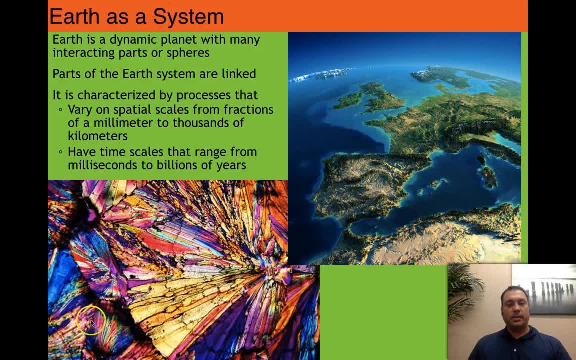 Another one blading out like this. Okay? Beautiful rock. Right? 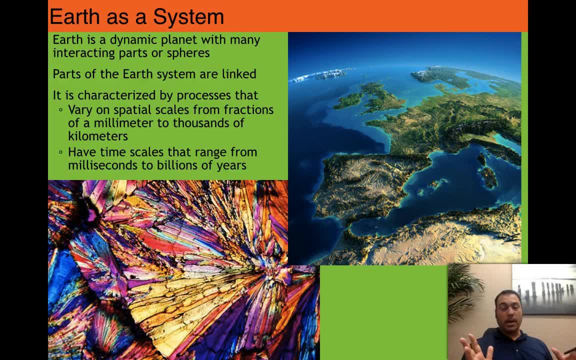 Beautiful minerals under a microscope. But we don't actually see that with the naked eye. We have to have the tools to look at them. And we're going millions, or I'm sorry, to millimeters. We're going to millimeters of a meter. Thousands of millimeters. Thousands of a meter. To be able to see these things. And even smaller than that sometimes. 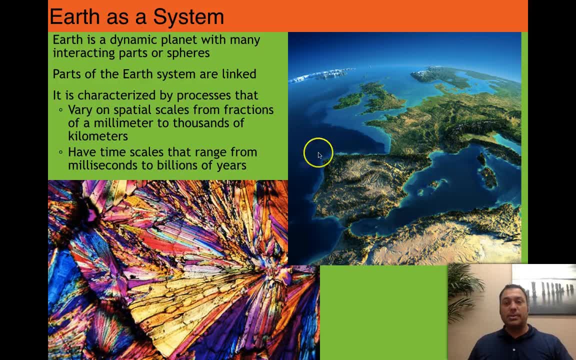 By comparison, we can look at satellite images. 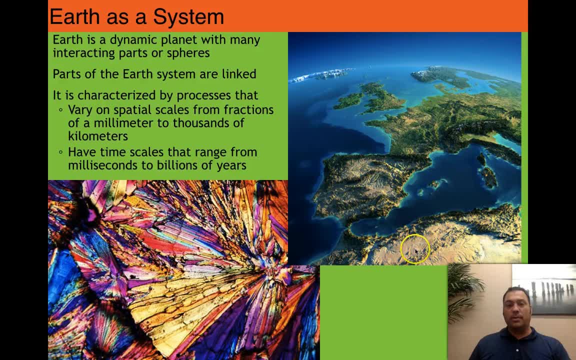 And here we see Western Europe. Here's, and North Africa of course. 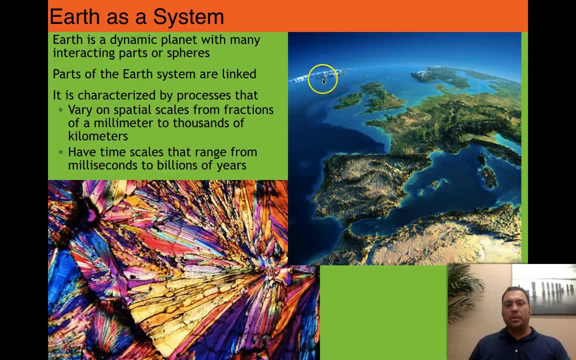 And over here is, I believe, Greenland. Or Iceland, I'm sorry. 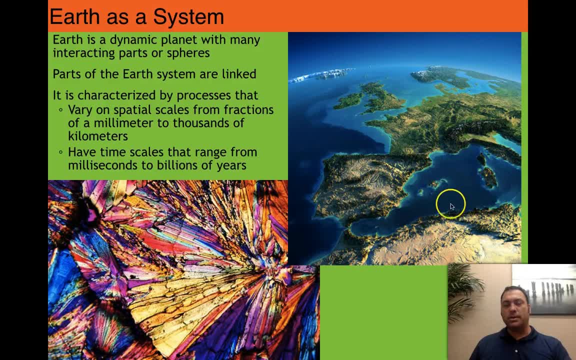 So here's what we see in North Africa. The Straits of Gibraltar. This is the Mediterranean Sea. The distances here are thousands of kilometers of distance. Right? Whereas this is just millimeters. Very, very small. 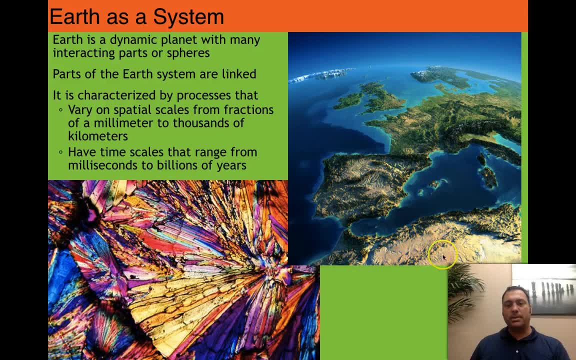 Here's the Sahara Desert. Right? Of North Africa. There's basically nothing out here. Right? 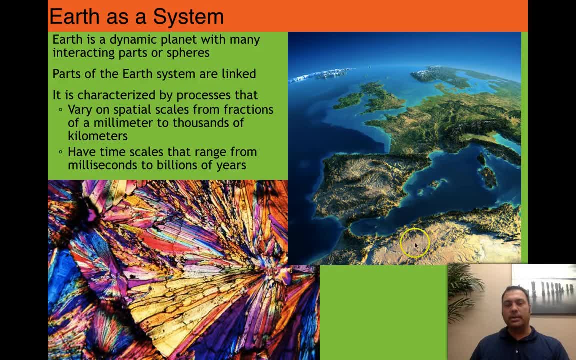 Libya is located right about here. All right? Right in this area here. 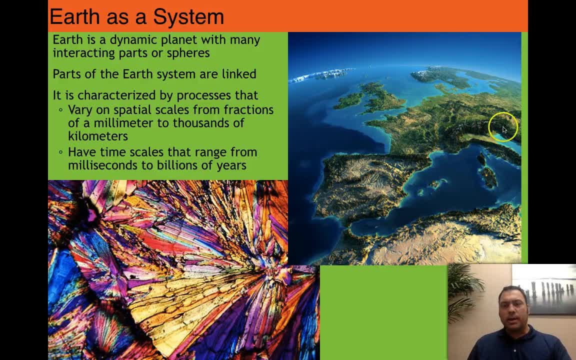 Morocco. These mountains, right? 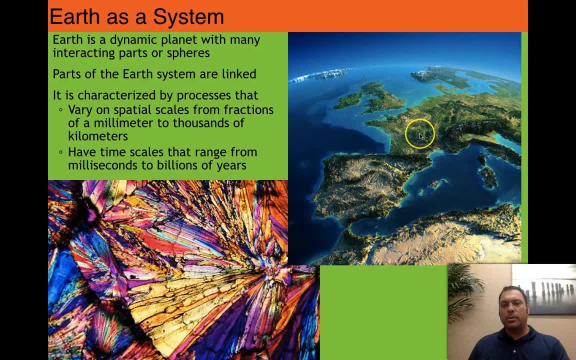 Here we see Italy. Why does the geography between Northern Europe and Western Europe exist? Well, look at the Alps. 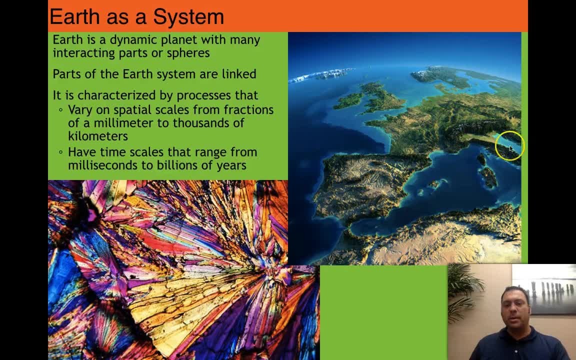 These are the Alp Mountains that separate Italy from the rest of Europe. Which allowed separate cultures and unique identities to flourish in this part of Europe versus this part. 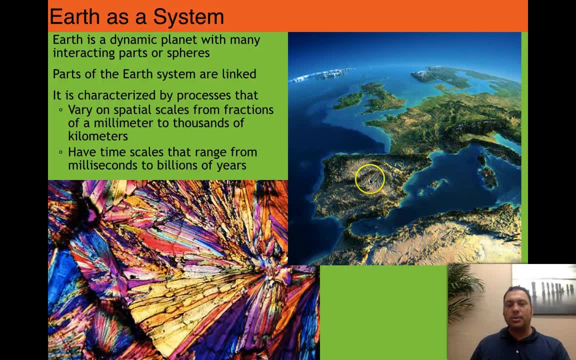 The same thing here. Why did French get spoken here and Spanish get spoken here? What's the big difference? Look at these mountains. Right? We have the Pyrenees right here that are blocking this whole area. 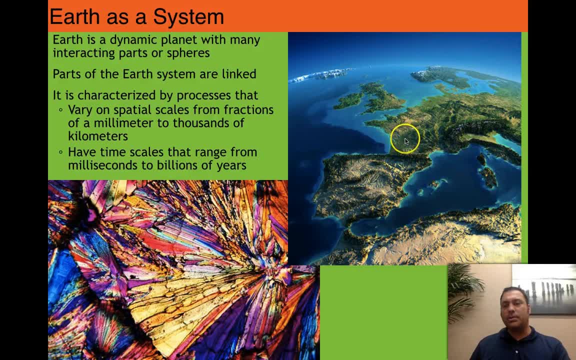 What about England? Why did England separate itself and have its own culture? 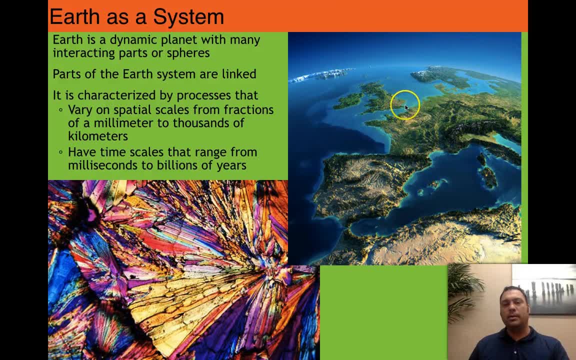 Again, the geology played a role. Look at this right here. Okay? England is a, or actually Britain is an island, of which England is a country on that island. And here's Ireland over here. Again, each one of them having separate cultural identities. 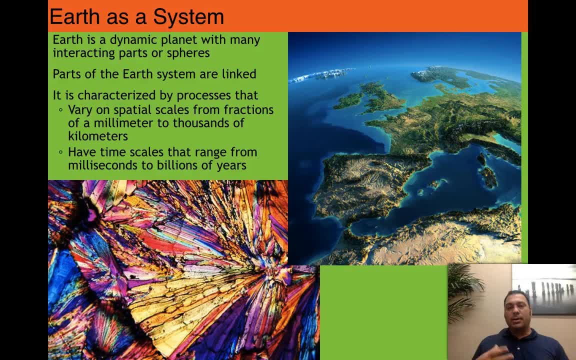 So, again, we see the interaction of the biosphere, which in this case is humans, having to deal with geographical barriers that are thousands of miles or thousands of kilometers long 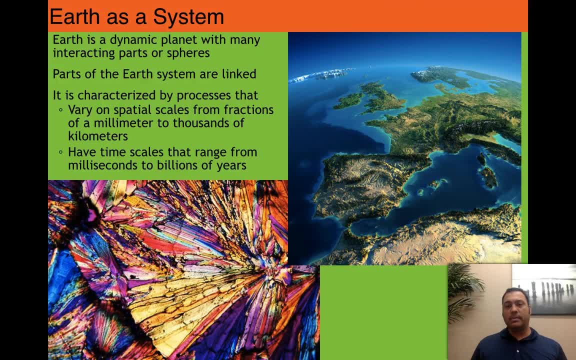 that have tremendous effect on our societies every day. This, of course, is Scandinavia and Russia back over here. 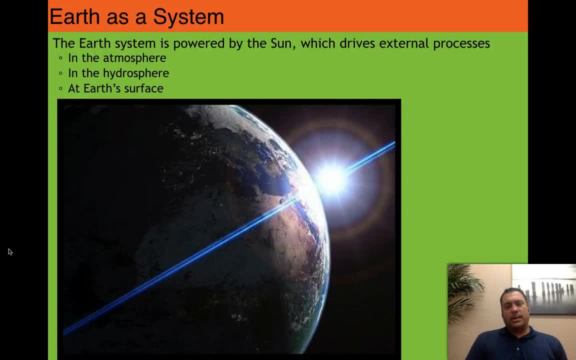 So the Earth as a system is powered by the sun, right? The biosphere, the geosphere, well, the geosphere we're going to come to in a little bit, right? It's not always powered by the sun. 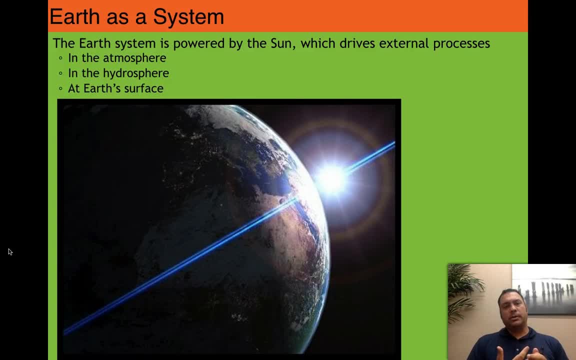 Some of it is. But largely the atmosphere, the biosphere, and the hydrosphere are powered by the sun, right? 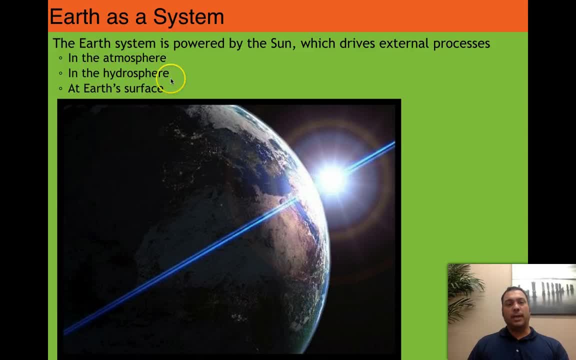 The sun gives energy directly to the atmosphere, to the hydrosphere, and at our surface, right? So when we go outside on a warm day, we can thank the sun for it. 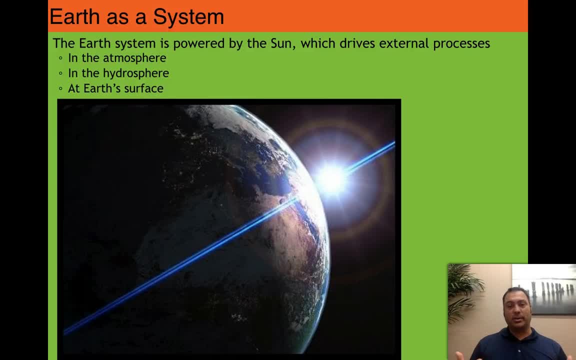 So the sun is always going to be life's best friend, right? Despite the fact that it has some effects, such as if you get too much exposure, you wind up getting cancer and things like this. 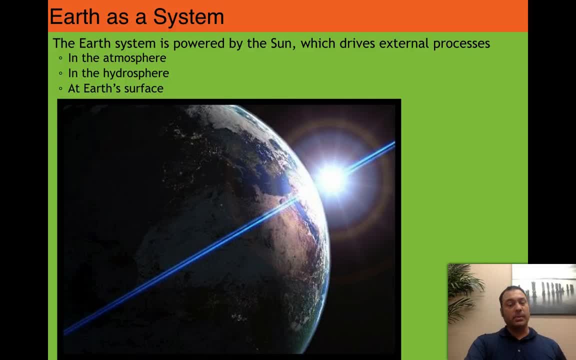 But if you don't get enough, you don't have any survival either. You've got to be able to balance it. 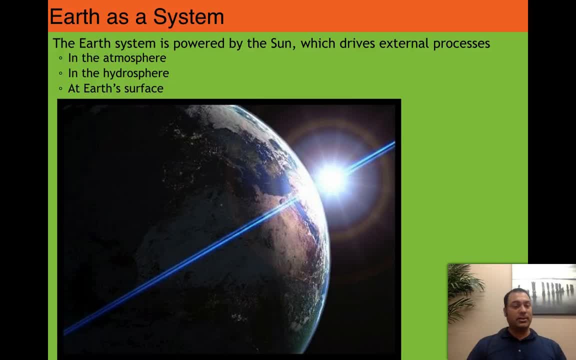 And the Earth, of course, being half in the sun and half in shade all the time, here's nighttime and here's daytime, is a great regulator, right? 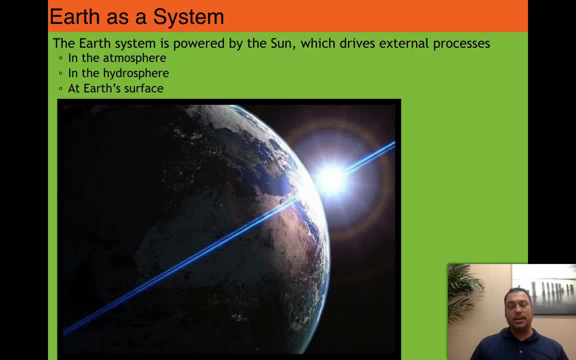 It gives humanity the opportunity to rest for 12 hours out of the sun. Amazing how our humanity is linked so closely, right? So tightly to the Earth as a planet. 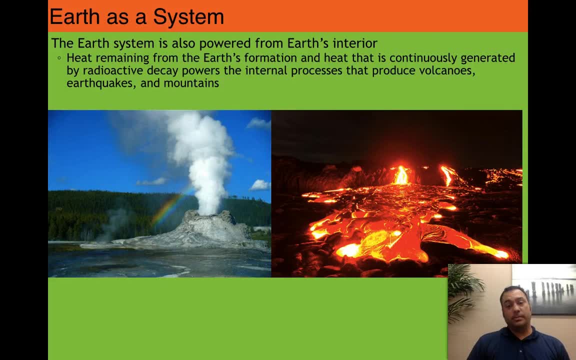 The Earth's system is also powered by the Earth's interior, right? So it's not all just solar power. Heat remaining from the Earth's formation and heat that is continuously generated from radioactive decay powers the internal processes that produce volcanoes, earthquakes, and mountains, right? 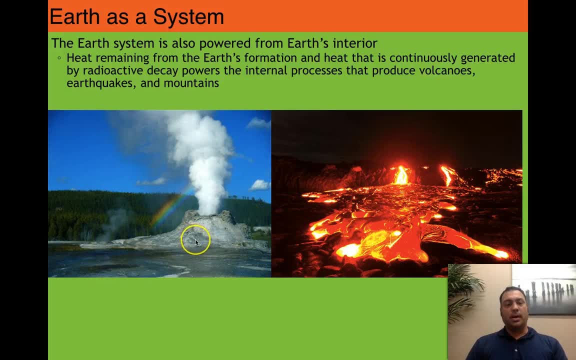 So here we see a geyser. This is Yellowstone National Park. The geyser is actually powered by internal heat from the Earth, some of it radioactive decay, some of it from the heat of formation of the Earth when you take two things and you slime them together during the Earth's formation. 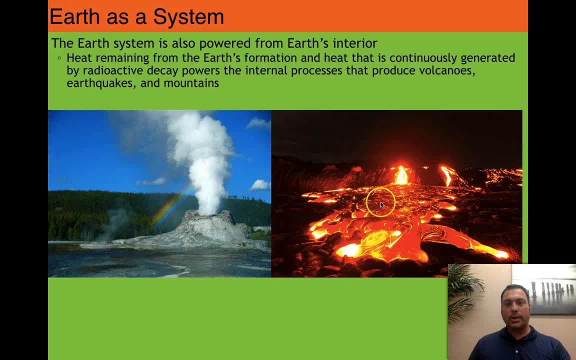 Things heat up, right? Here we see a lava flow. This is coming out of one of the principal vents right near Pu'u O'o on the Big Island of Hawaii. 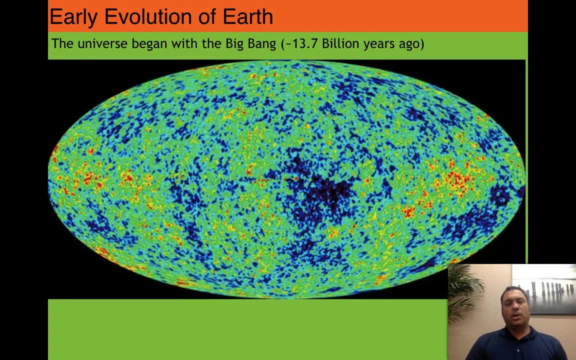 So where'd all this come from? Our current understanding is that everything, all matter, all energy, and the forces that control all of these interactions began with the Big Bang. 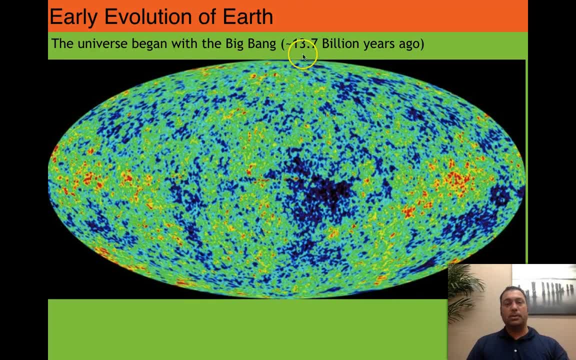 And the Big Bang is believed to have occurred 13.7 billion years ago. The Big Bang, and we've actually gotten a map of it, 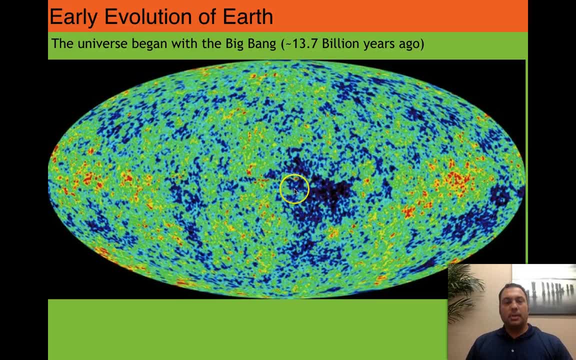 I mean science has gone so far with this, and I'm not going to really go into details of how they got this, but this is the Big Bang a couple hundred thousand years after it happened. 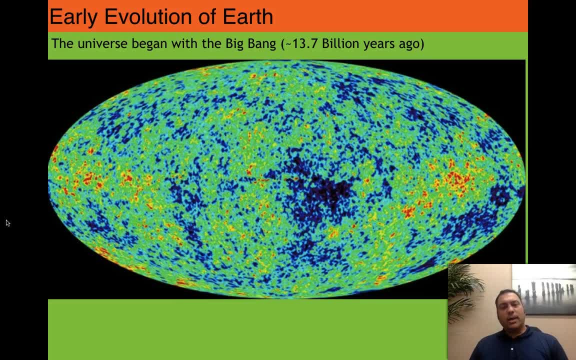 And you might be saying, how did they get that? So you can actually figure it out. There's several web links that you can do. And some great videos that explain it. 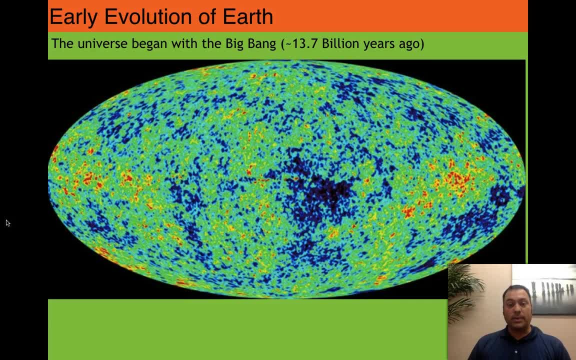 But it's basically background cosmic radiation, or radio waves actually, not as opposed to cosmic rays, but background radio waves that were emitted and pulled and extended as the universe expanded. 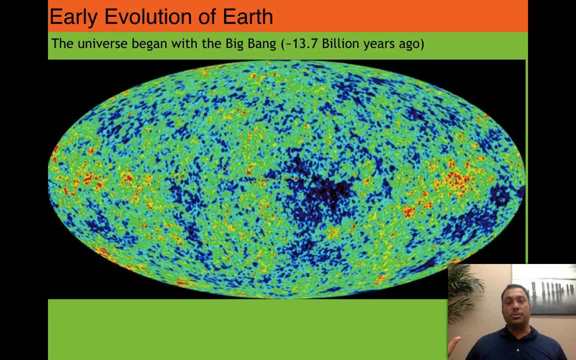 And we're able to actually use satellites to go out and map the distribution of the Big Bang. And this is what they came back with. 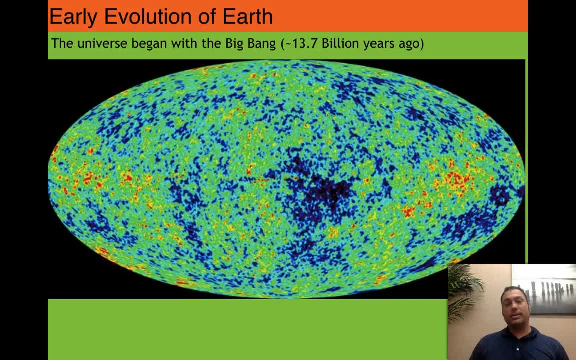 Now how they know that that's part of the Big Bang, again, that's a whole other science class. 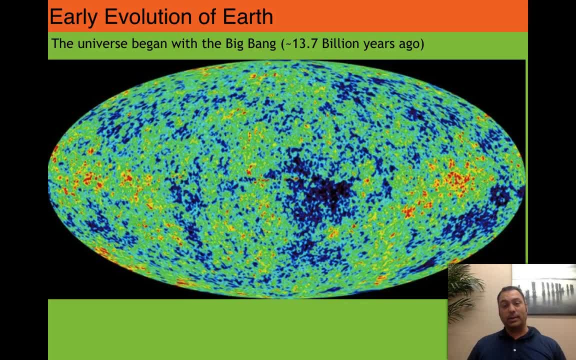 But nonetheless, they do have a really good understanding of what it looked like. And so at 400,000 years after the Big Bang occurred, they can get this picture. Before that, they can't get a picture. This is kind of locked into the universe. 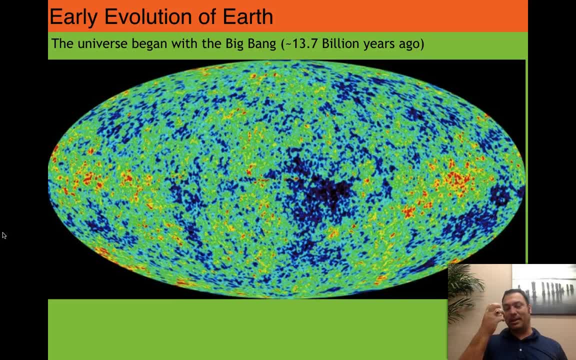 It's almost like a flash going off in your eyes. And you see kind of the memory of the flash in your eye, even though it fades over time. That's kind of what's happening here. 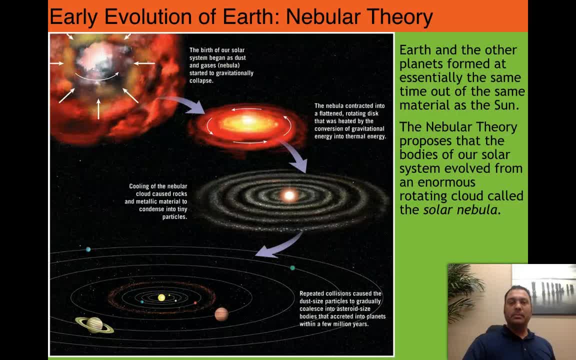 This is kind of the early cosmic flash right after the Big Bang. So the Earth and the other planets formed at essentially the same time and out of the same material as the sun. So you have the birth of our star. You have a bunch of gases and rocks that are floating in space. 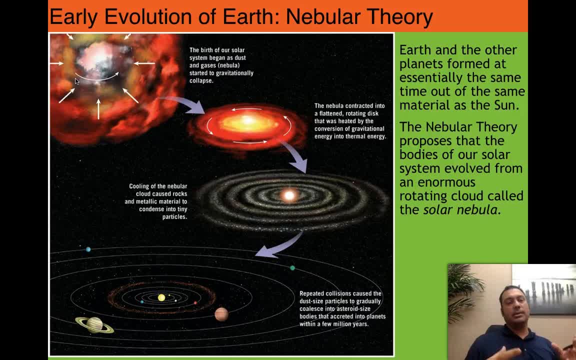 And we call these clumps of gas and rocks nebula. And one of the inherent properties of matter 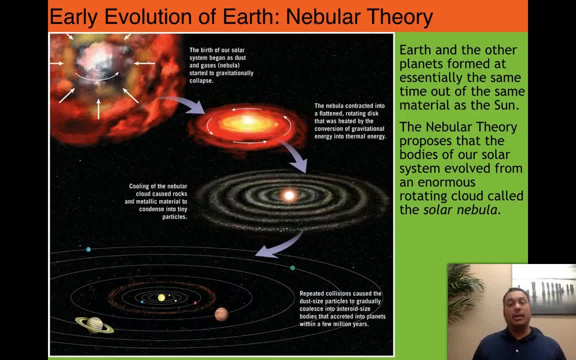 is that matter attracts matter. When we walk on the Earth, there's the force of gravity. The reason why the force of gravity works is because we are matter. We have mass. The Earth has mass. And for reasons that actually nobody knows and nobody's ever been able to understand, even though we call it gravity, we don't really know what it is. 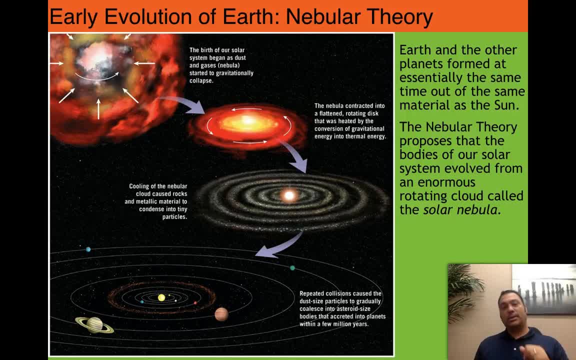 And the fact that you have mass and the fact that the Earth has mass means that you're drawn together. 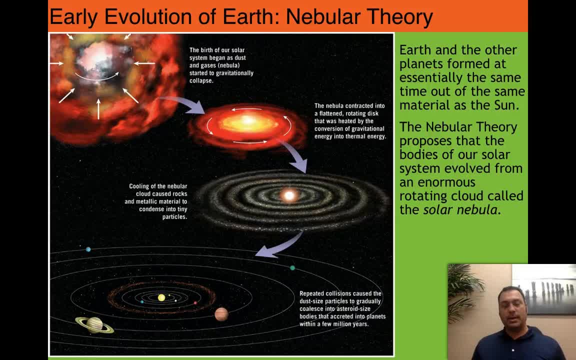 But that occurs with everything. So you're attracted to everything that has mass. And if you happen to have enough mass around you, everybody's attracted to everybody else. Everybody. Everything is attracted to everything else. 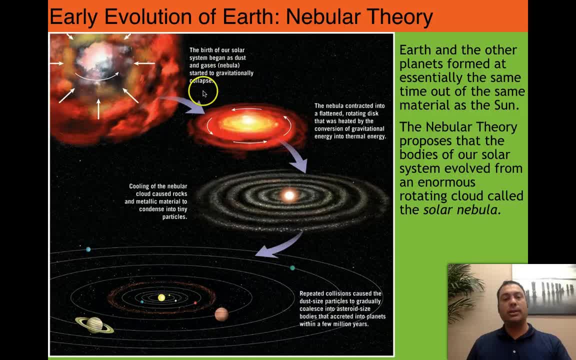 And so what'll happen is it'll eventually start to contract or gravitationally collapse. 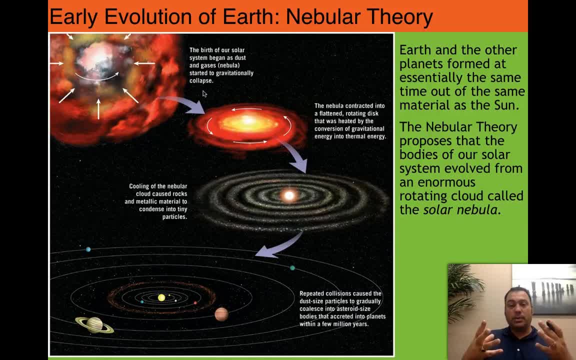 So you have so much material all close together, it all starts to pull in. 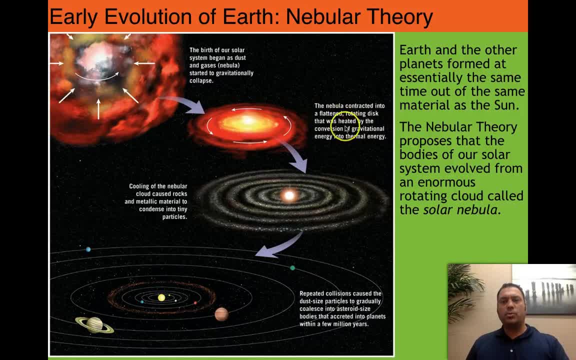 Now the nebula will contract into a flattened rotating disk and it'll heat up. It'll actually heat up because of a transference of energy types from gravitational energy into thermal energy. 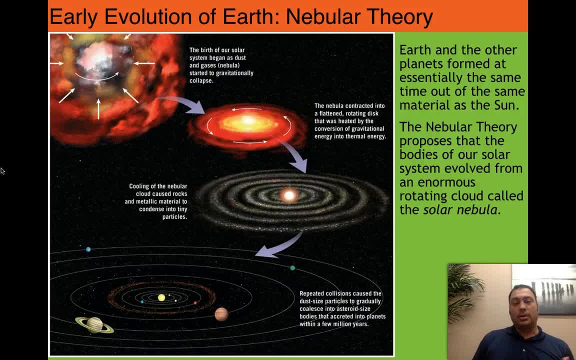 That is a law of physics called the conservation of energy. There's a lot of gravitational potential energy. 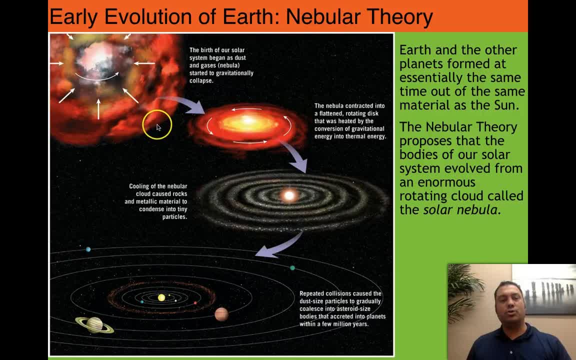 It's like jumping on, you know, this rock right here has dropped into the nebula further. 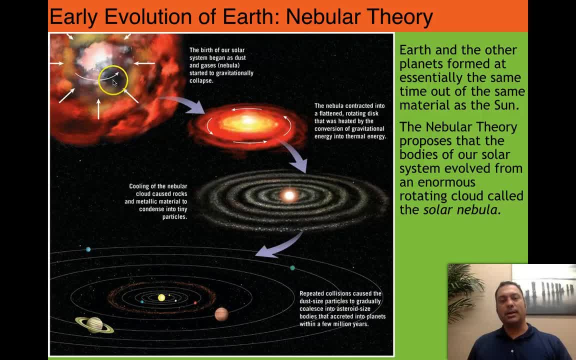 And so energy is released when that happens. It's converted from potential into kinetic energy. Kinetic energy is the energy of motion. And it causes things to heat up. That's really the point of all that. So if you didn't understand what I'm saying, just put it in your back pocket. 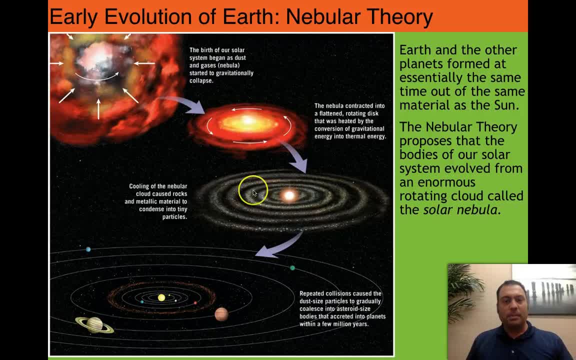 When things get smaller, they heat up. Okay? And they start to spin. Right? 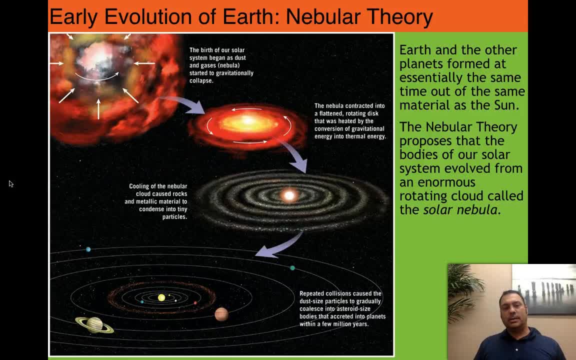 Anybody that's ever kind of seen things contract, let's say you're on a tire wheel and you're playing around and as you spin around and you pull your arms in, things spin faster and faster and faster. Okay? And things get a little stressful sometimes. 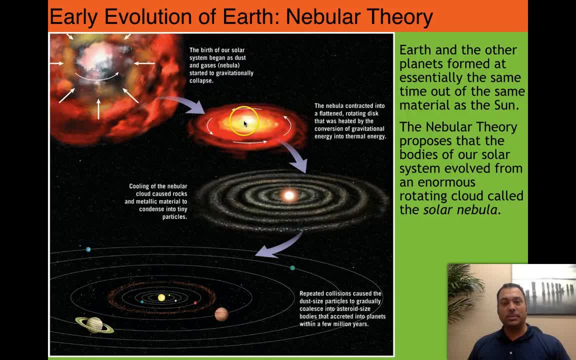 Well, that's kind of what's happening here in the formation of solar systems. So these disks occur and then you wind up with these kind of rings 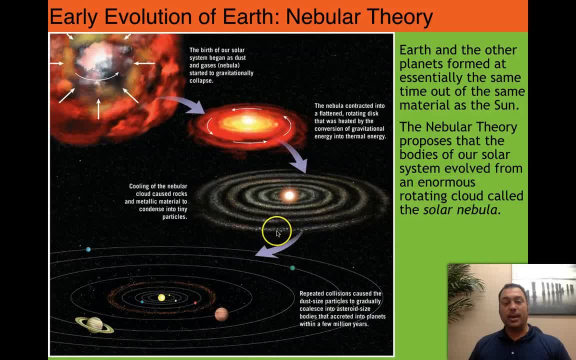 that are traveling at different velocities because the things out here can't go as fast as the things close to the forming star. 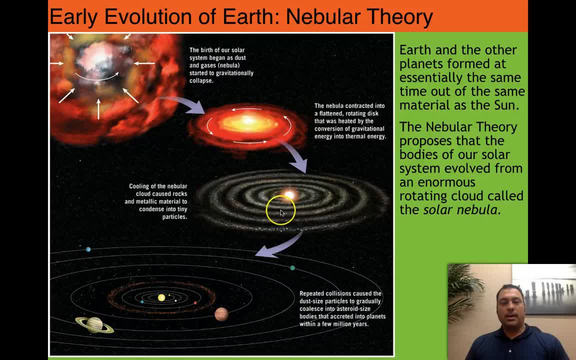 This would be the early proto-sun. And over time, these rings will gravitationally collapse into planets. 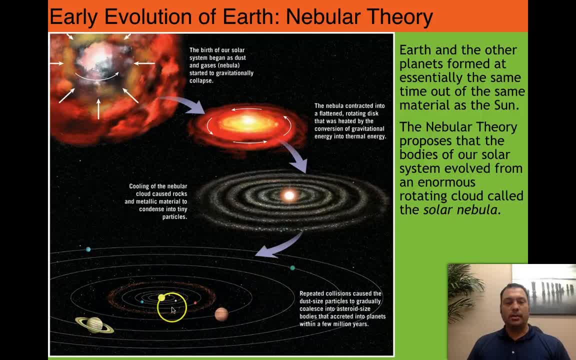 Here we see Saturn, Jupiter, and the inner planets, Mercury, Venus, Earth, and Mars. So the nebula theory proposes that the bodies of our solar system evolved 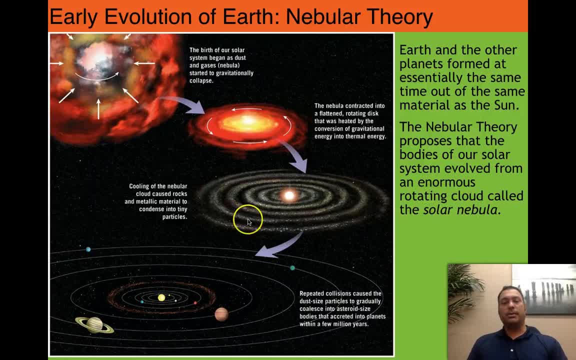 from an enormous rotating cloud called the solar nebula. Right? 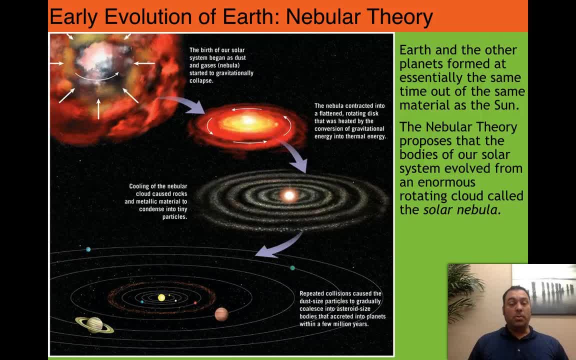 And so it turns out Mars is just as old as the Earth. The Moon is almost as old as the Earth. Neptune, Venus, Jupiter, even the Sun. And when we look at meteorites, we find that they're actually the same age as the Earth as well. 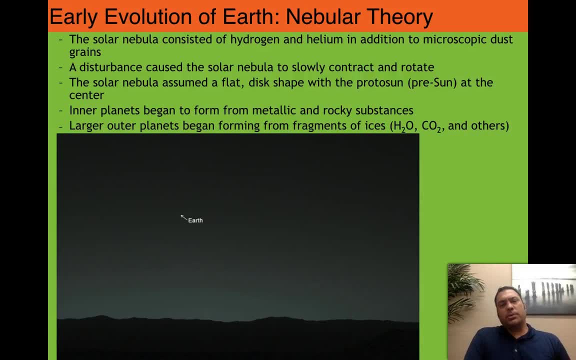 So what was the solar nebula? What is the theory here then? Well, the solar nebula consisted of hydrogen and helium 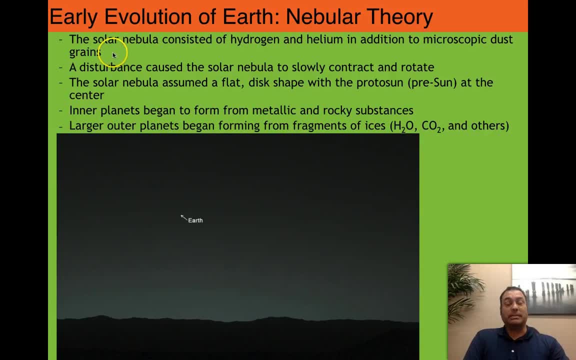 in addition to microscopic dust grains, you know, things that we would recognize right away as being little bits of dirt. Right? 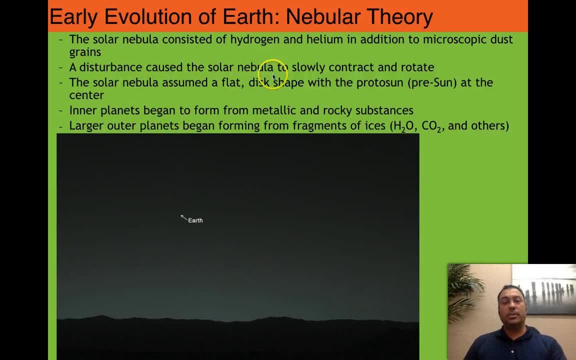 A disturbance caused the solar nebula to slowly contract and rotate. We don't know what that disturbance is. We do know that the Sun had at one time a sister Sun that formed at about the same time. But it's actually quite far away from us now. And maybe it was the interaction of those two stars that brought about the formation. But who knows? Right? Science hasn't answered that question yet. 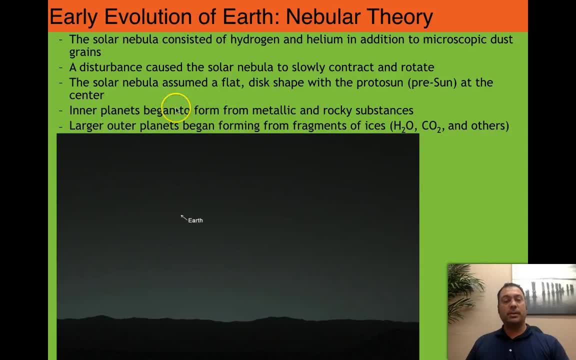 The solar nebula assumed a flat disk shape with a proto-sun at the center. The inner planets began to form from metallic and rocky substances. Large outer planets began forming from the fragments of ices. So it turns out that in the inner part of the solar system 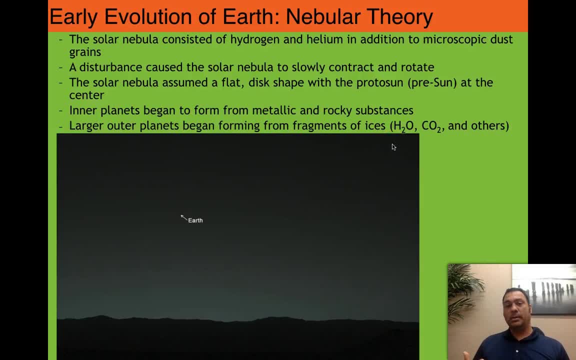 we find lots of rocky planets. Not unlike Earth in some ways. Mars is much smaller than Earth, but it has rocks and volcanoes and all of that stuff. 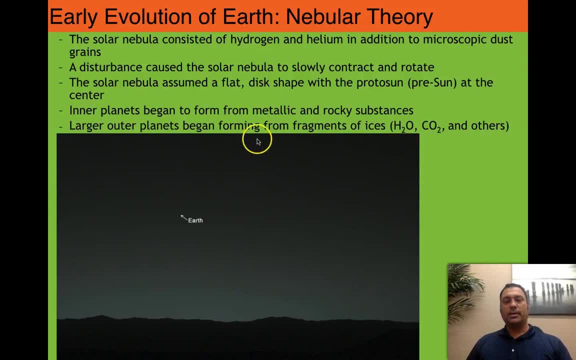 But when we go further out we don't see that so much. Instead we find that the moons that are surrounding Uranus and Neptune and Jupiter have large amounts of water and carbon dioxide and methane and things like that. 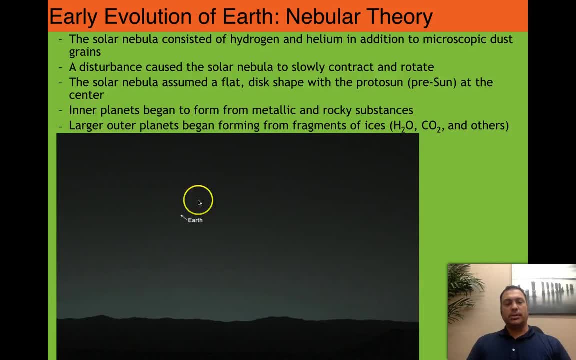 You might be wondering what this image is down here. You notice it says Earth. This is a real picture taken from a satellite that had landed on Mars pointed up towards Earth. And so if you can look right there to the middle it might look like a little piece of dust on your screen. 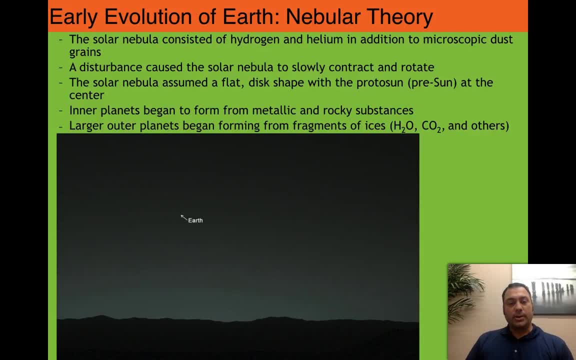 If you have it in high resolution you should see it. Or high definition. 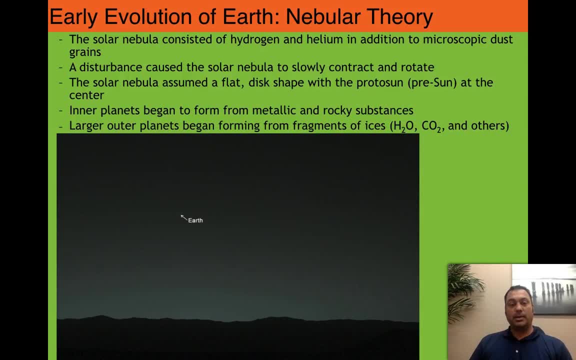 That's the Earth as seen from Mars. And if you look really, really carefully and I'm looking kind of carefully right now you may even convince yourself you see the moon, but I've never heard that it's visible. But anyway, but the Earth is. And it's really just a little light speck up in the sky from Mars' perspective. 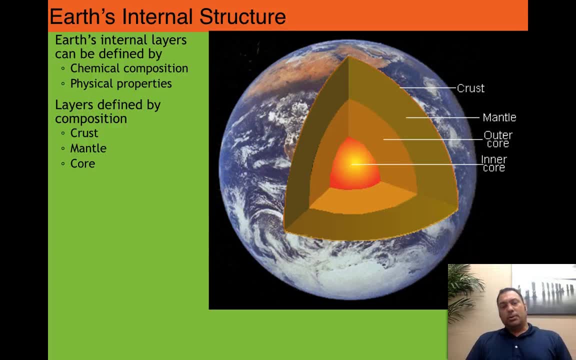 There's some structure to the Earth also, right? It's just not a blue ball with water and land on it, right? There's some structure to it. 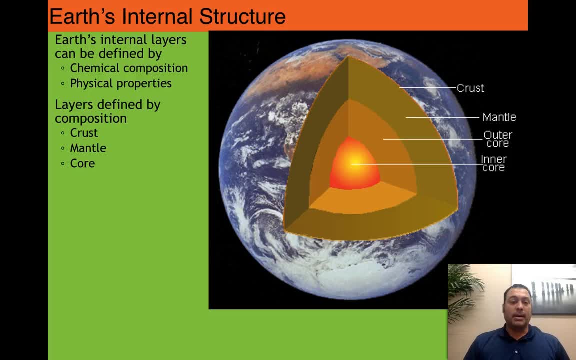 And this internal structure is something we're going to spend the next couple of weeks really hitting hard. It's important to understand that what happens on the inside is what's determining what's going on on the outside. The sun plays a role. But it's a minimal role compared to the internal heat of the Earth. 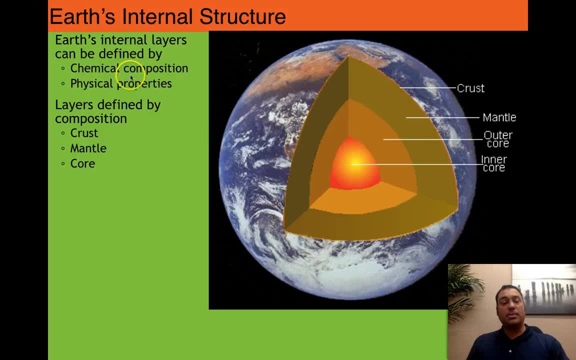 So the Earth's internal structure can be defined by the chemical composition. 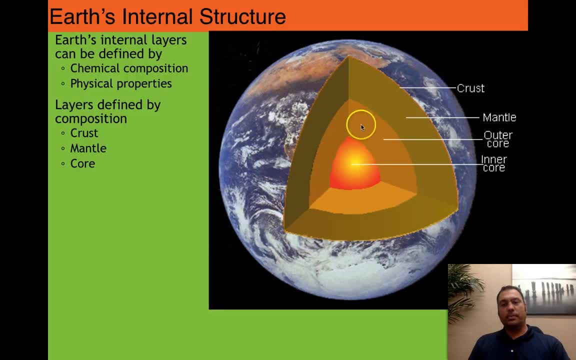 So here we have three layers, or actually four layers. There's an inner core, there's an outer core. So the core of the Earth, which is the centermost part. Here's the mantle, which is the part that's in between us and the core. 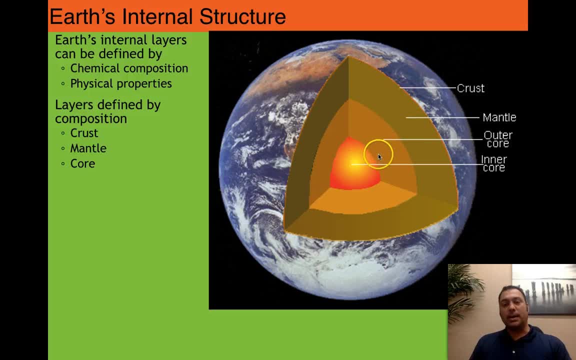 And it's made out of rocky material. Actually, the core is actually metallic. 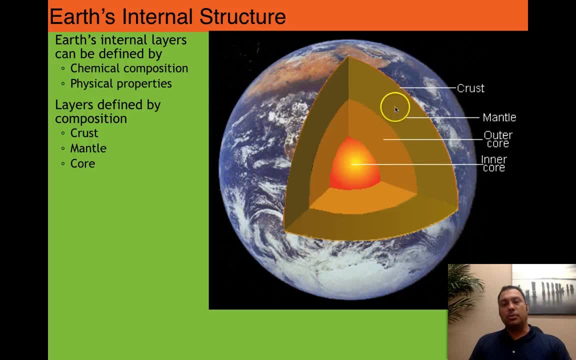 It's made out of iron, mostly. But the mantle is mostly rocky. And then, of course, we get up to the crust, and that's definitely rocky. 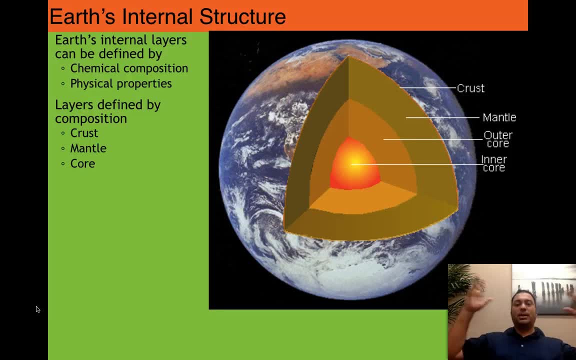 We know it because we live on it, right? We don't find metal sheets coming out of the volcanoes that are active today. 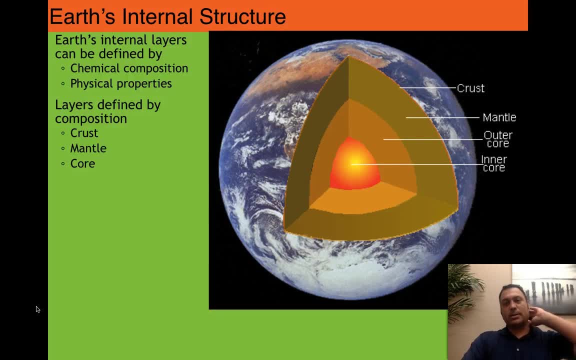 We find rock, basalt that is being spewed everywhere on the seafloor and on volcanoes. 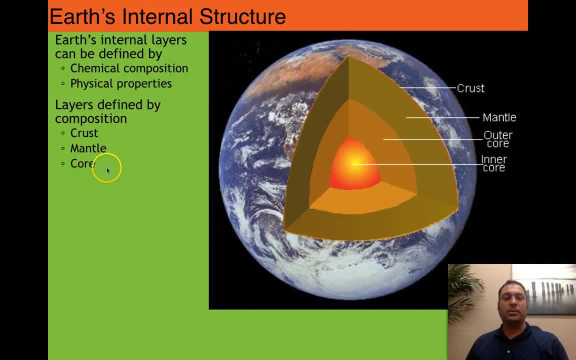 So the layers are defined by their composition, the crust and the mantle and the core. How did this come about? Why do we have a layered Earth? 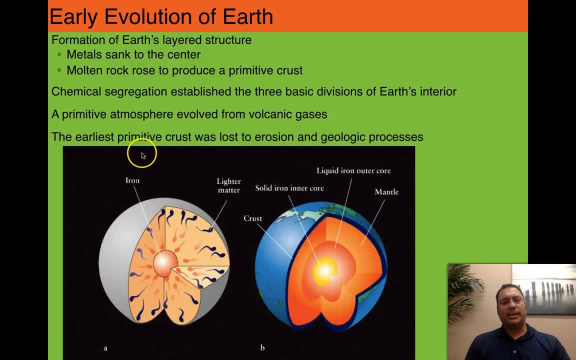 Well, it turns out that it's really just something called density that's driving everything. 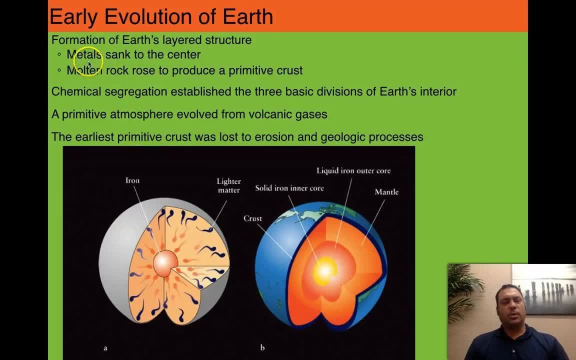 So basically, the layered structure occurred when metals sank to the center. Right? So here you have the Earth. The metals, all the iron and all the magnesium, and even some oxygen in some cases, are going to sink down to the bottom. 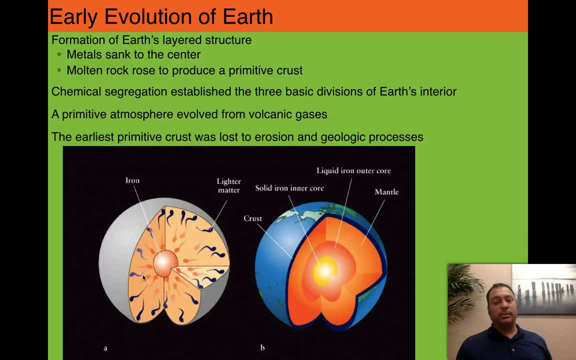 Because why? It's heavier, or what we would say denser. And if it's more dense, that means gravity has a stronger pull on it 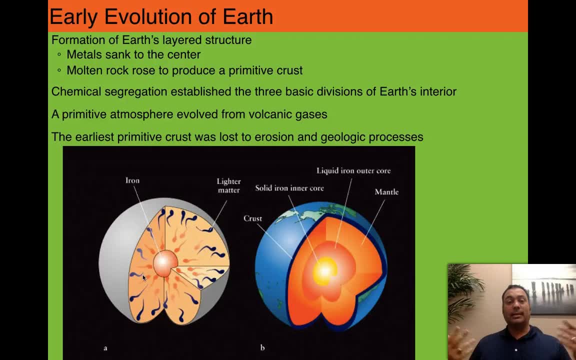 and it's able to pull it down more readily than it can the lighter things. 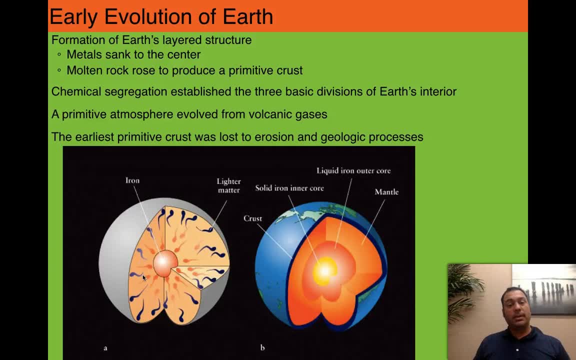 So greater gravitational force pulling the heavy things towards the center. Things that are still heavy, but not as heavy as that, wind up floating out to the edges. 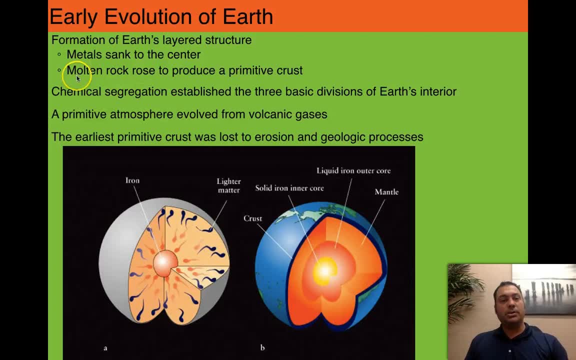 I should say molten rock rose to produce a primitive crust. So here we have our primitive crust right here in the image. 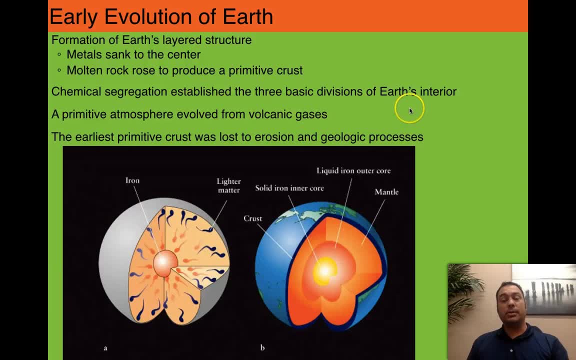 Chemical segregation established the three basic divisions of our center. We talked about that. The core, the mantle, and the crust. 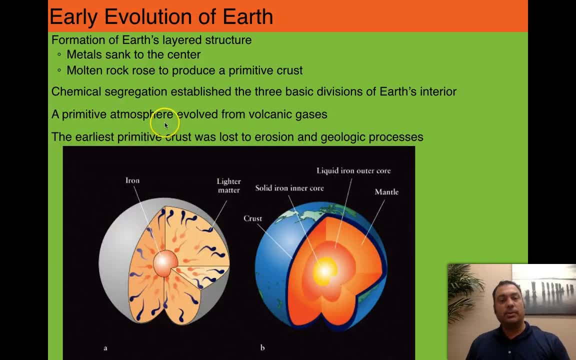 But it also produced a primitive atmosphere. From volcanic gases. And it's actually still making our atmosphere today is still being evolved by volcanoes. 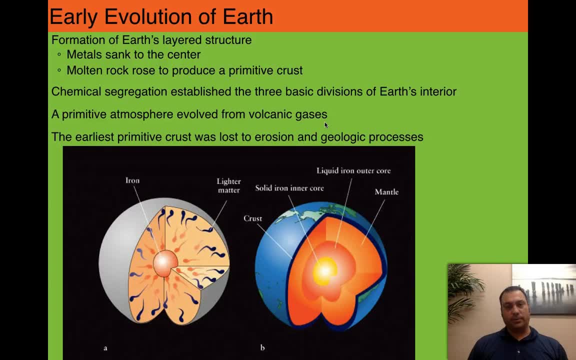 Largely the chemistry is controlled now by biological effects through interaction between animals and plants and the sea and some other complicated processes. 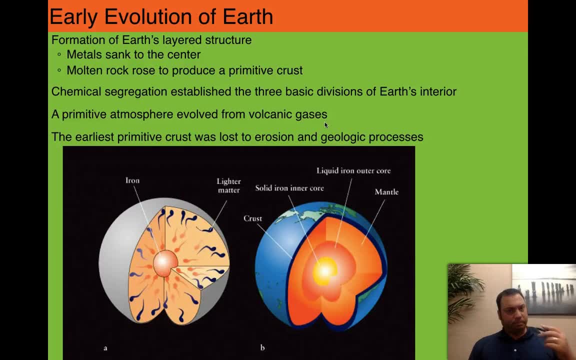 That is more of an environmental science question. But you get the idea. 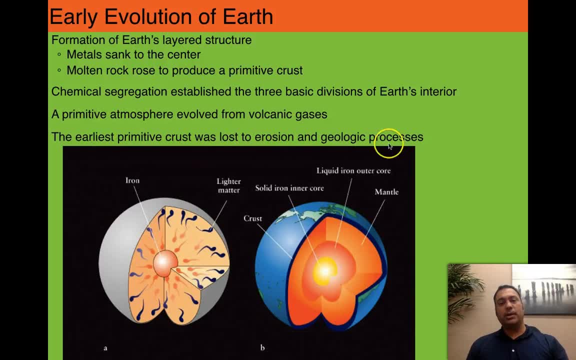 And the earliest primitive crust was lost to erosion and geologic processes. So there was so much turmoil occurring early on while this was occurring where the iron was going down to the bottom or sinking towards the core. 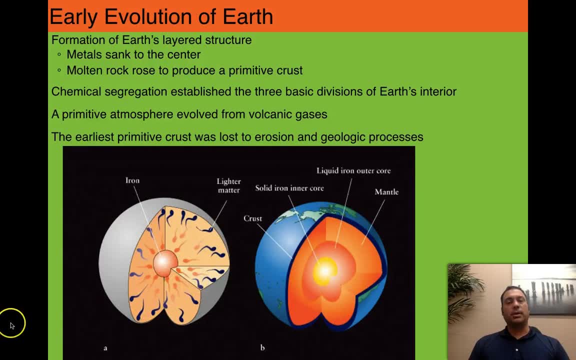 And the lighter rocky material was floating near the surface and making an early crust. But that early crust has been lost to us. 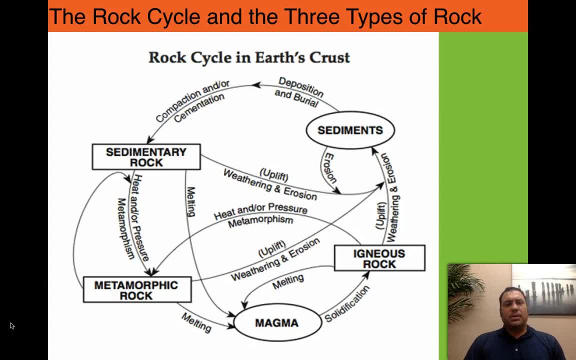 And of course how has it been lost to us? Well, something called the rock cycle. It turns out that things on Earth are constantly cycling around. Nothing is really the same forever. The oldest rocks that we have on the planet date to about three and a half billion years old. 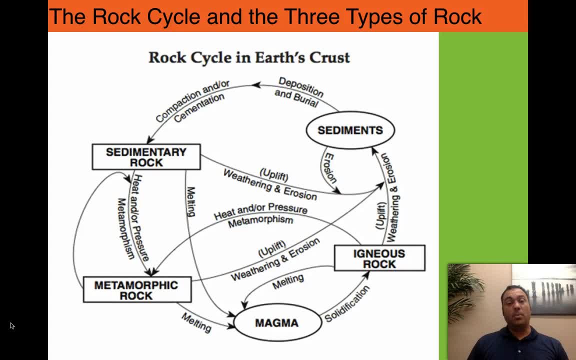 We do find minerals that are even older, almost as old as the Earth itself, about 4.3 to 4.4 billion, depends on who you ask, years old. 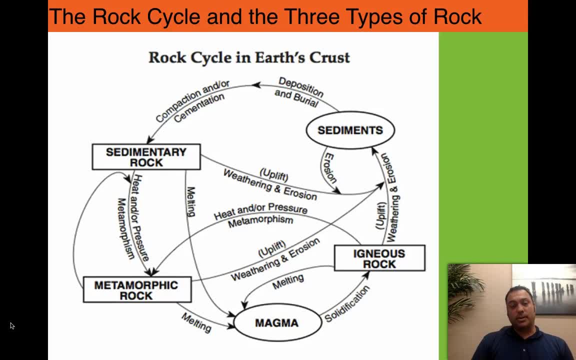 That's right after the Earth formed. And we find those actually in Australia. 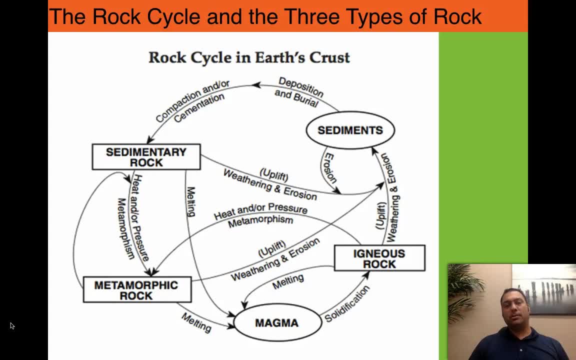 But those minerals were recycled out of a previous rock and now we find them in a new rock. And that's because Earth is constantly cycling minerals and rocks and stuff around. 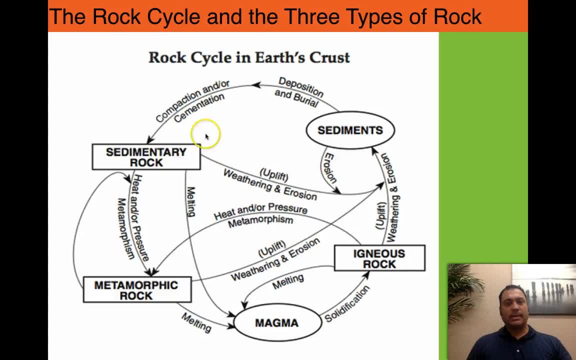 The material is always changing. And that is called the rock cycle. 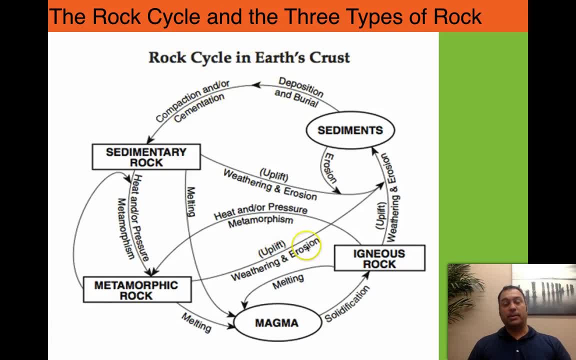 There are three different kinds of rocks on planet Earth. There's igneous rock, there's sedimentary rock, there's metamorphic rock. Igneous rock is rock that is brought from, you know, literally means, igneous means fire-born or fire-breathed rock. It means it's actually from a molten magma. 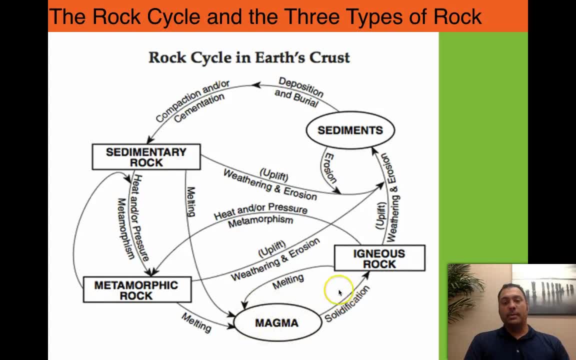 It's from a melted rock source, a liquid. And it solidifies. And over time, it might get eroded or attacked by weather patterns. And that causes it to break up into small pieces and maybe the igneous rock eventually becomes a sedimentary rock, which is like a sandstone or a shale or silt or dirt, you know, dust. And if you take those sediments and you bury them long enough and you add water, you wind up getting a sedimentary rock, right? So you get loose sediment that becomes sedimentary rock, an actual rock that you can pick up or you can polish up or whatever. And put into a rock collection. 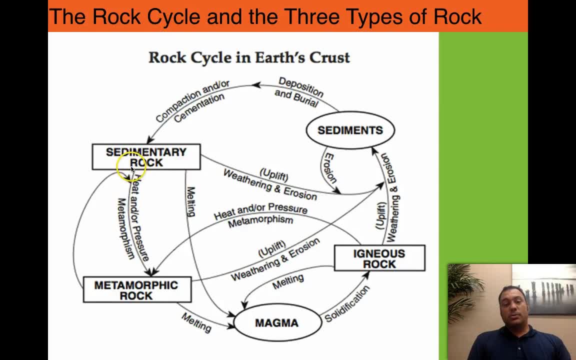 Sedimentary rock can also be altered into igneous rock because I can melt it, right? I can heat it back up or actually it would be this path. I can melt it and it would go into the magma chamber and I can make igneous rock out of it again. 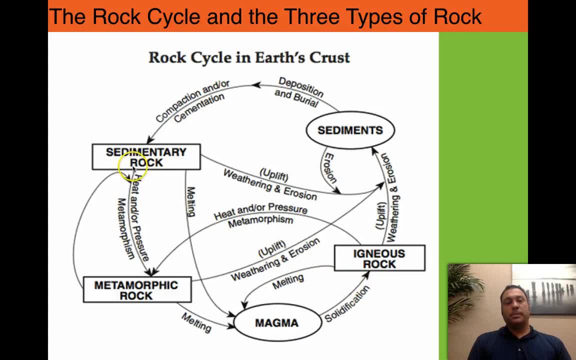 Or I could continue to put it under heat and pressure, you know, right? So not just compaction and cementation, 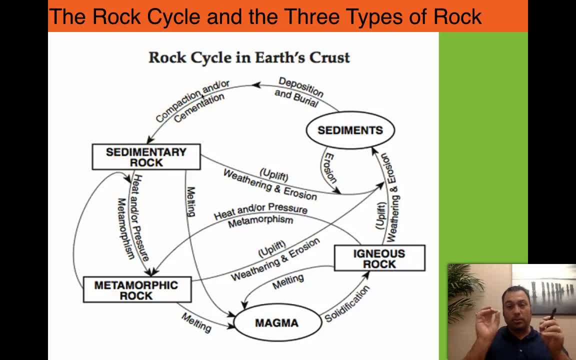 which is the process of lithifying or making a rock out of little particles of rock. 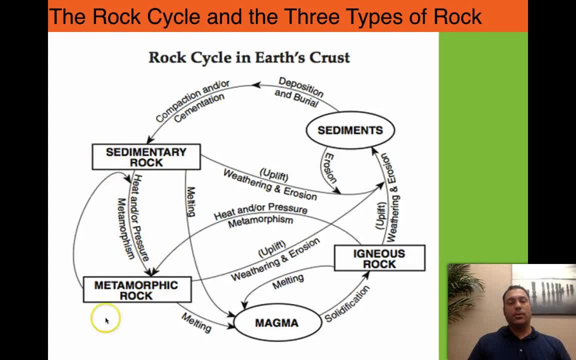 I can then take sedimentary rock and turn it into a metamorphic rock. Meta meaning changing face or changing shape rock. So a metamorphic rock is one that is not quite melted but it's at such high heat and high pressure that the sedimentary rock gets altered into this. So it actually is kind of a hybrid in some ways, or not really a hybrid. It's kind of a mid-level stage between a sedimentary rock, which usually forms at the surface of the earth, and igneous rocks, which form under conditions which actually melt the rock. 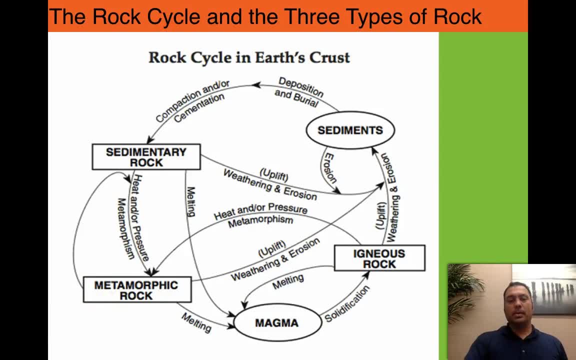 And metamorphic rocks exist in the middle of those two. And they cycle around, right? 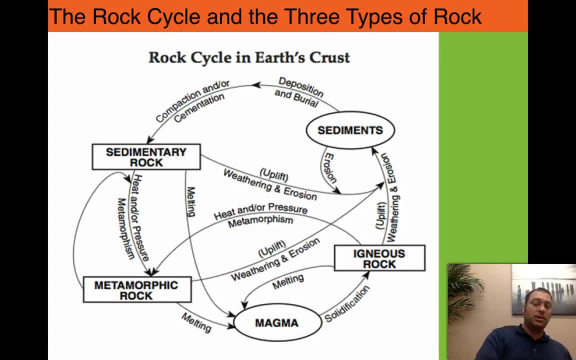 A metamorphic rock can be melted. An igneous rock can be put under heat and pressure and made into a metamorphic rock. Anyways, you get the idea. 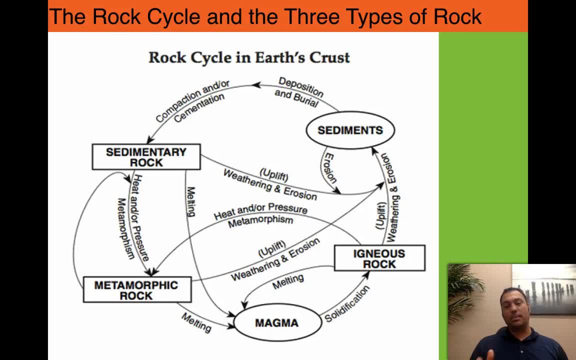 We're going to be talking about each type of rock in detail as we go through the class. It's the primary focus of the first series of lectures, actually. 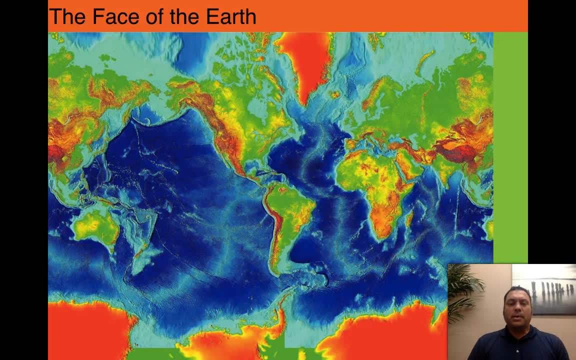 So we've been talking a lot about the earth, about the rock cycle, about how things are constantly changing and turning over. 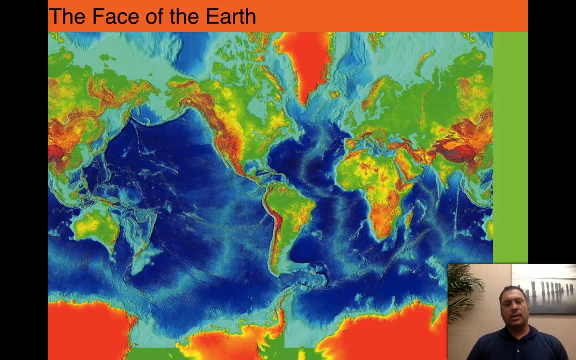 We need to kind of understand what the face of the earth is. What does the earth look like? There's several features that pop out. 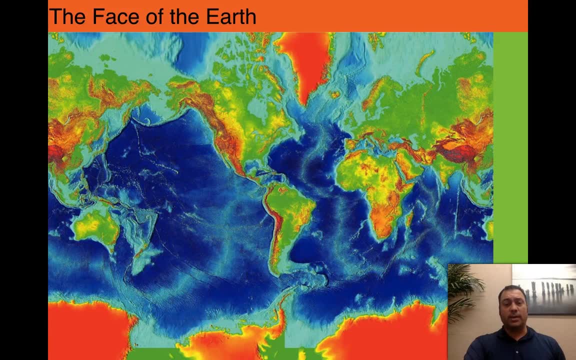 This, of course, is what they call a physiographic map of the earth. And basically the color tells us how high something is. So something that is red is actually quite high. It's a mountain. 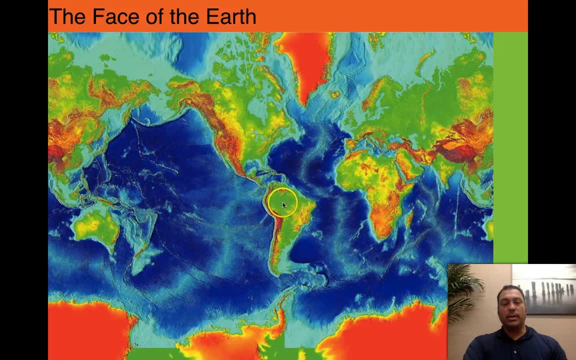 Something that is yellow or green is quite low, right? Usually the green is actually the lowest. Blue is the oceans, but the light blue is shallow ocean, whereas the dark blue is the deep ocean. 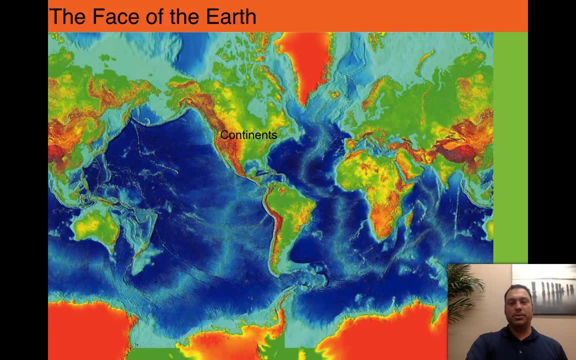 And we notice pretty rapidly there's a couple of interesting things that happen. First off, we notice that we have continents, right? We have deep ocean basins here, and we have continents. The continents are these areas with large mountain chains. 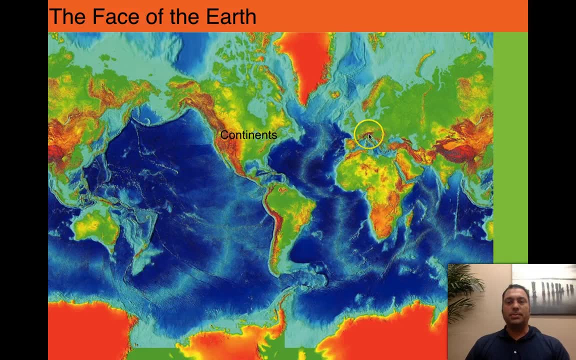 These are the Himalayan Mountains. Here are the Alps. The Alps are very small by comparison with the Himalayas. 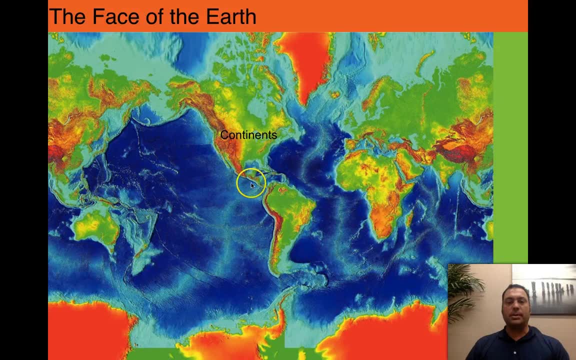 And, of course, the Appalachian Mountains and the Rocky Mountains that extend all the way from Mexico into Alaska. The Andes Mountains here. 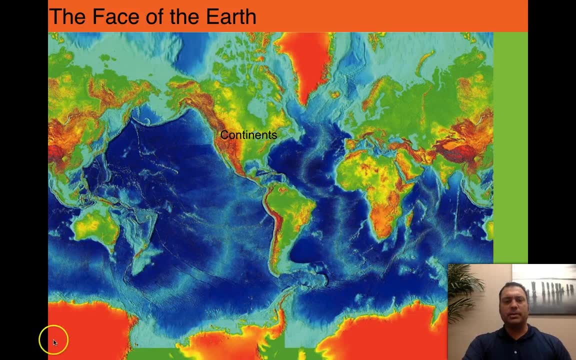 Now you might notice, well, there's a lot of research that says the Himalayas are red down here, but it doesn't look like mountains. 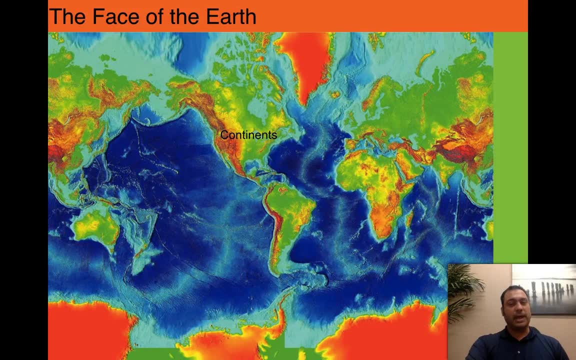 We'll get into what that is differently. It does turn out that it is very high. 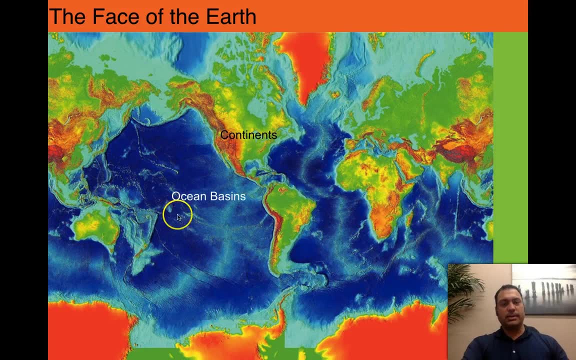 It has a very high elevation, but it's also very flat. Here are the ocean basins, right? The ocean basins are these deep sections of the earth that are covered largely by water. 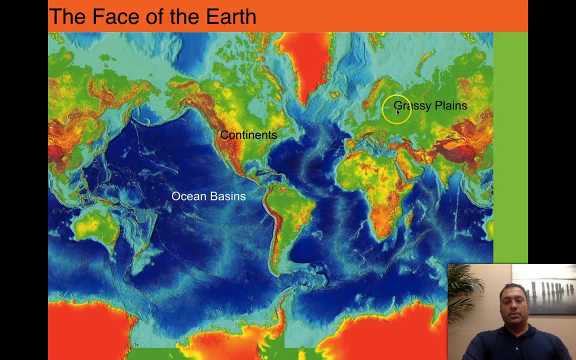 In almost all cases, it's covered by water. These green areas here are usually the grassy plains, or actually tropical rainforests. 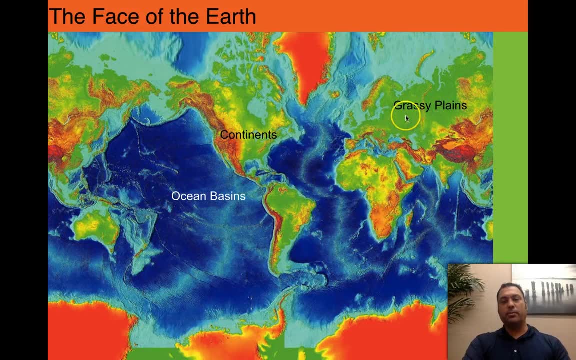 So here we see the Amazon rainforest here is in green. These are the grassy plains. These are the plains of western Russia. Our Great Plains of the United States and Canada extend all through here. And you get the idea. 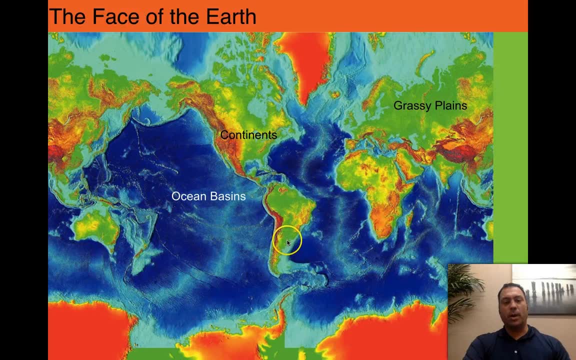 Here's basically a really good growing country for wine and things like this in South America. 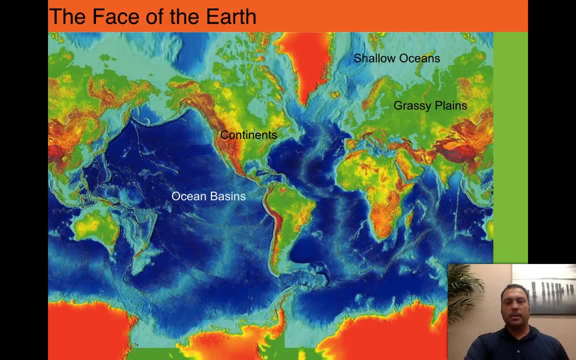 And we have plains over here in Australia as well. 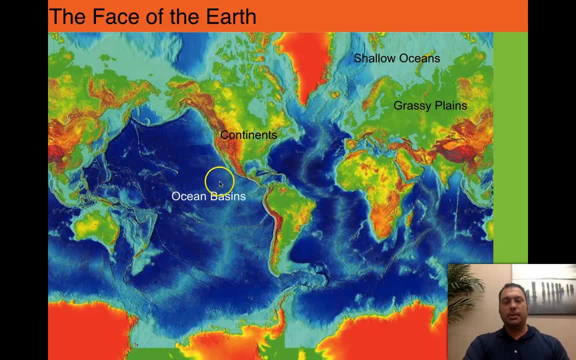 We also have shallow oceans, right? Not everything is a deep ocean basin like we see over here. Sometimes we get shallow oceans. And those are mainly concentrated not just up here in the top part of the map, but they're also located here off the coast of Alaska, located in Hudson Bay, and even along the coast, eastern coast of the United States, southern coast of South America. 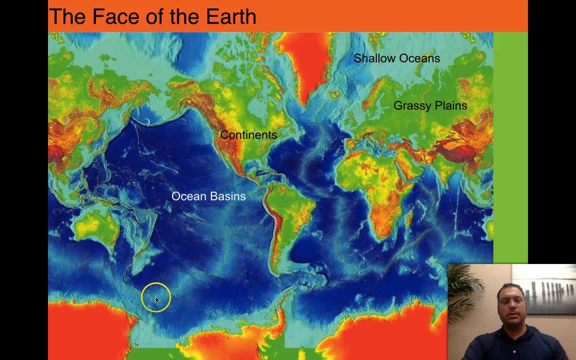 But we also find something else, that there's these blue areas in the middle of the ocean. 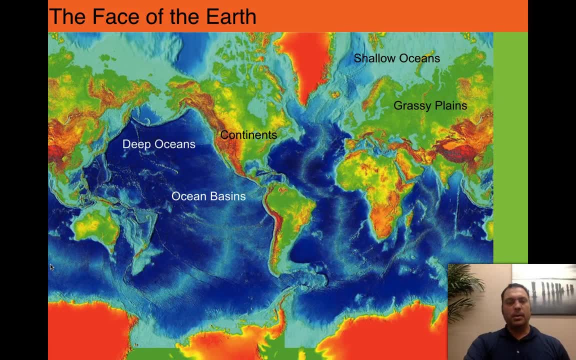 What is that? We'll come to those here in a moment. 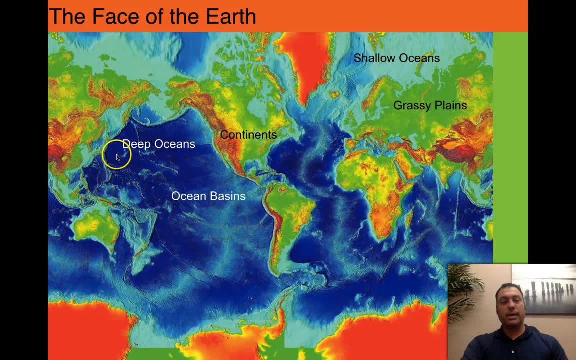 Here we see the deep oceans here, these deep parts. We'll notice that the Pacific Ocean has the deepest part actually located way over here near, this is Japan, right near Japan relative to the eastern part where it's actually fairly shallow. 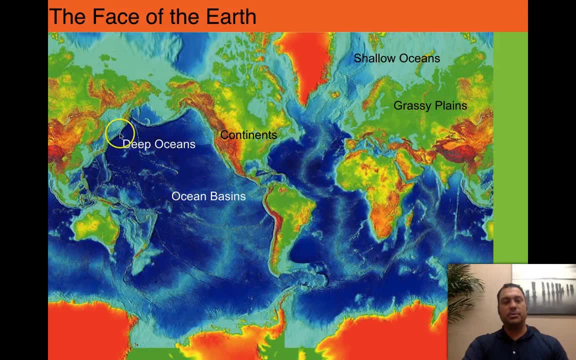 You would think that the deepest part of the ocean is right in the middle, but it's not. 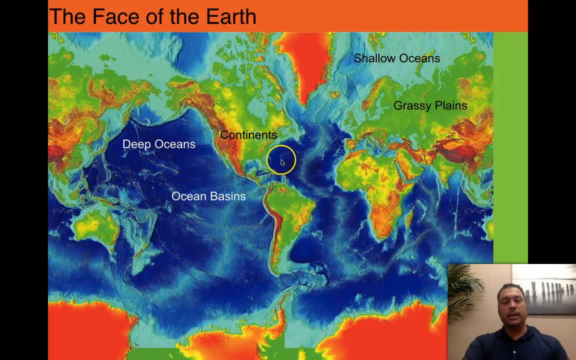 It turns out it's actually near the edge. The deepest part of the Atlantic is here and here, and the same thing with the Indian Ocean, the deepest part is here. 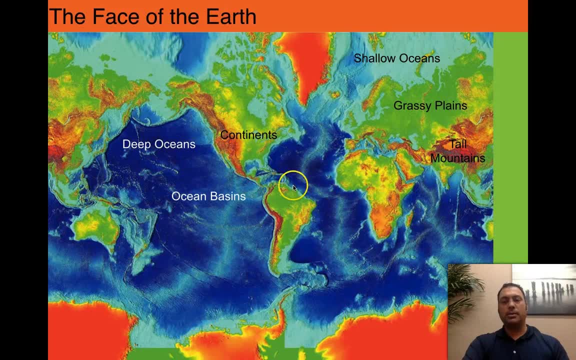 We also have tall mountains, right? Notice the tall mountains. I actually went through those in detail. 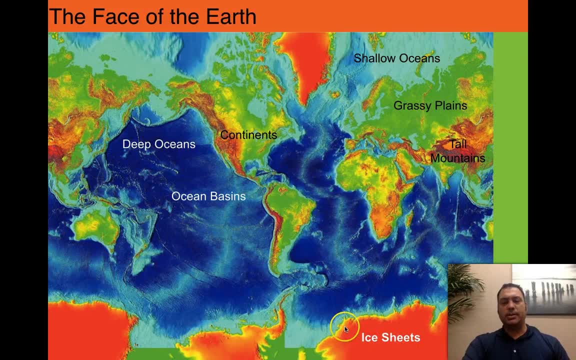 But what about these things? These turned out to be ice sheets. 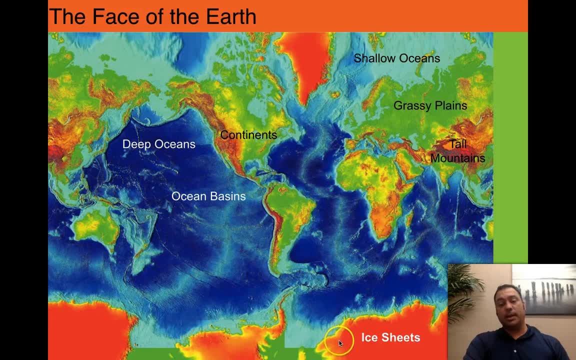 These are ice sheets that are several kilometers thick. Think of a kilometer. A kilometer is, there's 1.6 kilometers in a mile. So these are ice sheets. 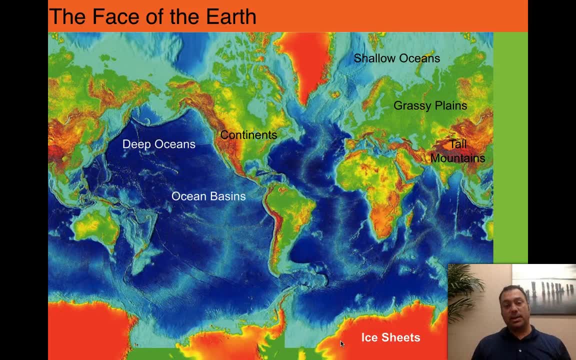 These are big, thick layers of ice that are in some cases miles thick or kilometers thick. 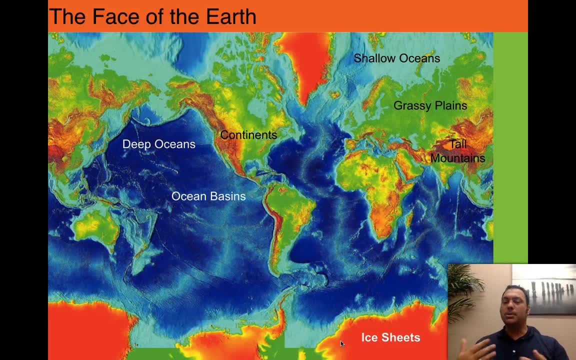 I'm going to use the metric system in this class, so be accustomed to hearing kilometers and if you need to, get out a calculator and learn how to convert between the two. 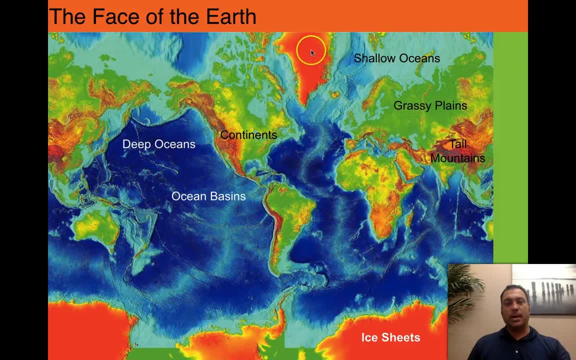 But we also notice that here's Greenland, and Greenland is nice and high, but it's all smooth, right? 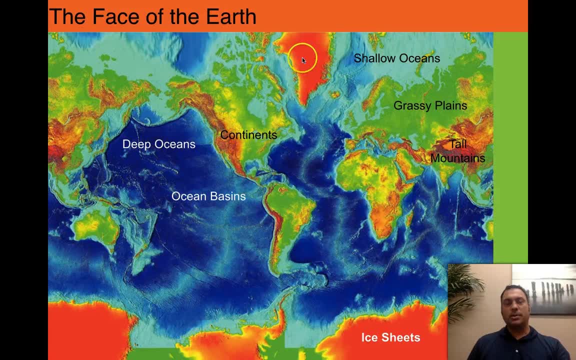 Unlike what we see over here in the Himalayas and the Rockies. It's all smooth. It's all covered with ice, too. 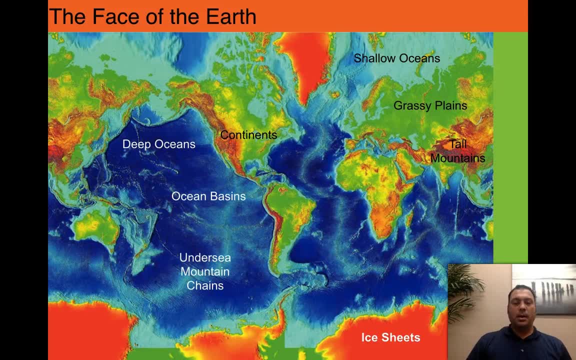 This is Antarctica, by the way, down here. It turns out that this shallow blue area is an undersea mountain chain. 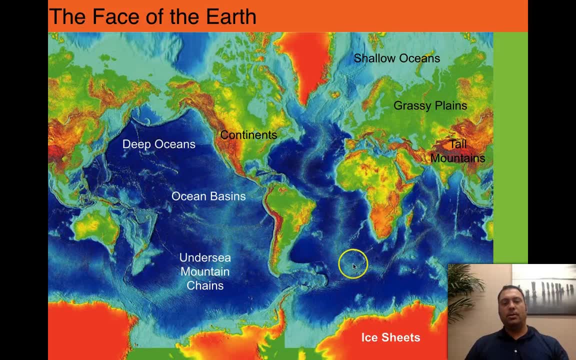 So there's large undersea mountain chains, a zipper all over the planet. 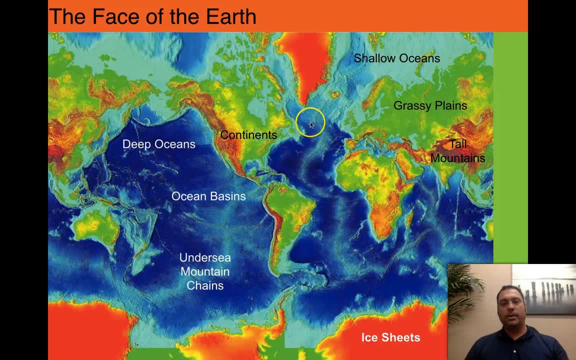 Here is the longest and tallest of them all, right here, the Mid-Atlantic Ridge, which is a large undersea mountain chain. 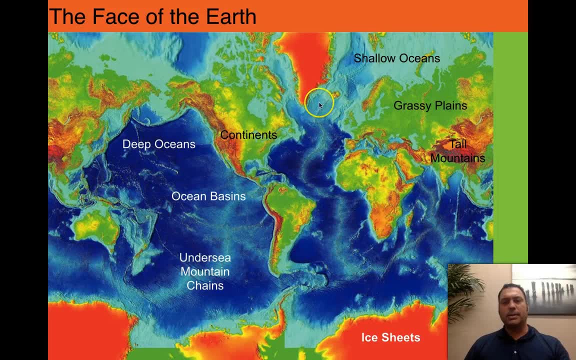 And the top part of it is Iceland. Iceland is part of this undersea mountain chain that actually pokes up out of the surface of the ocean. 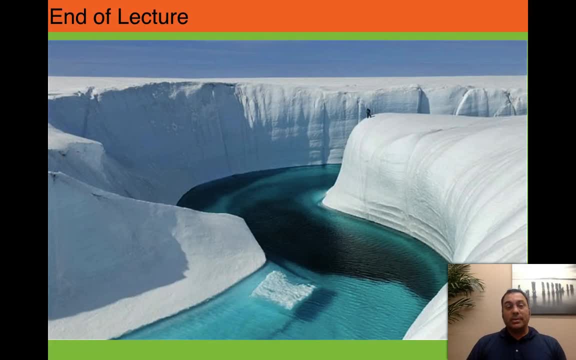 So with that said, I hope you got a decent introduction to what this class is about and what we're going to be looking at. I want you to be interested and get an understanding. 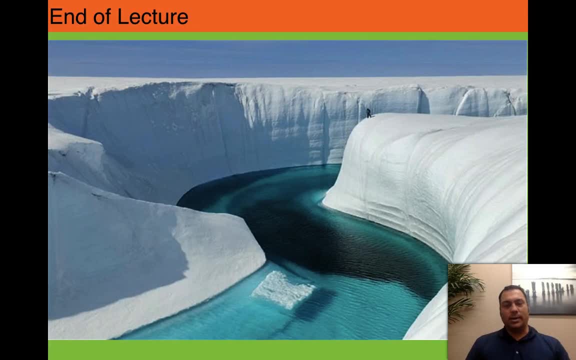 This is an ice geologist that's doing work in Greenland. And in case you can't see him, he's right up over here. 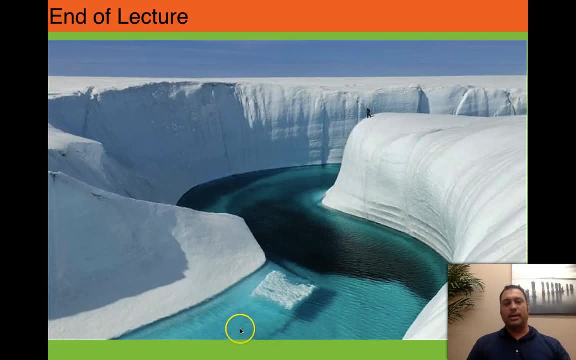 And this beautiful lake. If he was to fall in here, it would be instant death. He would die of icy cold water, hypothermia. You get the idea. 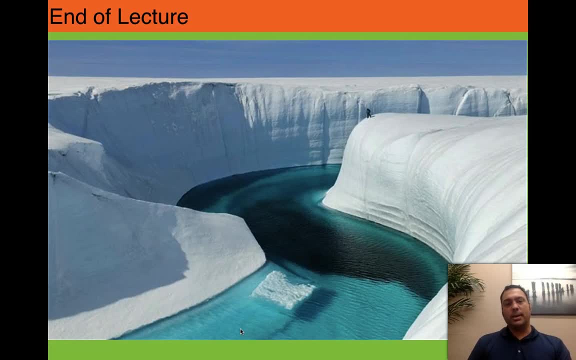 This is a way of life for a lot of people, studying the Arctic and studying ice geology 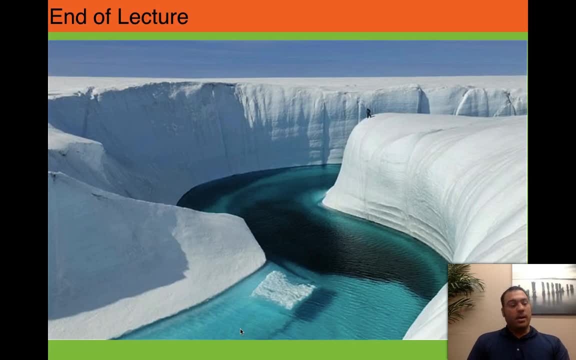 and how these rivers form and what they mean for global warming, 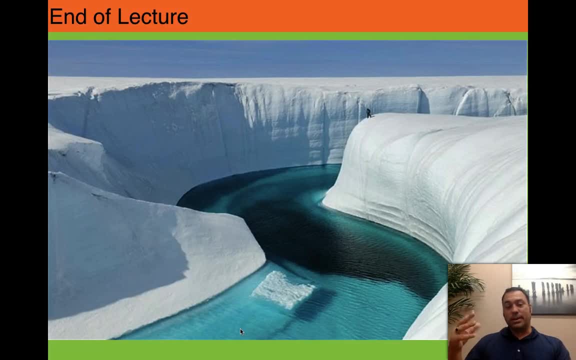 what they might mean for global cooling in some areas, right? Some places heat up. 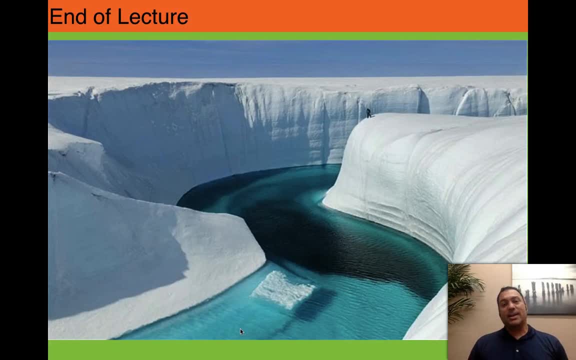 Some places are actually going down. It's complicated. And it takes scientists, those with really good instruments and good will and somebody who has the know-how to be able to solve these problems and to ask the right questions to start solving them. 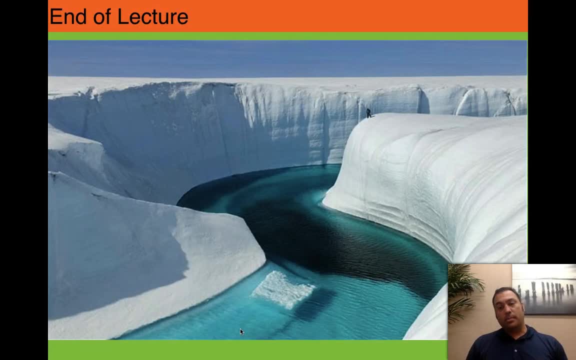 So with that said, this concludes our first lecture. And I hope if you have any questions, feel free to get onto a discussion board 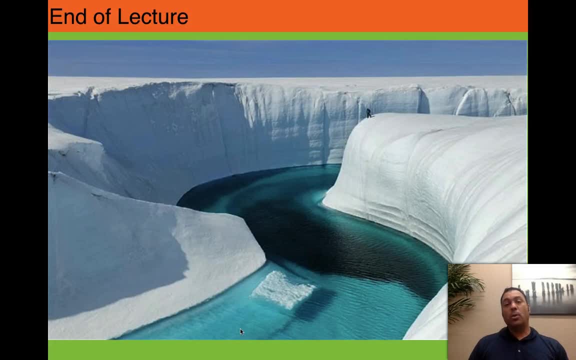 or to send me an email because I'm happy to answer any of your questions that you have. 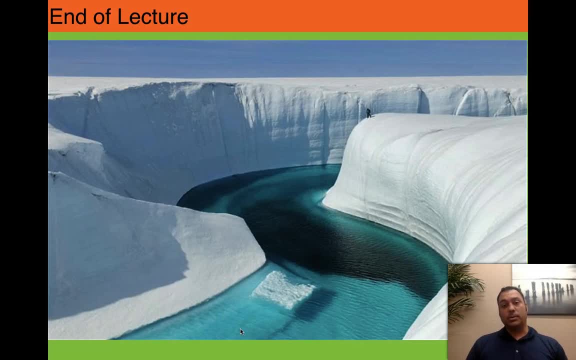 Or you can always ask your classmates on the discussion boards. So until next lecture, have a good one.